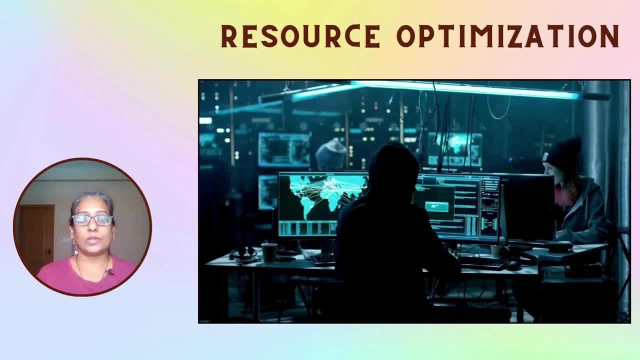 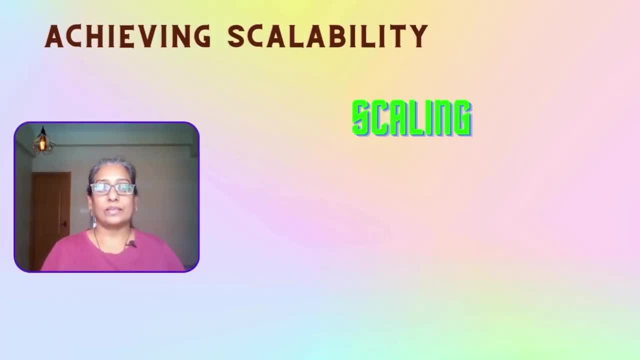 on demand. This optimization reduces operational costs and maximizes the return on investment in infrastructure. Scalability comes in two flavors: Vertical scaling, where you upgrade a single machine, and horizontal scaling, where the load is paid across several machines. Let's discuss a few practical approaches to implement scalability. 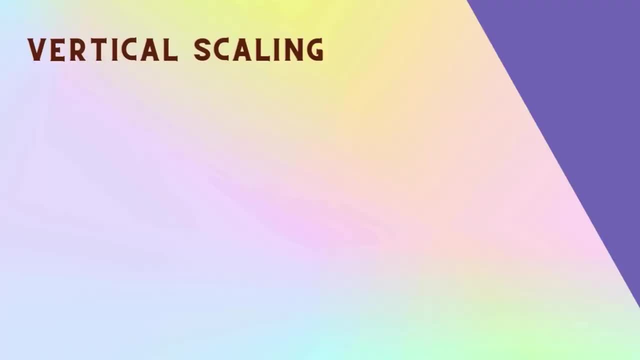 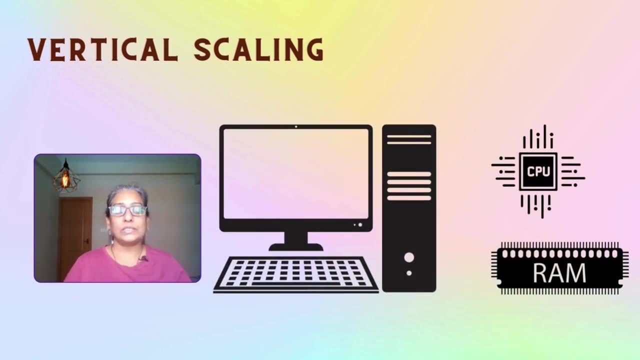 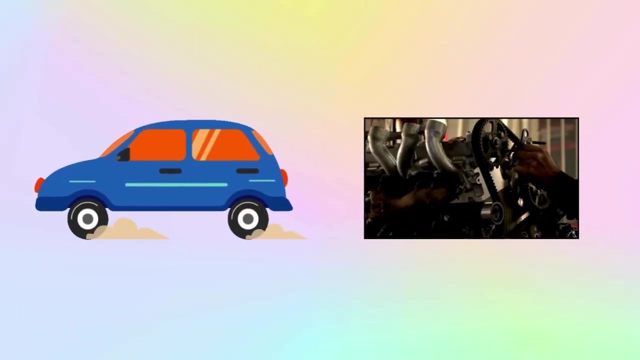 including vertical scaling and horizontal scaling. Vertical scaling is also called scaling up. To achieve vertical scaling, more resources are added to a single machine, like more CPU power or more RAM. Imagine adding more horsepower to your car by upgrading the engine. That's vertical scaling in action. It's simple and effective, but has its limits. 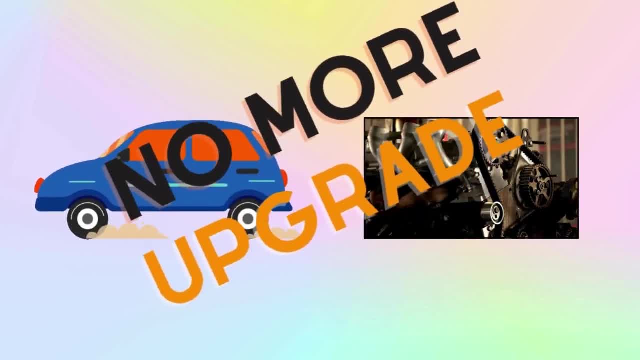 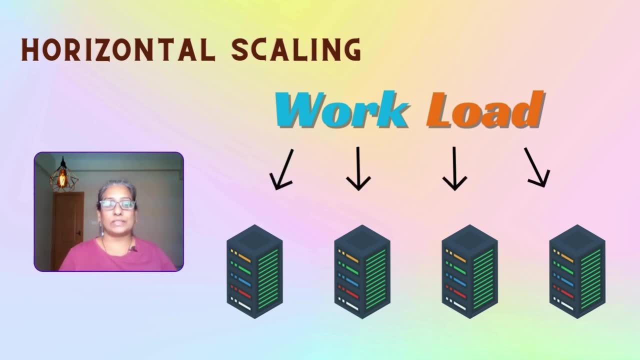 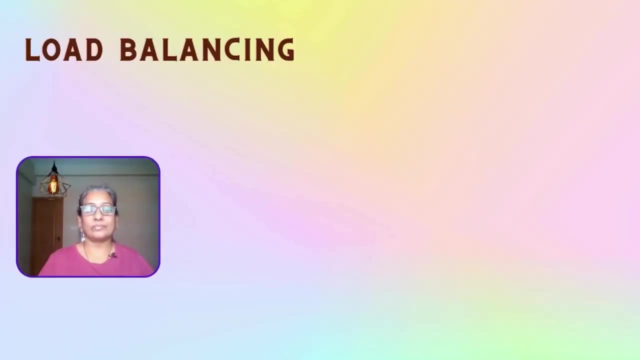 After a certain point, you no longer can upgrade the engine. In horizontal scaling, the load is spread across multiple machines of either same or different capacities. It is like having multiple cars instead of just one for a group trip. Load balancing helps us achieve horizontal scaling. Load balancing distributes incoming requests across multiple servers, ensuring optimal performance and efficient resource usage. It's like having a traffic cop directing cars to the least congested lanes on the highway. Load balancers employ various algorithms, such as round-robin, least connections or IP hash, to distribute traffic effectively. 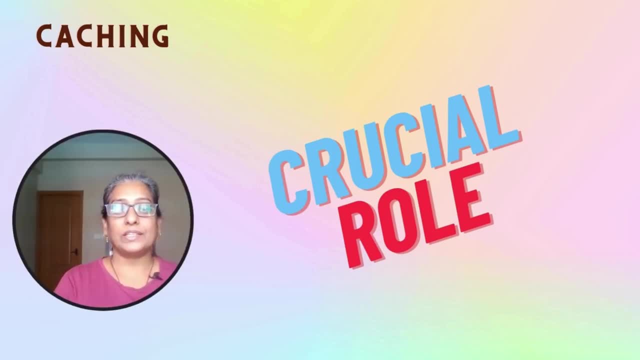 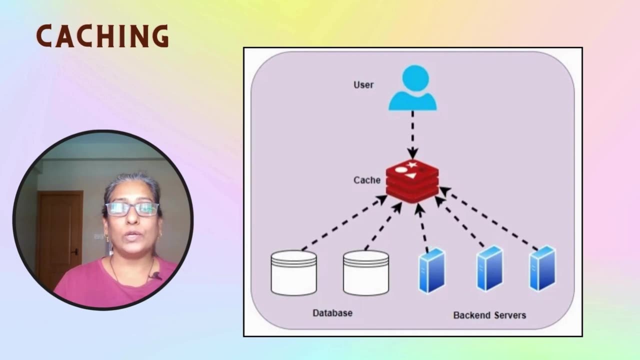 Caching plays a crucial role in scaling a system. Caching involves storing frequently accessed data in high-speed storage such as memory or SSD, to reduce the latency and improve the performance. By caching the data near application or user systems can server requests faster and minimize the load on back-end databases or services. 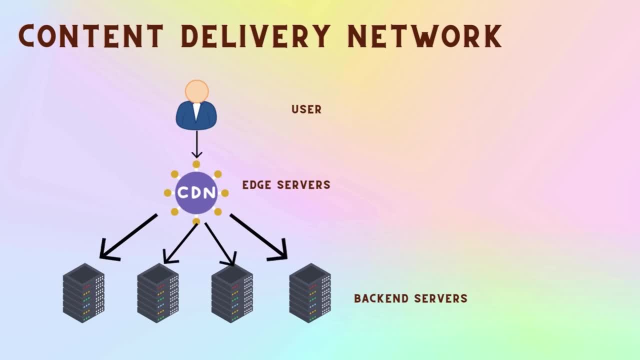 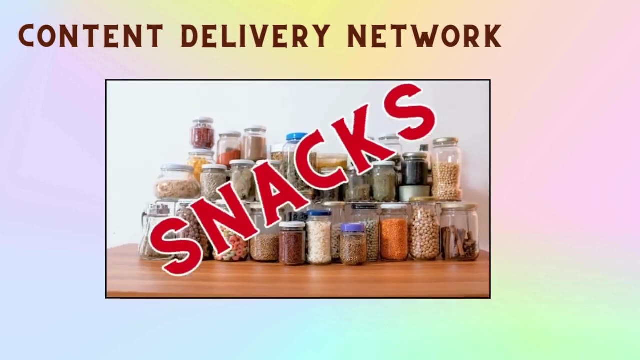 Content delivery networks, or CDNs, exemplify caching on a global scale. CDNs cache static content at edge servers worldwide to deliver content with low latency to users across the globe. Caching is like having a pantry stocked with your favorite snacks: You can grab things quickly without having to run to the store every time. 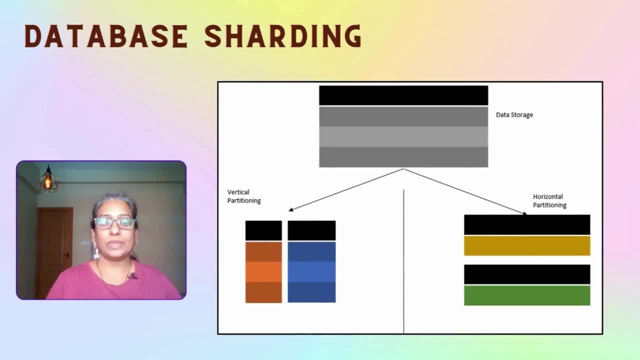 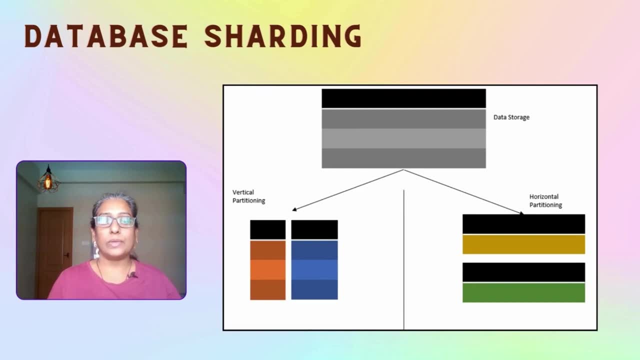 Database sharding is one another way to achieve horizontal scaling. It involves horizontally partitioning the data across multiple database instances or shards, Based on a predefined key or rule. each shard operates independently, allowing the system to distribute the data storage and processing workload efficiently. 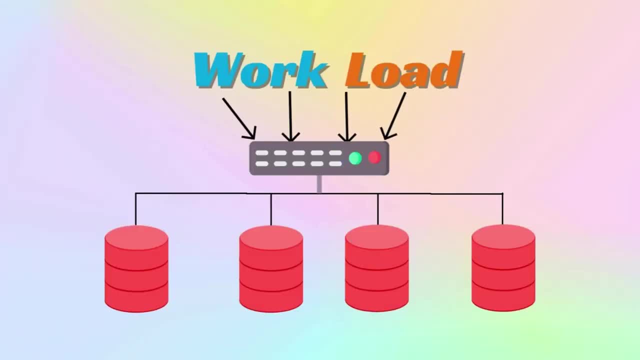 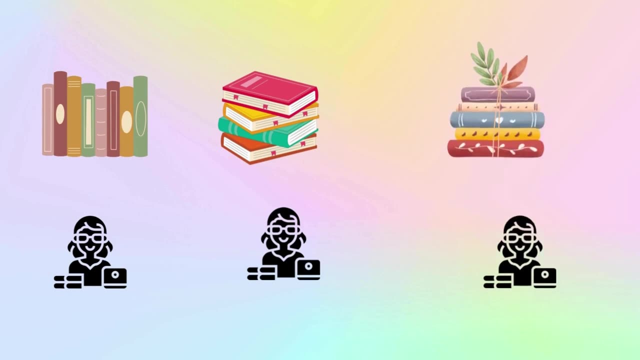 Sharding enhances scalability and performance by enabling systems to handle large data sets and high transaction volumes. Imagine organizing your book collection by genre and distributing them across different bookshelves. Database sharding is like having multiple librarians managing different sections of the library. You can find books faster and up-to-date, more readers. 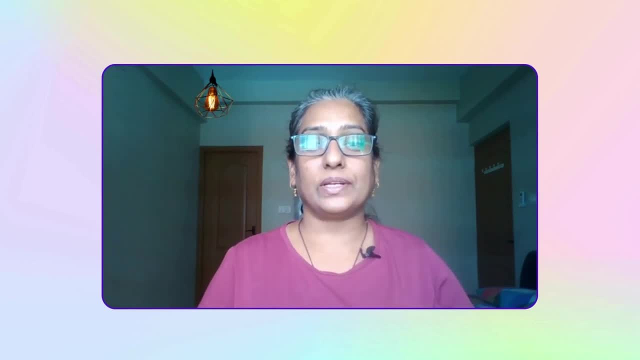 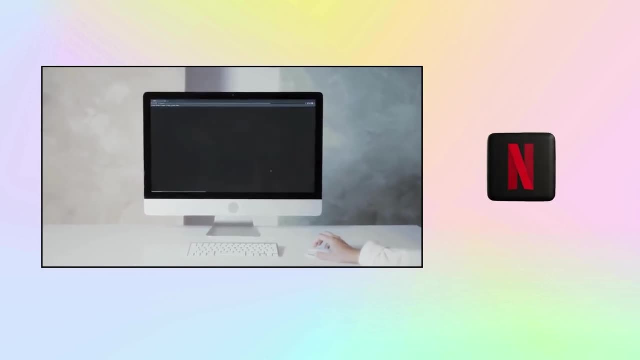 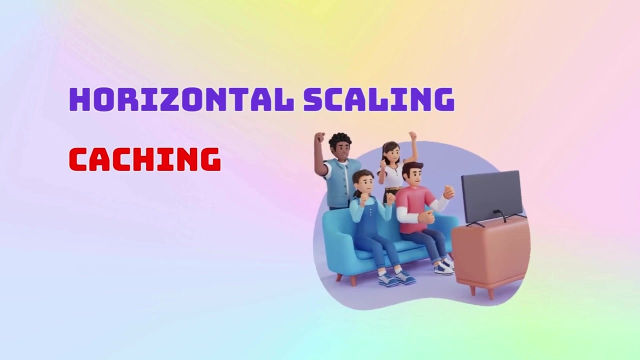 Let's explore real-world applications where scalability is implemented. Think about how smoothly Netflix steams your favorite shows, even during peak hours. That's because they use horizontal scaling and caching to handle millions of viewers without buffering or downtime. Ever wondered how Uber matches riders and drivers in? 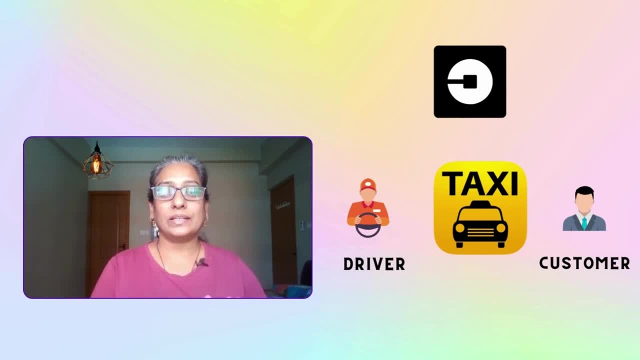 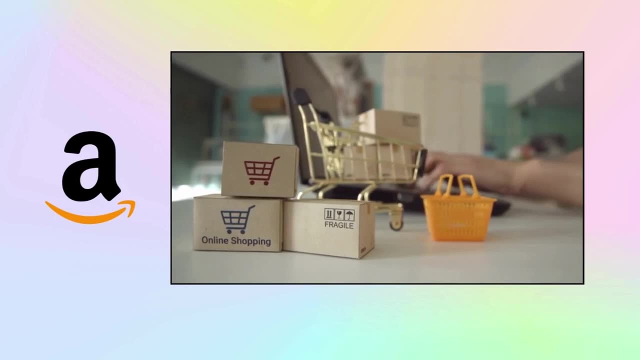 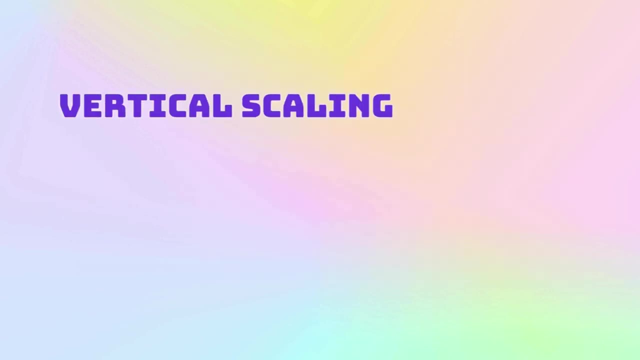 real time, no matter where you are. it's thanks to their use of horizontal scaling and load balancing. consider how amazon manages to process millions of orders seamlessly, especially during the holiday season. they leverage a combination of a vertical and horizontal scaling, load balancing and caching to deliver a stress-free shopping experience to their customers. scalability is the secret sauce. 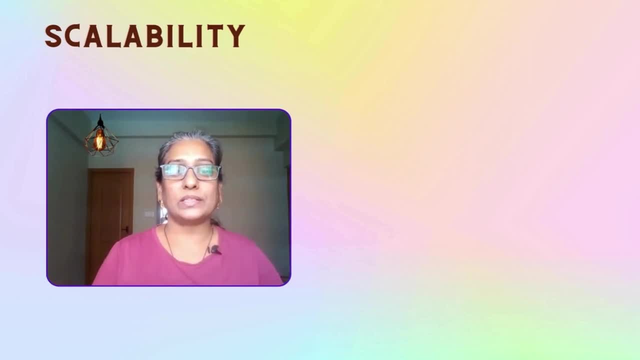 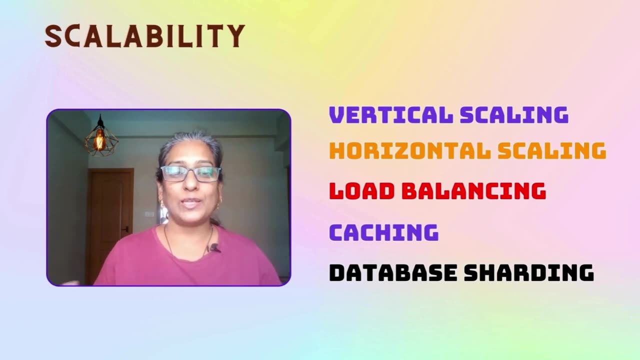 behind every successful digital service. by adopting practical strategies like vertical and horizontal scaling, load balancing, caching and database sharding, we can build systems that can handle exponential growth. so, whether launching a new app or simply ensuring everything services can handle whatever comes their way, scalability is the key to business success. if you found this, 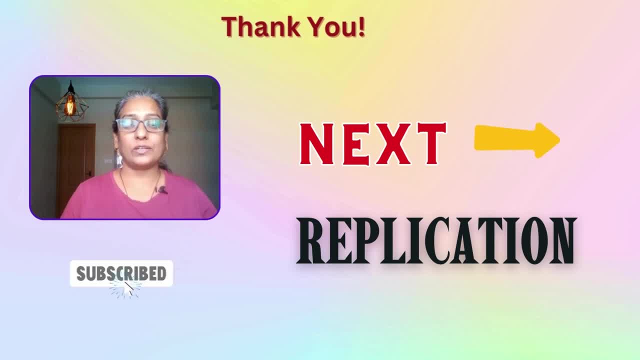 video helpful. give us a thumbs up and subscribe to our channel for more such interesting topics. do check out our other videos on software performance optimization, case studies, coding, big data and career growth. my name is rupa and i thank you so much for watching this video. see you next time. 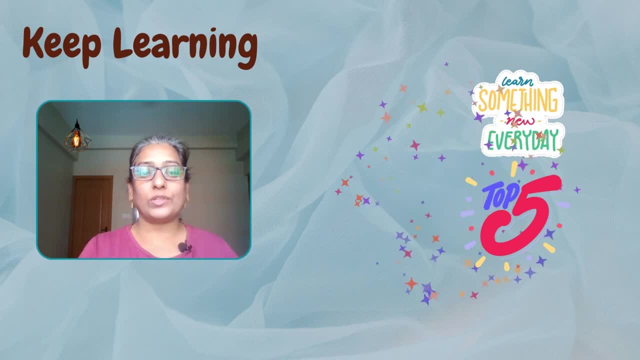 before we get into the details, let me emphasize the importance of staying updated and continuously learning. in the tech world, with new advancements and innovations emerging every day, it's crucial to keep honing our skills. check the description box for some learning resources covering coding, system design and advanced computer science concepts. 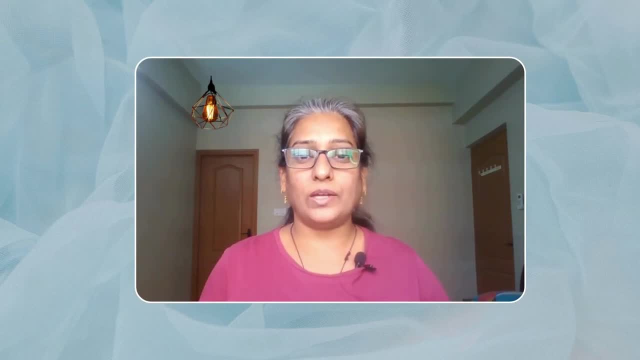 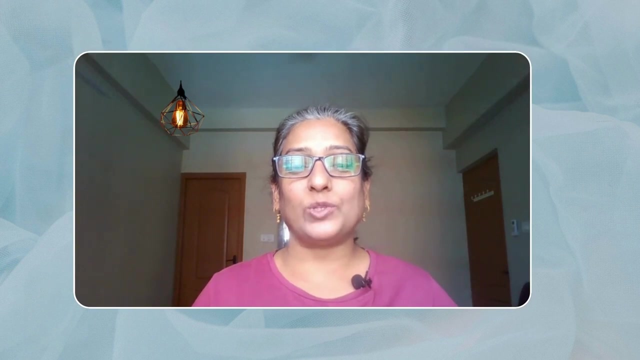 do you know how companies like amazon, netflix and google maintain reliability, availability and scalability in their large distributed systems? today we are diving deep into the world of replication and its critical role in maintaining smooth operation of large distributed systems. hi there, welcome to tech and career bites. i'm a software professional with the 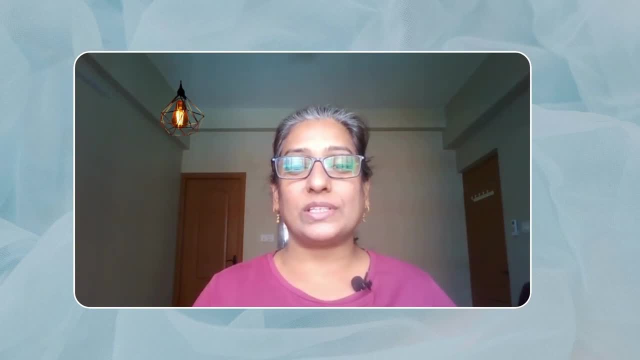 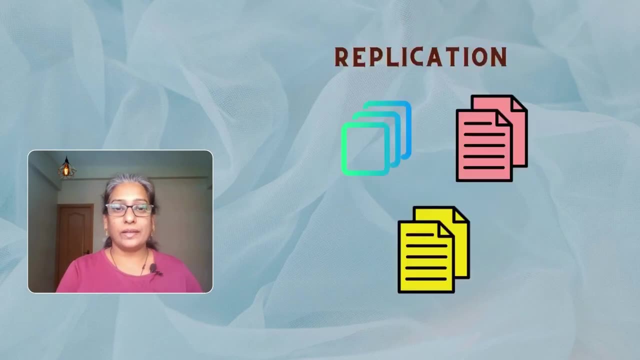 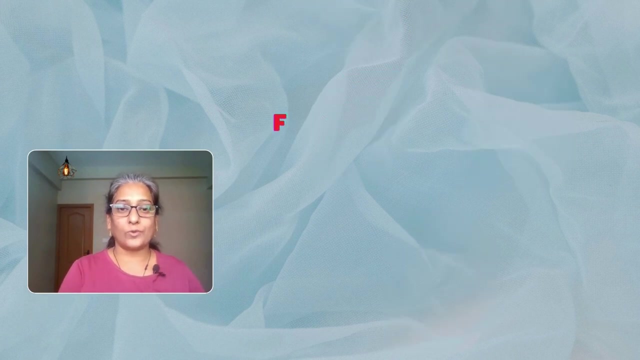 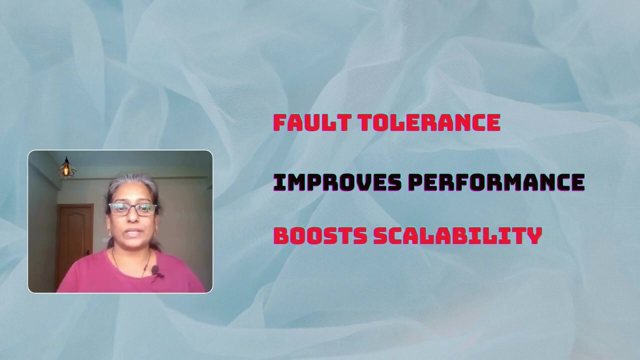 over two decades of experience, including seven years in leadership roles at a global product based organization. replication and distribution systems is all about creating and maintaining copies of data and resources across multiple nodes. doing so enhances support, tolerance, improves performance and boosts scalability. let's understand what each of these means by replicating data across. 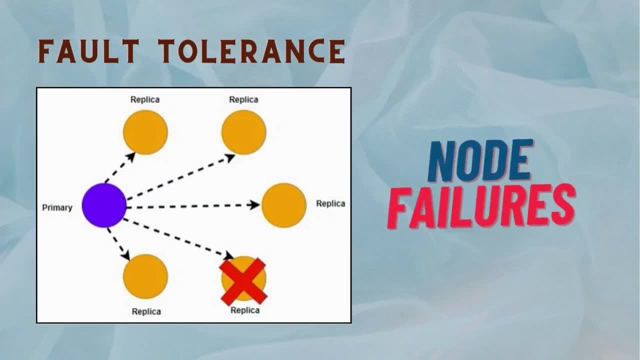 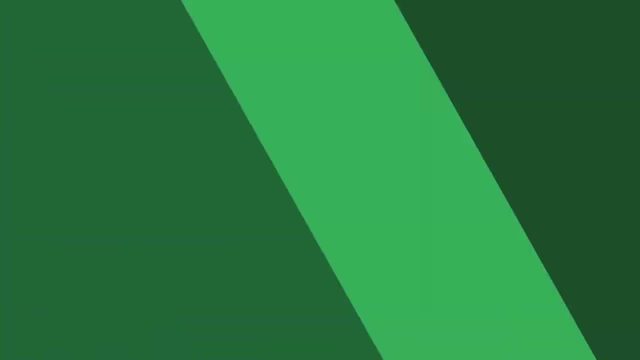 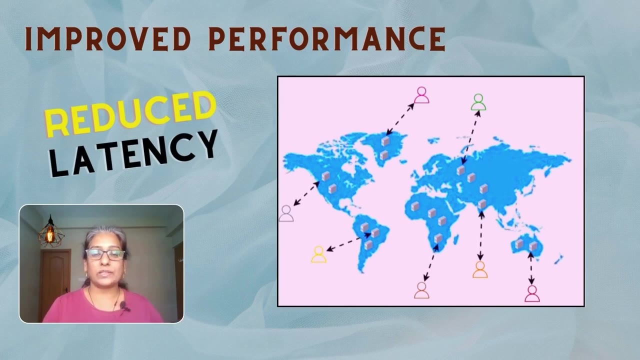 multiple nodes systems can withstand and maintain data across. multiple nodes systems can withstand individual node failures. This improves overall system reliability and availability, even in the face of node failures. Replicating and locating data closer to users reduces access latency. This enhances overall performance and the responsiveness of distributed applications. 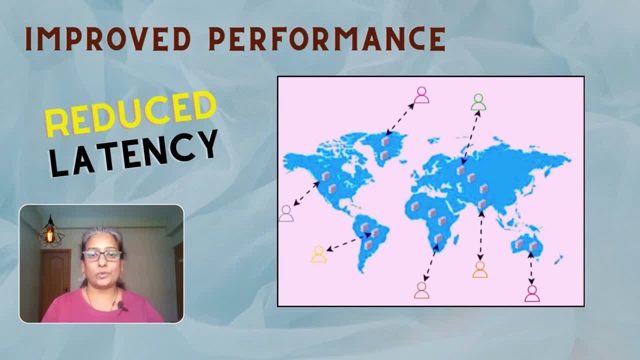 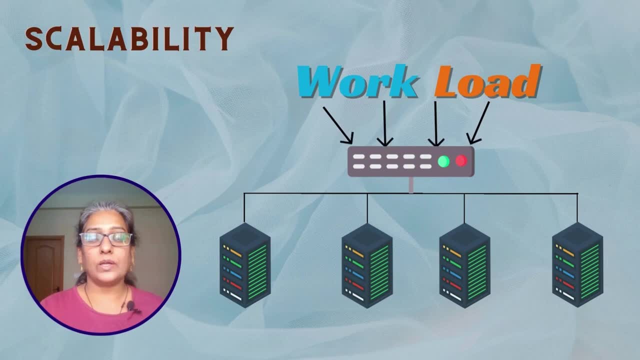 We have a separate video dedicated to the topic of software performance metrics. Please watch that to gain more insights. Scalability enables the systems to handle increasing workload and user traffic by distributing the data access and processing across multiple nodes. Please watch our video on scalability to learn more. 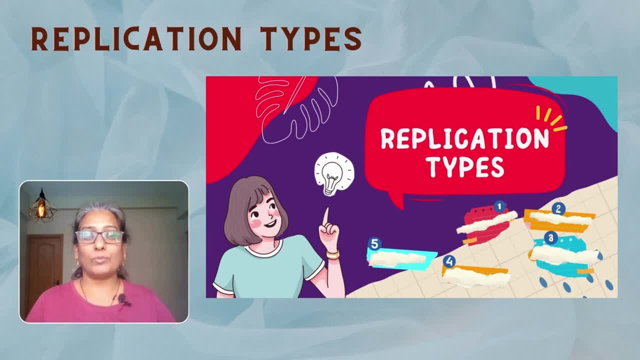 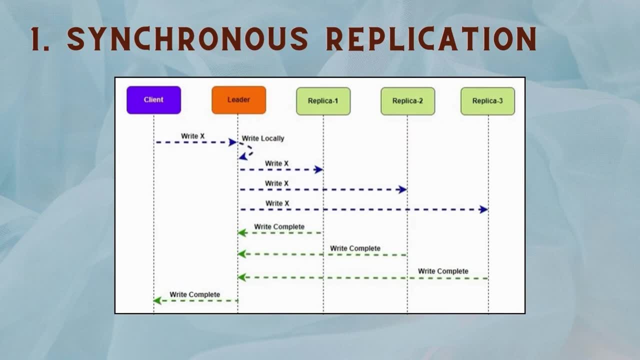 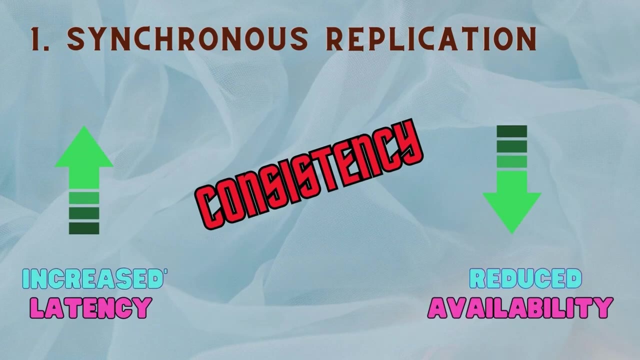 Now let's explore various replication types employed in distributed systems. In synchronous replication, data modifications are acknowledged only after they are successfully replicated to all designated replicas. This ensures consistency, but may introduce latency and reduce availability. This replication type is ideal for scenarios requiring strict consistency guarantees. 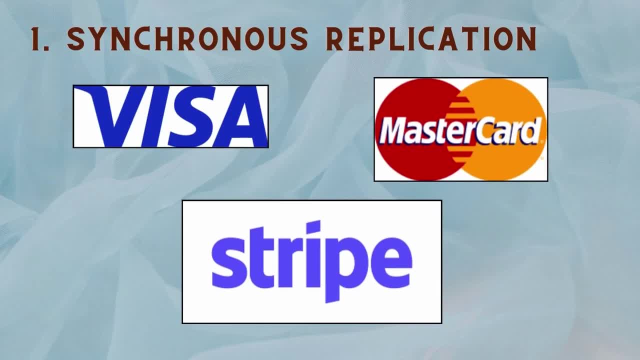 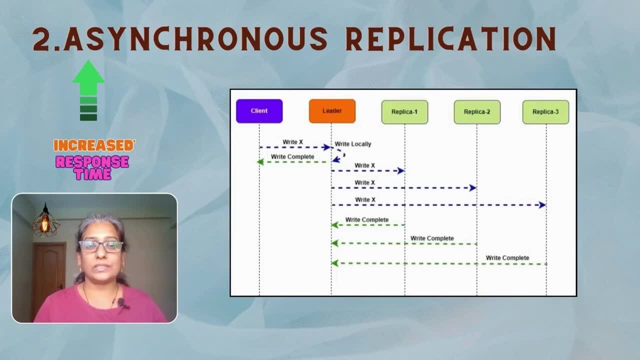 such as financial transactions or critical data updates. Irresynchronous replication speeds up the response time by acknowledging the data changes before replicating them to all the replicas. However, this can lead to data consistency issues if a node fails. This replication is suitable for applications prioritizing performance and 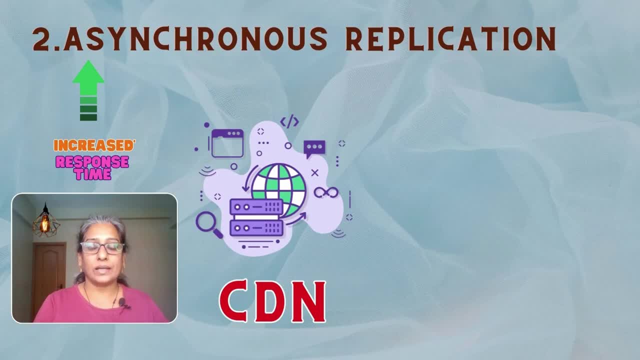 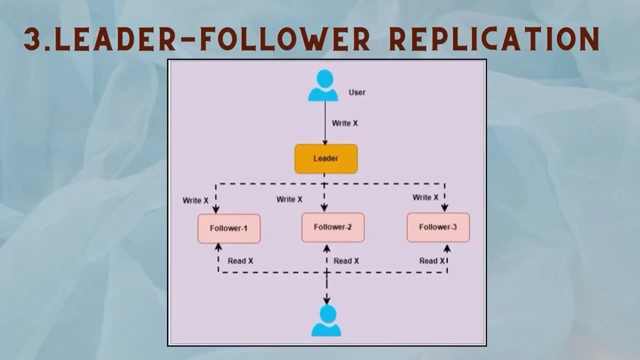 availability over strict consistency, such as content delivery networks or social media platforms. In leader-follower replication, one node, the leader, handles all right operations propagating changes to follower nodes asynchronously or synchronously. This model simplifies consistency but may introduce bottlenecks and single points of failure. 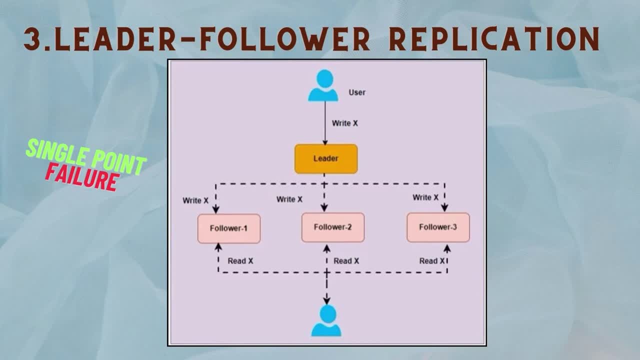 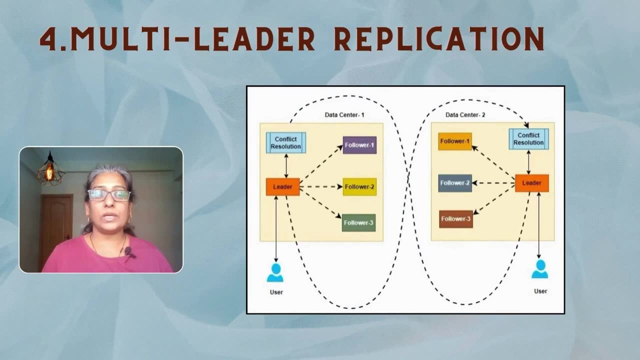 Leader-follower replication is effective for systems with a clear distinction between read-heavy and write-heavy workloads. Multi-leader replication allows multiple nodes to accept right operations independently, propagating the changes to other nodes either synchronously or asynchronously. This approach improves scalability and performance. 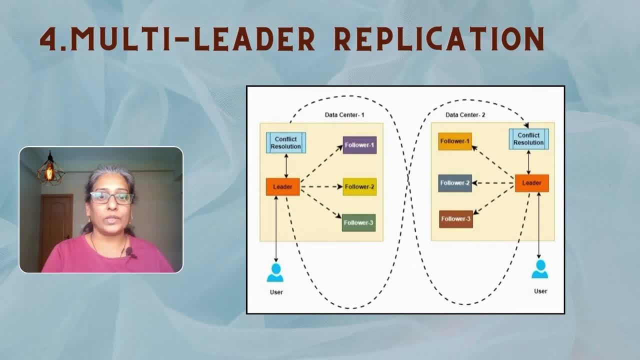 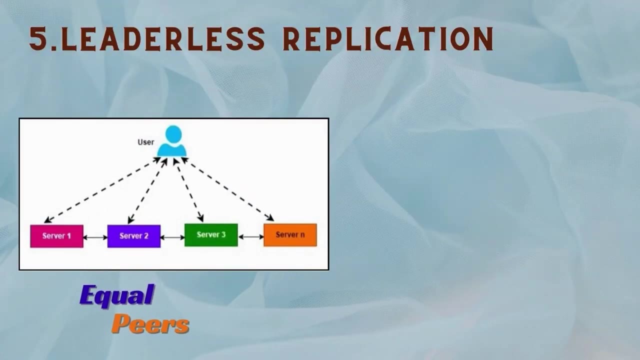 but requires complex resolution mechanisms to ensure consistency. Multi-leader replication approach is often employed in globally distributed systems for replication across distribution centers. In leader-less replication, all nodes are equal peers accepting read and write operations independently. This model offers high availability and scalability, but requires consensus protocols. 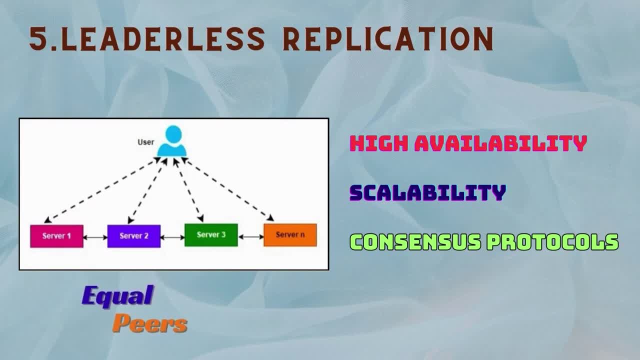 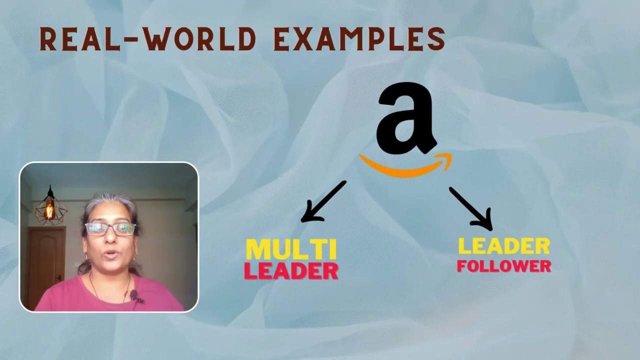 to maintain consistency. Leader-less replication cannot be synchronous due to the inherent difficulties and compromises involved in achieving synchronous replication without a leader. Leader-less replication is recommended for highly scalable systems with decentralized architectures where the emphasis is on fault tolerance and horizontal scalability. Amazon uses a combination of multi-leader and leader-follower replication strategies. 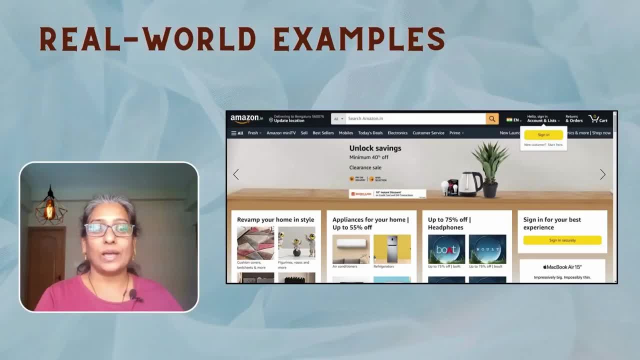 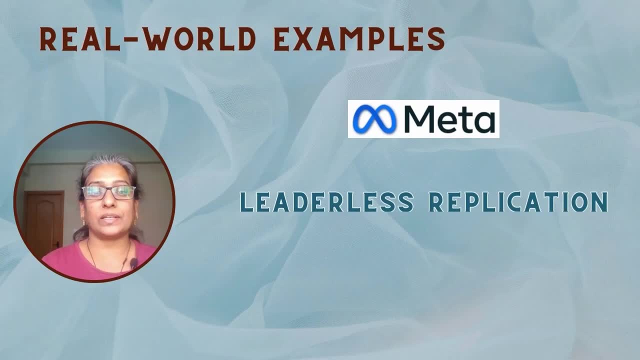 to ensure high availability and consistency across its globally distributed e-commerce platform, Meta utilizes leader-less replication techniques enabling seamless interaction and content delivery, allowing users to use the platform in multiple ways. The platform is designed to be a platform for millions of users worldwide on its social media. 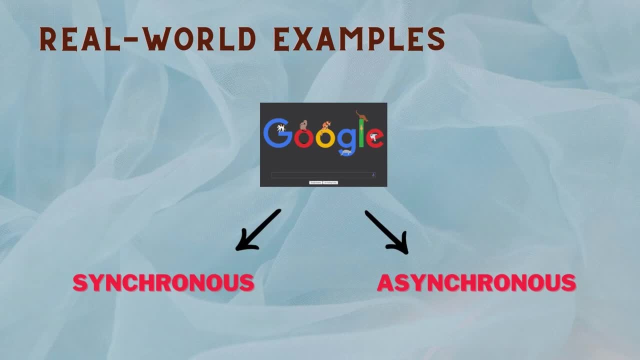 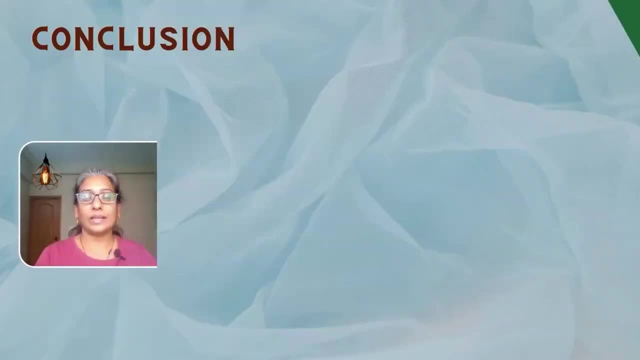 platform. Google employs a mix of synchronous and asynchronous replication approaches tailored to the specific requirements of its diverse portfolio of services, including Google Search and Google Cloud platform. In conclusion, replication serves as the backbone of distributed systems, offering solutions to scalability, availability and reliability challenges. 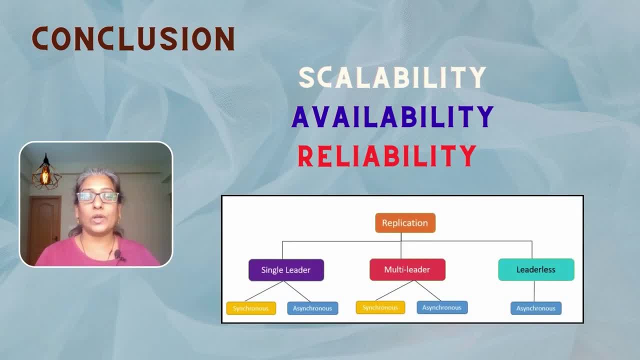 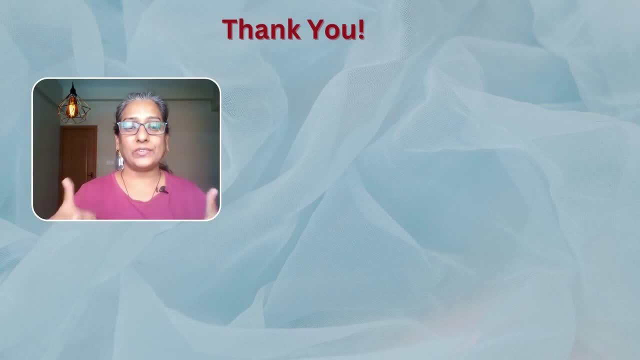 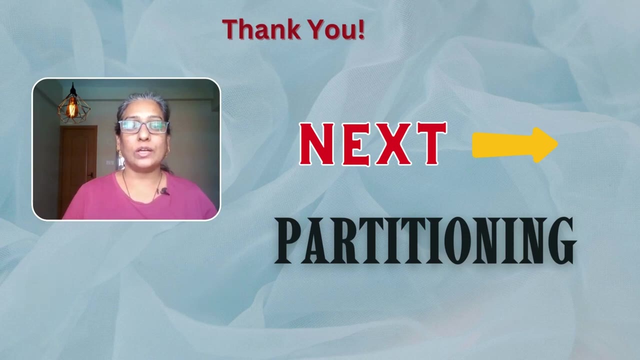 Different replication methods work and where they are best used. organizations can design strong and effective distributed systems. If you found this video helpful, give us a thumbs up and subscribe to our channel for more such interesting topics. Do check out our other videos on software performance. 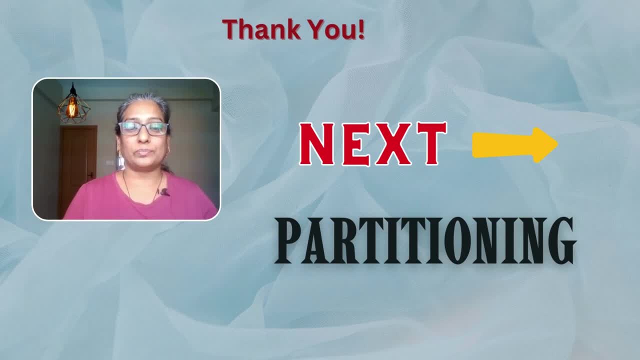 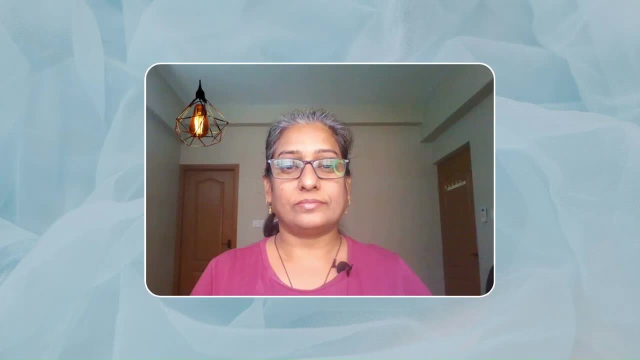 optimization, case studies, coding, big data and career growth. My name is Rupa and I thank you so much for watching this video. See you next time. In this video, let's explore partitioning- the various partitioning techniques used in. 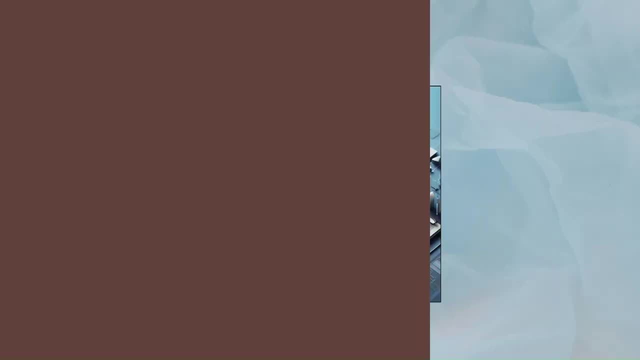 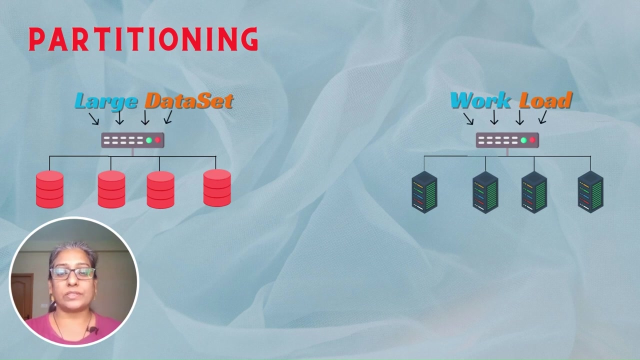 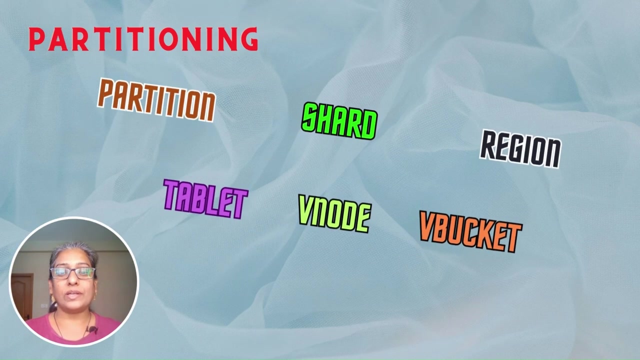 distributed systems and the benefits of partitioning. Partitioning in distributed systems involves dividing large data sets or workload into smaller partitions for better performance, availability and scalability. What we call a partition here is called a shard in MongoDB and Elasticsearch. It is also known as 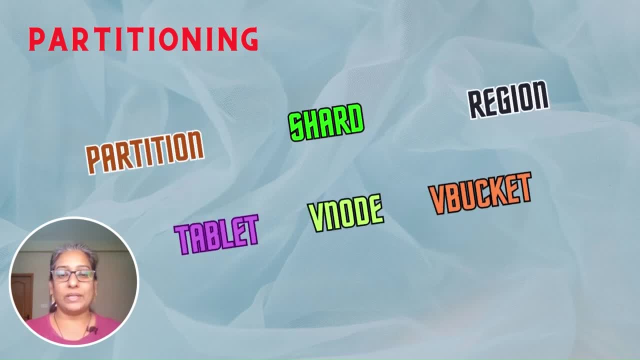 a region in HBase, a tablet in MongoDB and Elasticsearch. It is also known as a region in HBase, a tablet in MongoDB and Elasticsearch. It is also known as a region in HBase, a tablet in Bigtable, a vNode in Cassandra and React and a vBucket in Couchbase. 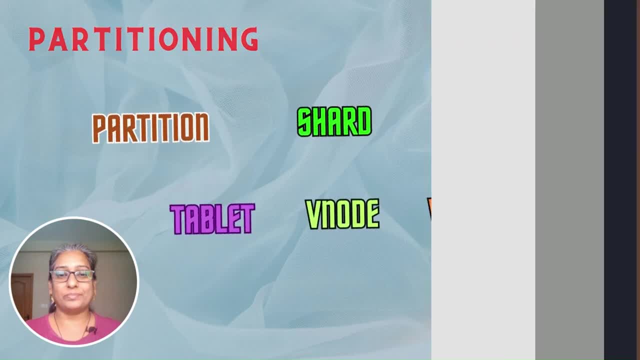 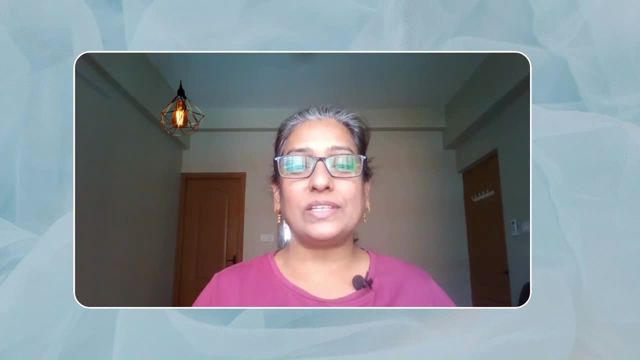 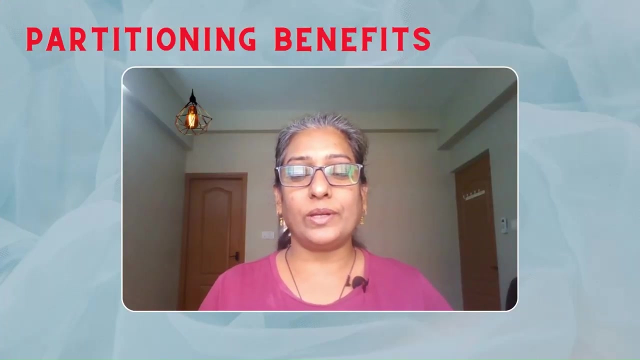 So not to get confused, they all mean the same. Hi there, welcome to Tech and Career Bites. I'm a software professional with over two decades of experience, including seven years in leadership roles at a global product-based organization. Let's dig deeper to understand the benefits of partitioning. 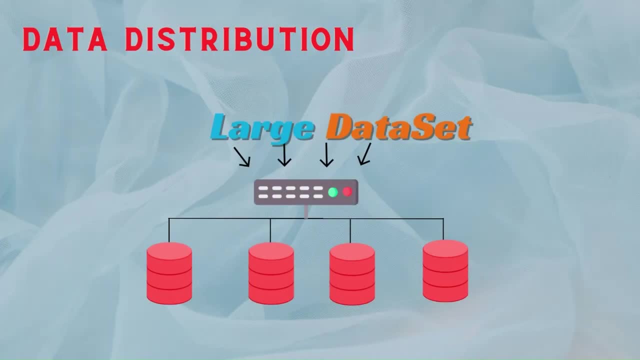 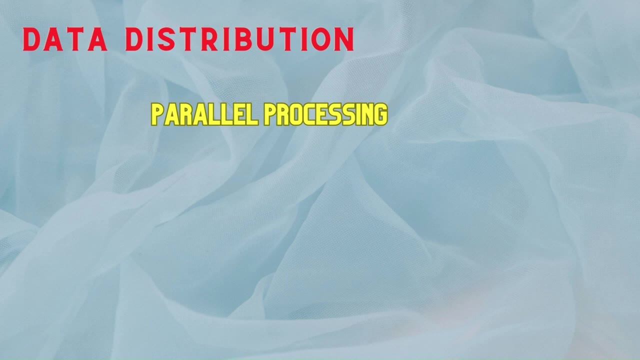 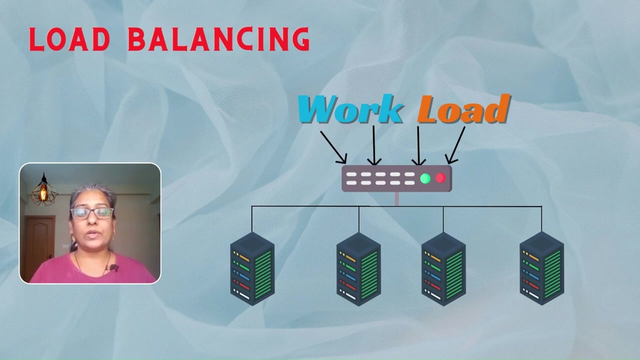 Partitioning a data set distributes it across multiple nodes or machines. It is a very simple process, but it is very easy to understand. Each node handles a specific partition enabling parallel processing. This boosts performance and reduces processing time. Partitioning helps evenly distribute the workload across the nodes in a distributed system. 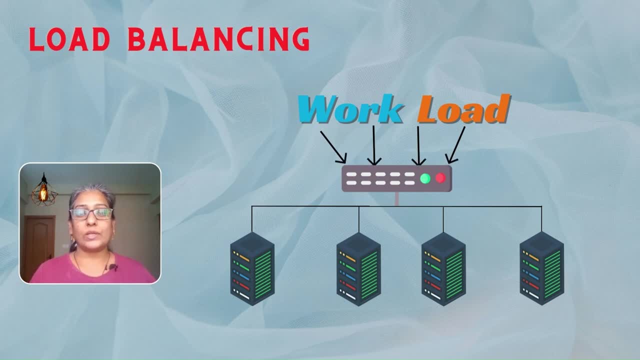 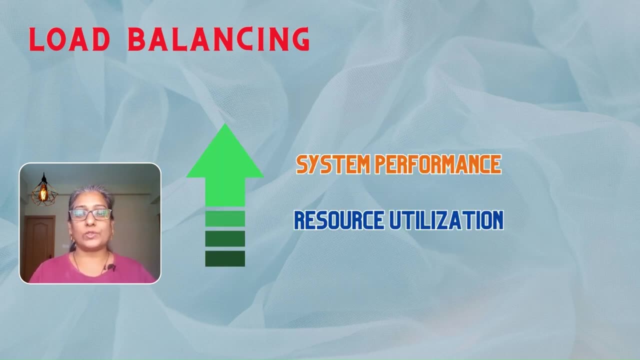 This load balancing approach ensures that no single node is overloaded, while others are underutilized. This maximizes system performance and resource utilization. Partitioning lets a system scale horizontally. This maximizes system performance and resource utilization. Partitioning lets a system scale horizontally. 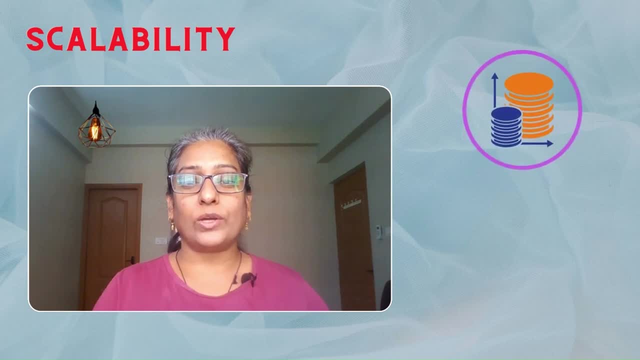 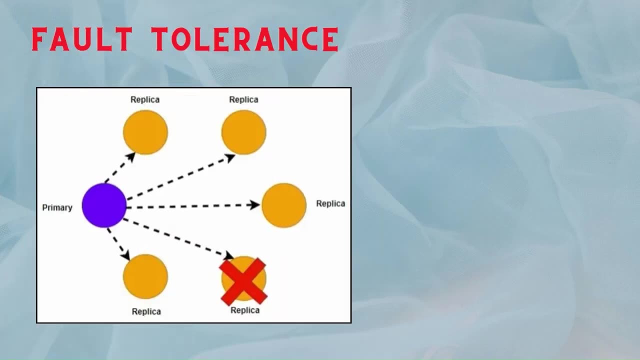 This maximizes system performance and resource utilization. This enables the system to handle more data or users To know more. watch our video on scalability. Partitioning provides a port tolerance and high availability. Even if a portion of the system becomes unavailable, the remaining partitions and nodes can continue to function. 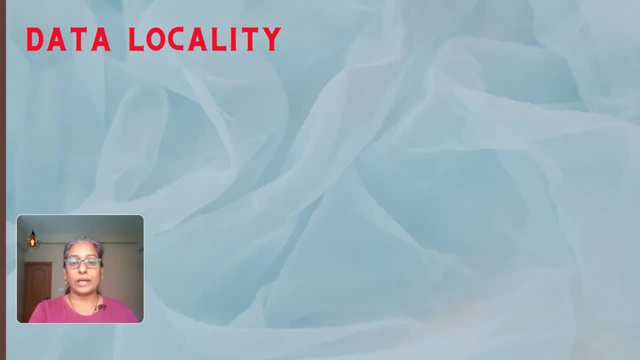 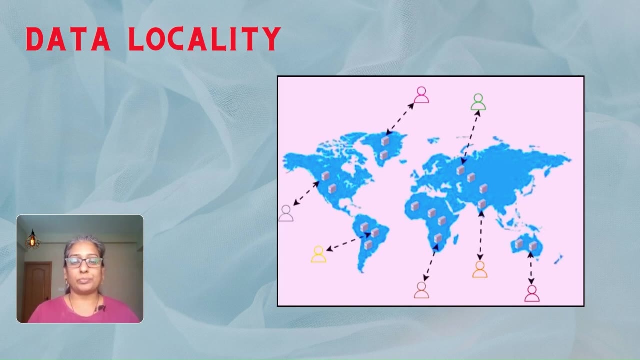 maintaining the overall system's availability. Partitioning can also be used to optimize the data locality, where data is stored and processed closer to the computing resources. Data locality minimizes the load balancing and resource utilization. Data locality minimizes the load balancing and resource utilization. 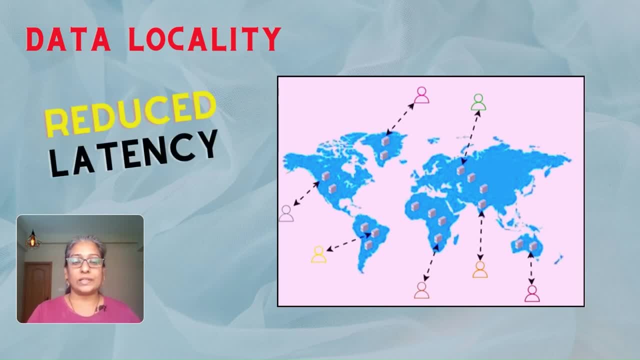 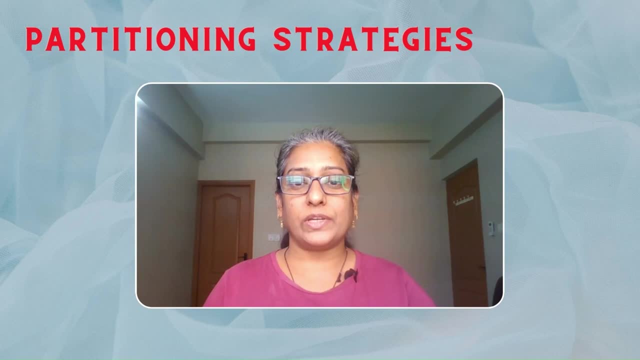 Data locality minimizes the load balancing and resource utilization. Data transfer across the network: reducing latency and improving the overall system performance. Data transfer across the network: reducing latency and improving the overall system performance. Partitioning techniques vary based on the specific requirements and the characteristics of data and the distributed system being used. 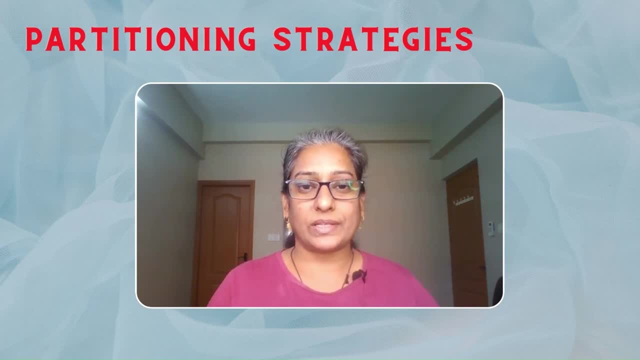 Partitioning techniques vary based on the specific requirements and the characteristics of data and the distributed system being used. Let's discuss some of the common data partitioning techniques. Let's discuss some of the common data partitioning techniques. There are two different types of data partitioning. 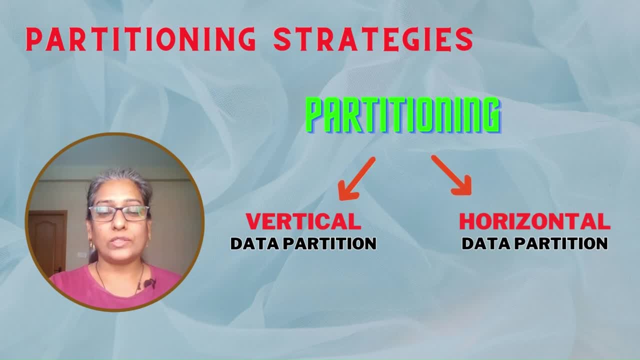 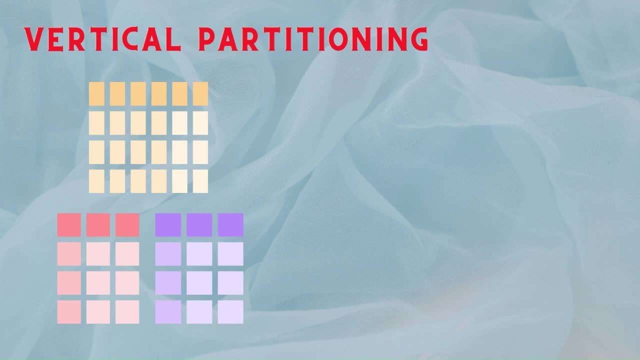 is a data partitioning technique where a table is divided vertically based on columns. is a data partitioning technique where a table is divided vertically based on columns. In this approach, columns with similar characteristics or access patterns are grouped together in separate partitions. Normalization is one way to perform vertical partitioning. 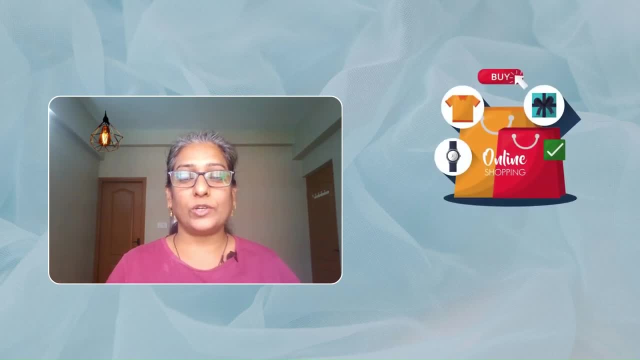 Let's consider an example of vertical partitioning in the context of an e-commerce application that manages customers' information. In the context of an e-commerce application that manages customers' information. In the context of an e-commerce application that manages customers' information. 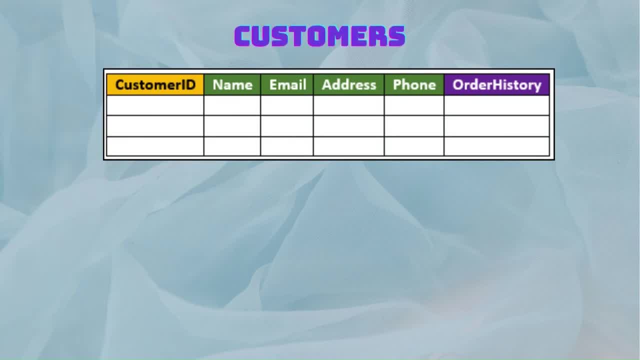 In a traditional table structure, you might have a single table called customers, with columns such as customer ID, name, email address, phone and order history. with columns such as customer ID, name, email address, phone and order history. 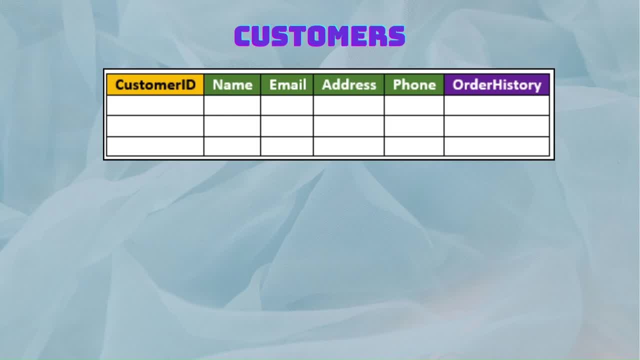 All these columns are stored together for each row representing a customer. With vertical data partitioning, we can partition the table based on the logical relationships between columns. based on the logical relationships between columns, Let's say we decide to vertically partition the customers table into 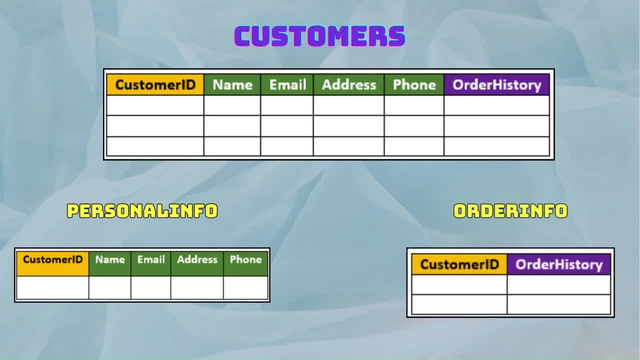 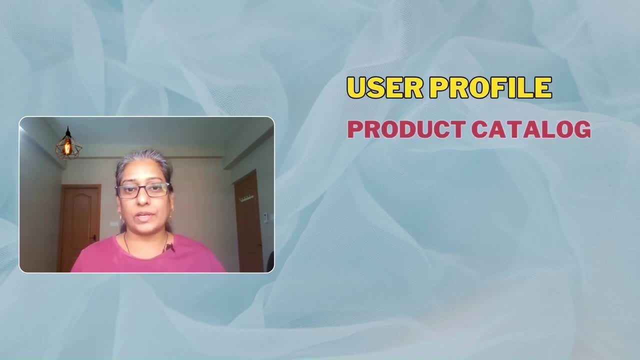 two partitions personal info and order info. two partitions personal info and order info. Let's say we decide to vertically partition. the customers table into two partitions personal info and order info. Vertical data partitioning is typically performed on user profile, product catalog. 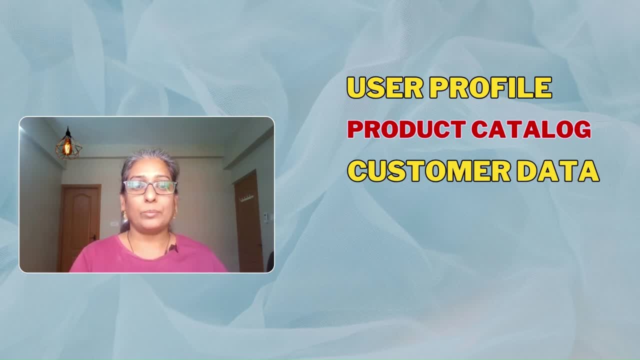 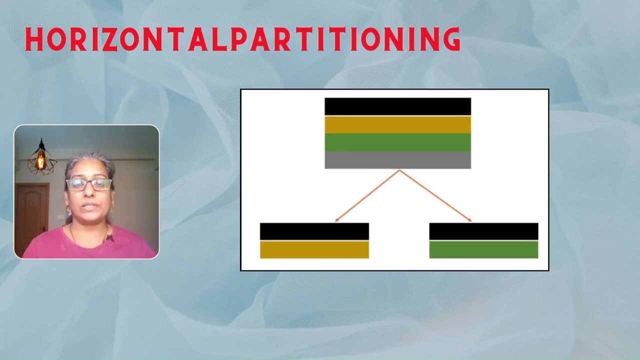 and customer-related data in e-commerce and patient records and medical data in healthcare and customer-related data in e-commerce and patient records and medical data in healthcare. In horizontal data partitioning, a table is split into smaller multiple tables where each table contains a subset of the original table rows. 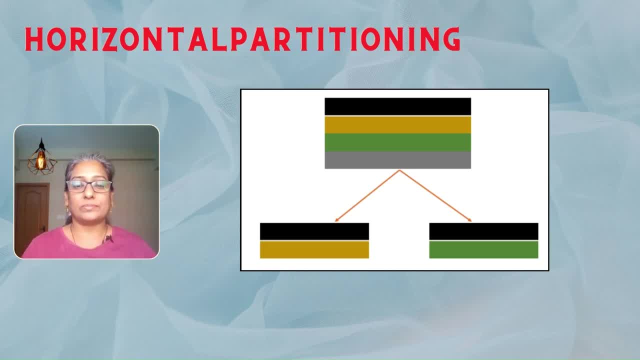 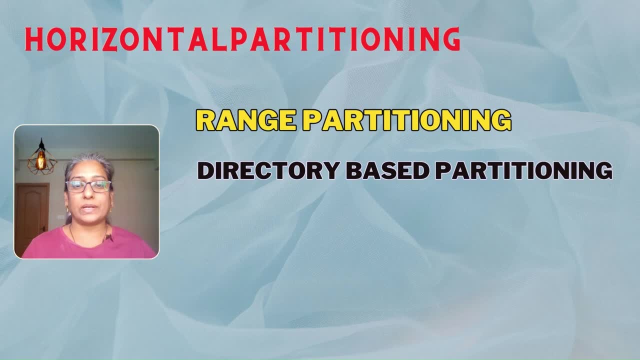 These subsets are then placed on different nodes. Some of the popular horizontal data partitioning techniques are Range Partitioning, Directory-based Partitioning, Hash Partitioning and Partitioning based on Consistent Hashing. We will be discussing each one of these in detail, so don't go anywhere and stay tuned. 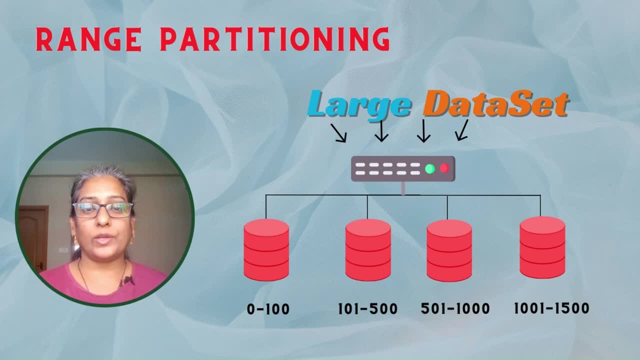 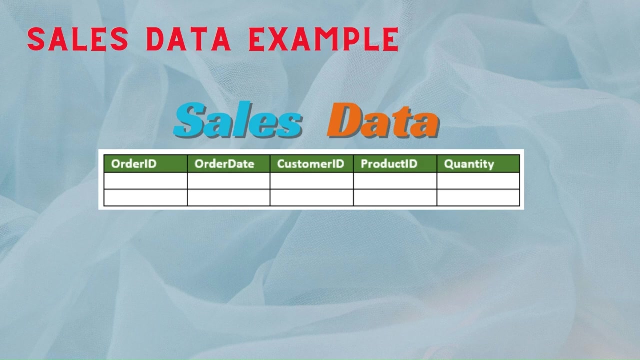 In range partitioning, data is divided into partitions based on a specific range criteria. Each partition then contains a particular range of data, predefined range of values. Let's consider an example of range partitioning in the context of a sales database. We have a table named sales data with columns order id, order date, customer id. 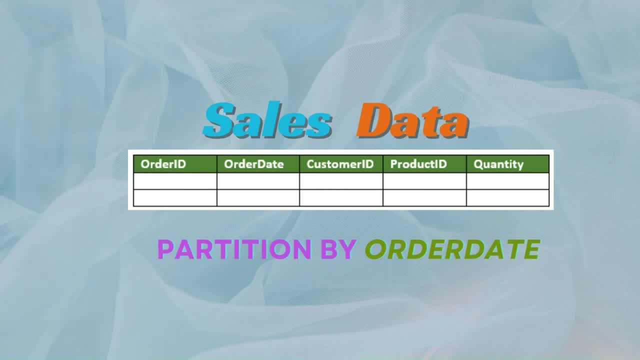 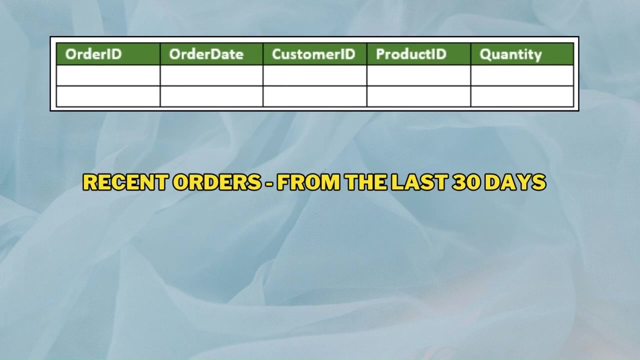 product id and quantity To apply range partitioning: we divide the sales data table based on the order date column which shows when each order was placed. Here is how we split the data into three partitions. First partition: recent orders containing the last 30 days orders. 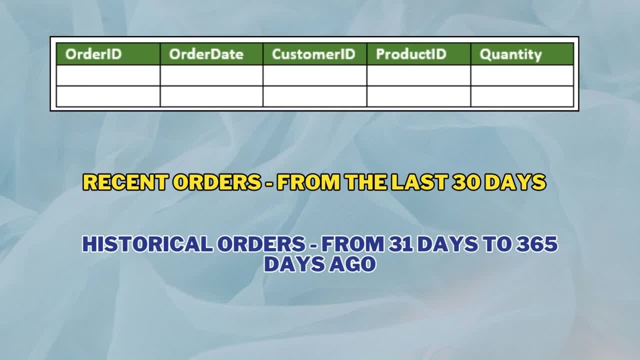 Second partition, historical orders, which contains orders from 31 to 365 days ago, and the third partition- archived orders, containing orders older than 365 days. Each order is stored in the partition that matches its order date. New orders go into the recent orders. 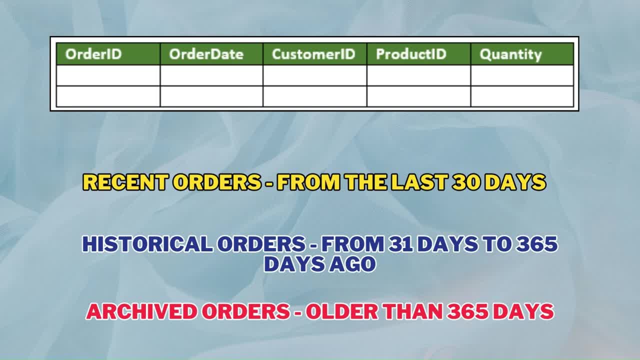 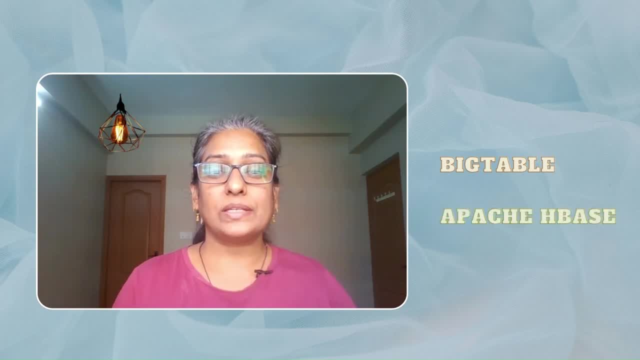 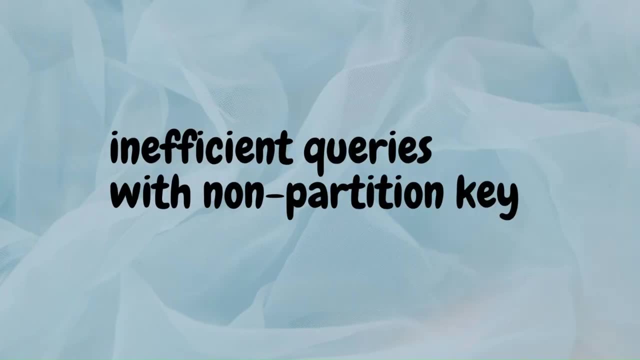 Second orders partition and as time passes, orders move to different partitions based on how old they are. Google's Bigtable and Apache HBase seem to leverage range partitioning. However, range partitioning has its limitations. In range partitioning, efficient range queries. 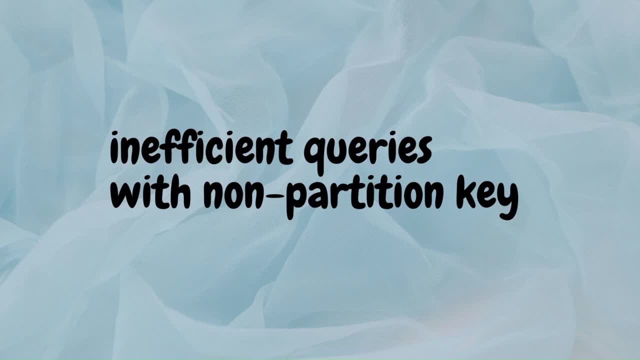 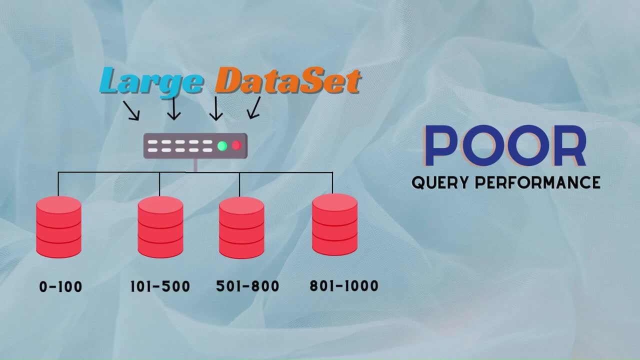 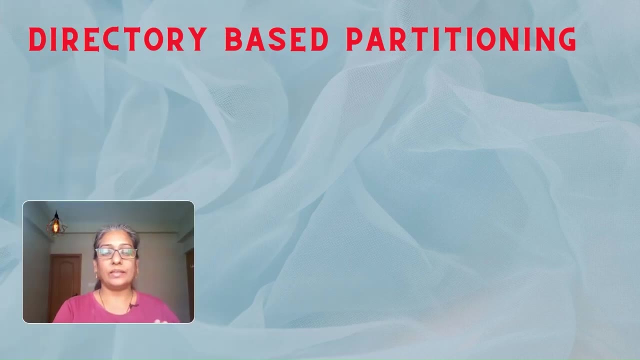 can only be done using the partition key, not other keys. Plus, if a big range spans multiple nodes, query performance suffers. Data distribution may be uneven if one range has more data than others. In directory-based sharding, the data items are distributed across the shards based on. 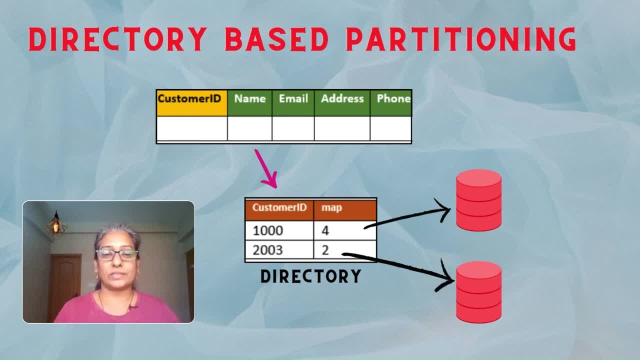 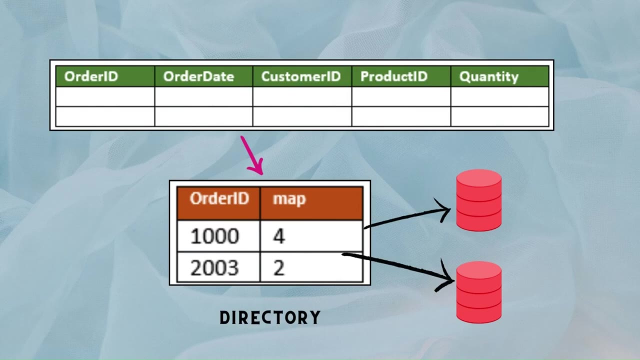 explicit mappings maintained by a centralized directory or metadata service. This approach is beneficial when there is a need for a centralized control over data distribution and routing in a distributed system. Consider an example of directory-based sharding. in an e-commerce sales database, For instance, the data that was transferred will be stored in this directory as a archer. 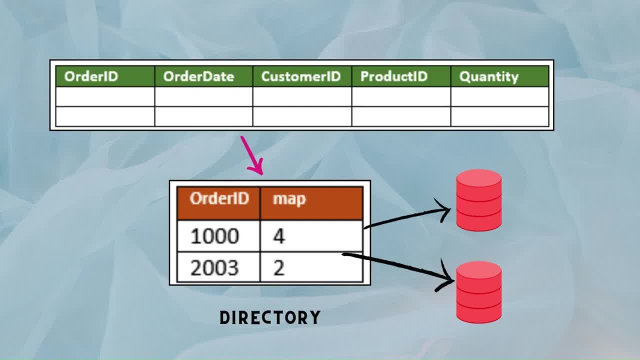 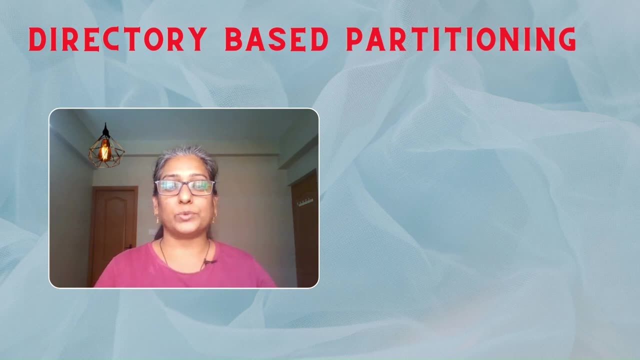 망 vaakas per release date and countless的时候. secure frame takes era of balance, ratio andい instead of predefined ranges. a central directory maps each order to a shard based on its id. When accessing or modifying data, the directory routes a request: the correct shard. 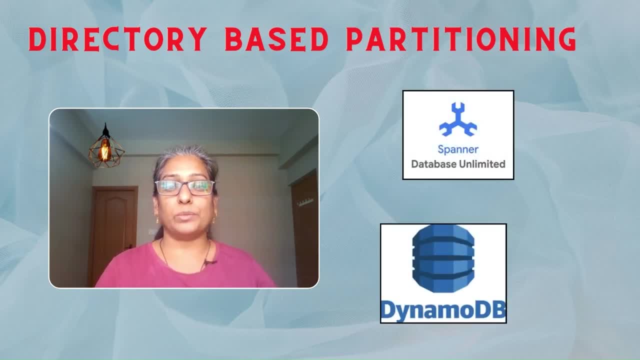 Directory-based sharding centralizes control over data distribution, but the directory becomes the single point of failure. Google's Spanner and Amazon's DynamoDB uses США's directory-based sharding to control over data distribution. In this way, the directorless sharding becomes a single point of failure. Google's Spanner and Amazon's DynamoDB uses directory-based sharding. 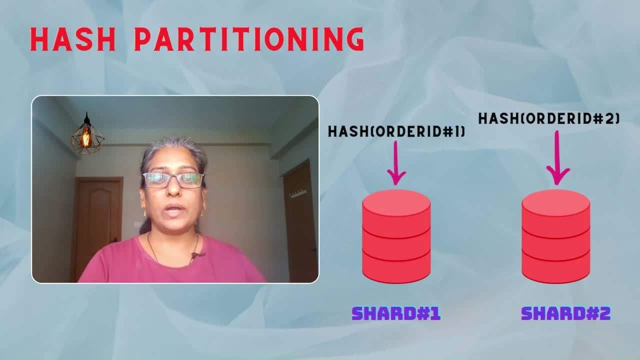 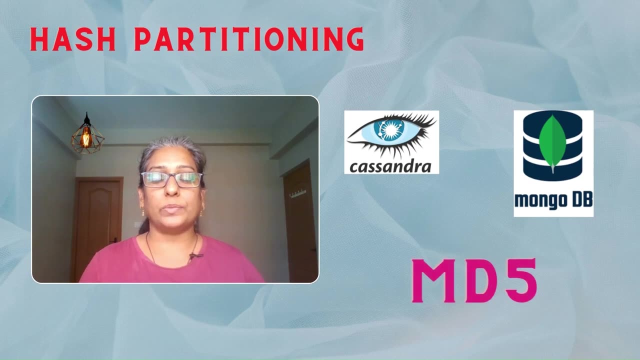 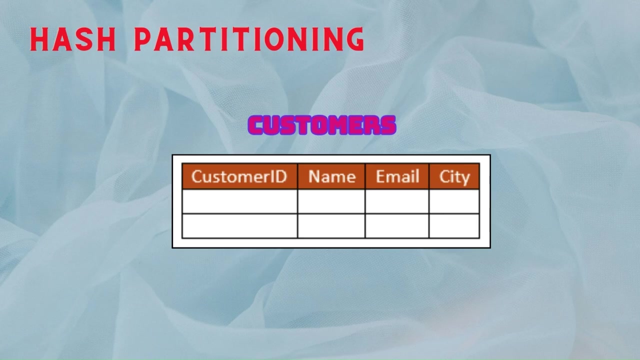 hash partitioning divides the data into partitions using a hash function on a column. for example, cassandra and mongodb use md5 as the hash function. let's consider an example of a hash partitioning a customer database. we have a table called customers with the following columns: 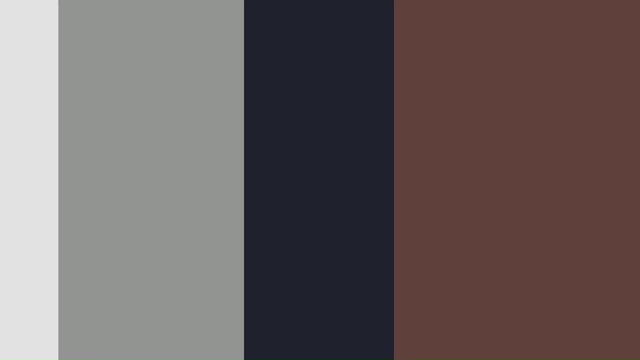 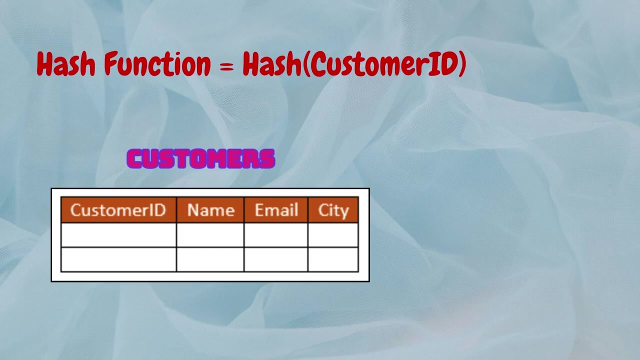 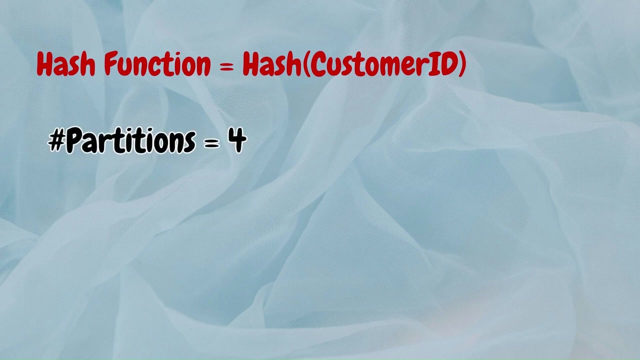 customer id name, email and city. to apply hash partitioning: we partition the customers table based on the customer id column. the partitioning process involves the following steps. first step: determine the number of partitions. let's say we want four partitions. then, second step: define the hash function. choose a hash function for the customer id column. lastly, apply the hash function. 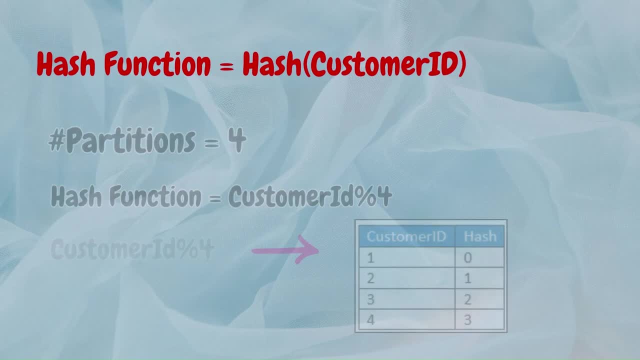 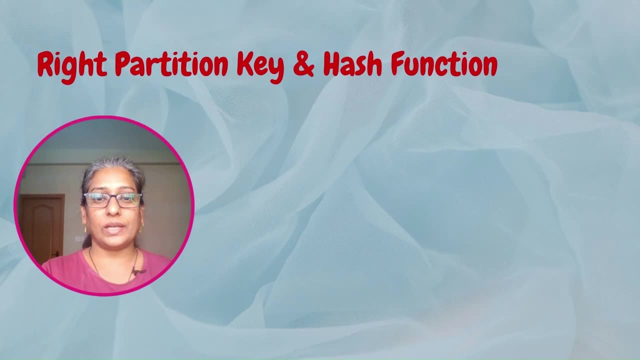 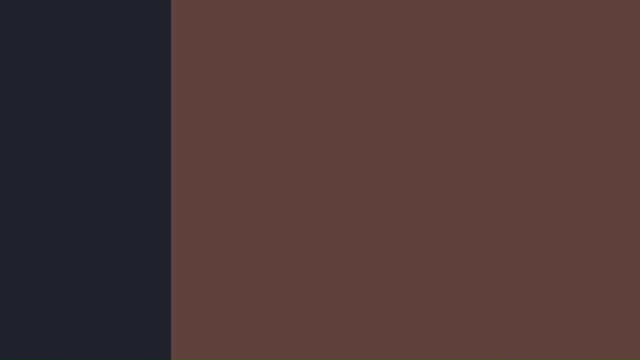 to each customer id. this way, each customer record gets assigned to a partition based on its hashed customer id. choosing the right partitioning key and hash function is vital in hash partitioning to ensure the data is distributed evenly. constant hashing is a smart way to distribute data across. 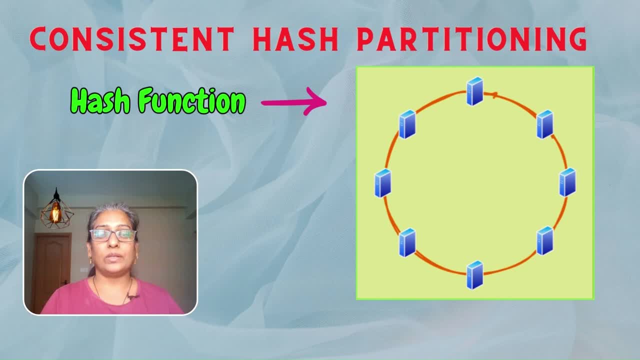 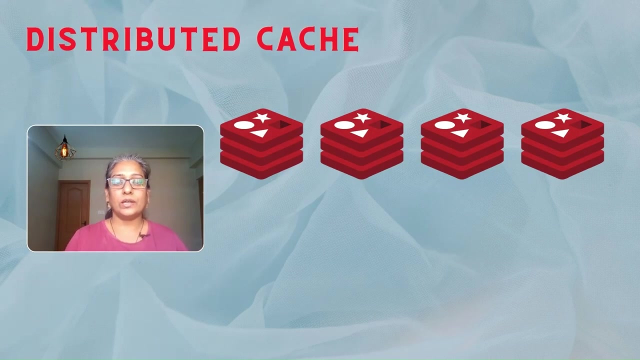 many nodes without the need to move the data around when nodes are added or removed in the cluster. it works by using a hash function and a circular structure to assign data to partitions. let's illustrate consistent hashing with an example of a distributed cache system. suppose we have a distributed cache with four nodes: a, b, c and 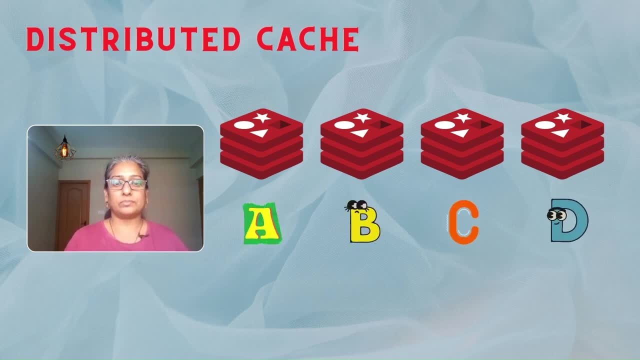 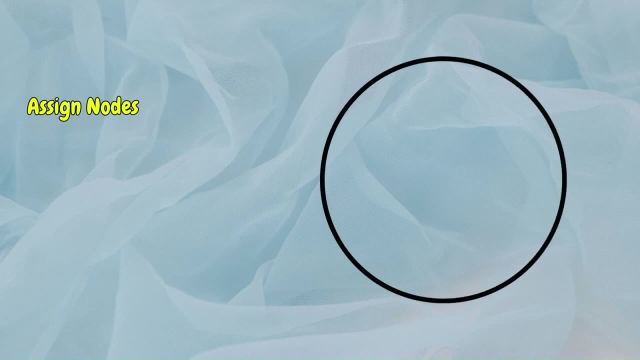 d. each node represents a partition. the partitioning process involves assigning nodes, where we create a circular ring representing all possible hash values. each node is placed multiple times on this ring based on its hash value. after that mapping data, During our retrieving data, we hash its key to get a value. 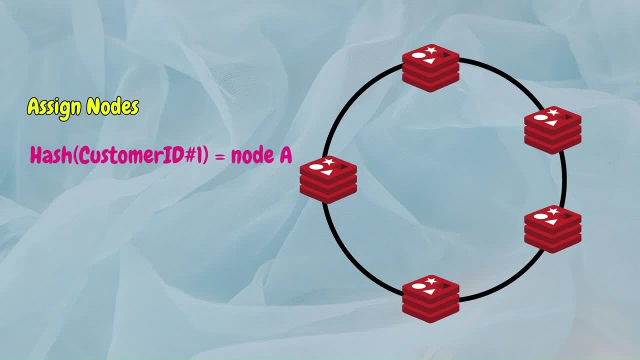 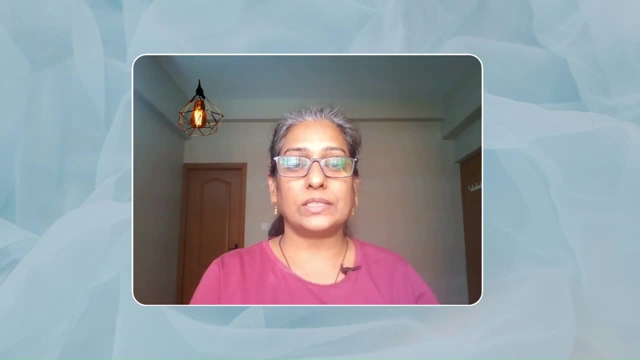 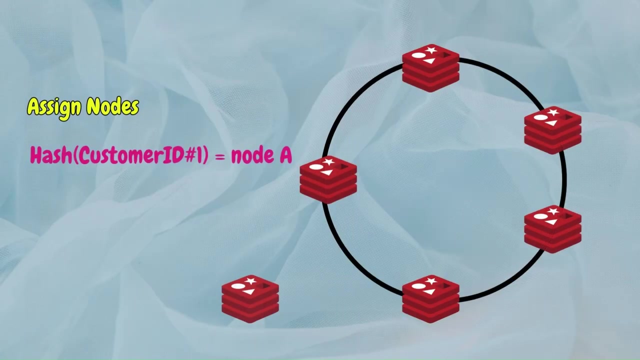 This value is then mapped onto the ring to find the corresponding node. Now let's understand how the partitioning using consistent hashing works when the cluster changes, That is, when we add or remove nodes from the cluster. If we add a new node, like E, its positions on the ring are determined. 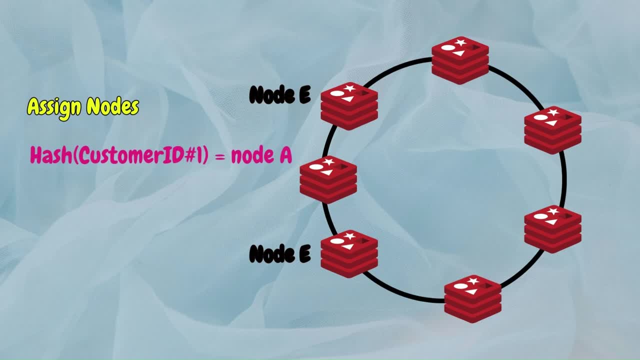 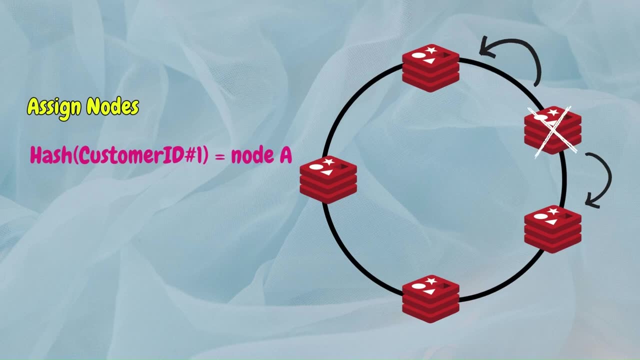 We adjust the positions between existing nodes to balance the load, minimizing the data movement. If a node fails, like C, its keys are redistributed among other nodes. Only a fraction of keys need to be moved as other nodes take over some of the failed nodes'. 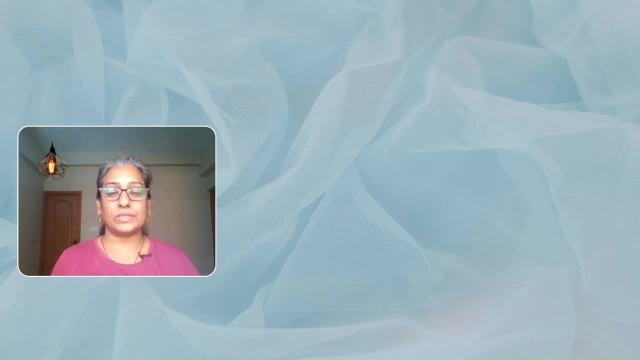 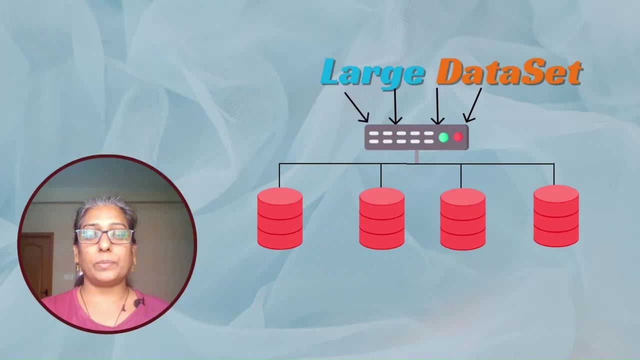 responsibilities. Consistent. hashing is widely used in distributed systems like caches, databases and CDNs. We have explored data partitioning. This is the first example, But how does a client find the right node to connect to for a request? Also, the allocation of partitions to nodes varies after rebalancing which the client 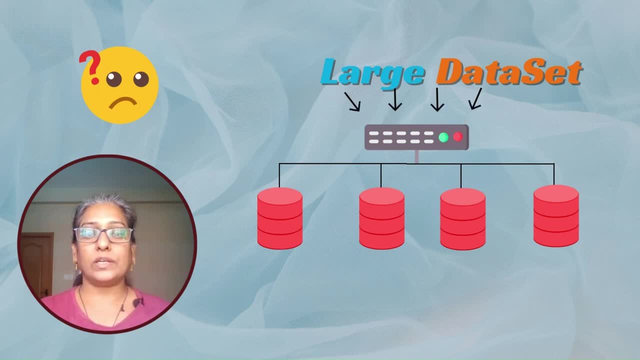 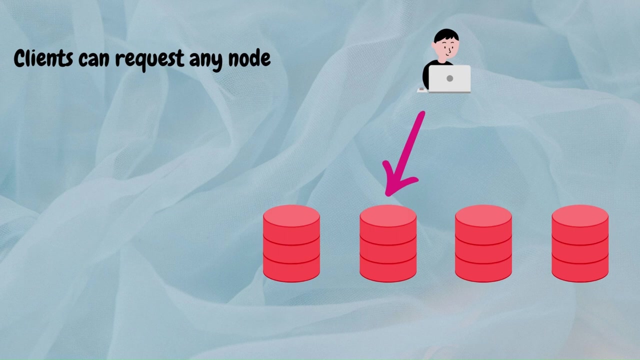 is unaware of. So how does a client find the right node to connect to? This is called service discovery. There are a few methods to handle this. Let's discuss them. In one approach, clients can request any node if it does not have the data it forwards. 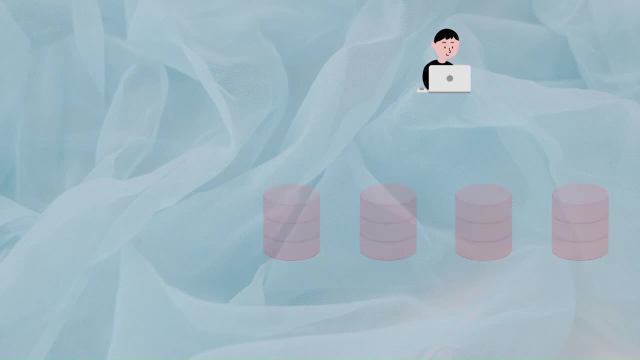 the request to the correct node. Another approach is using a routing tier: Requests are sent there first, which then directs them to the appropriate node. And the last approach is that the clients already know which partition is on which node and can connect directly. 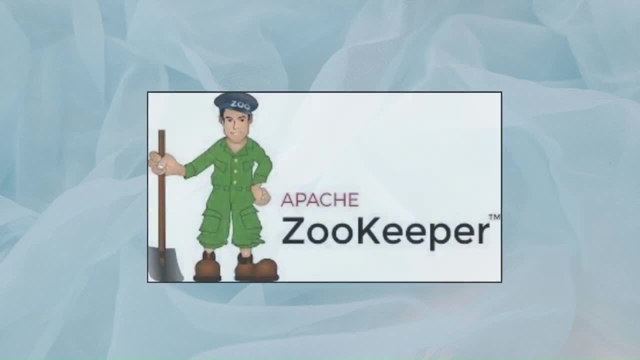 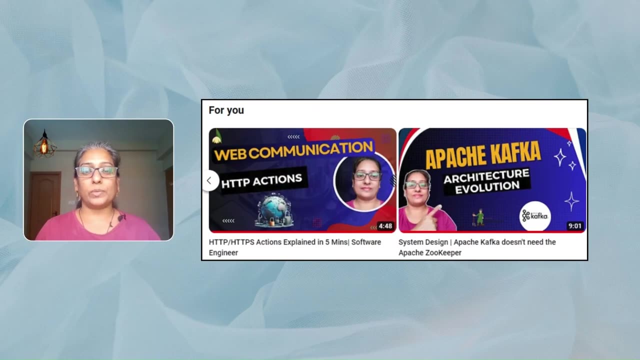 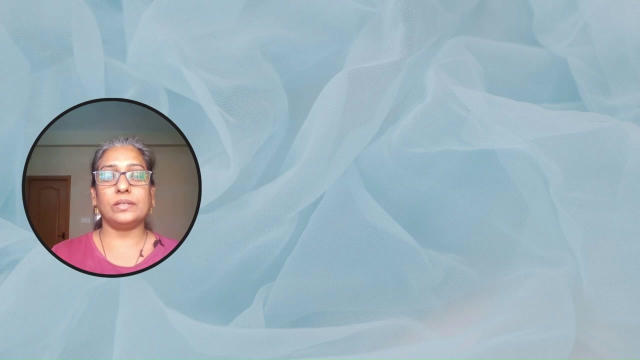 But keeping track of node changes is a challenge. Solutions like ZooKeeper help manage these updates. We have a separate video explaining how ZooKeeper manages Apache Kafka cluster. Please watch it. Thank you, Bye. You can watch that to learn more. Sharding or partitioning helps systems scale and improve performance, but it adds complexity. 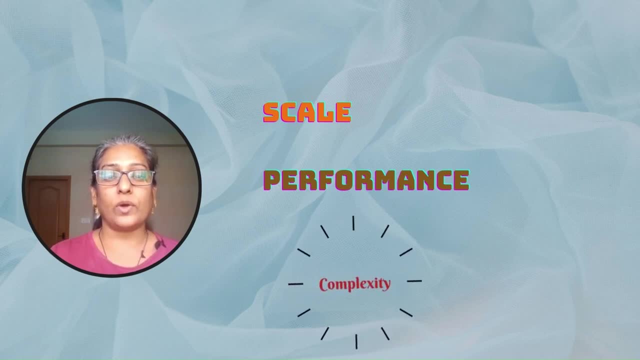 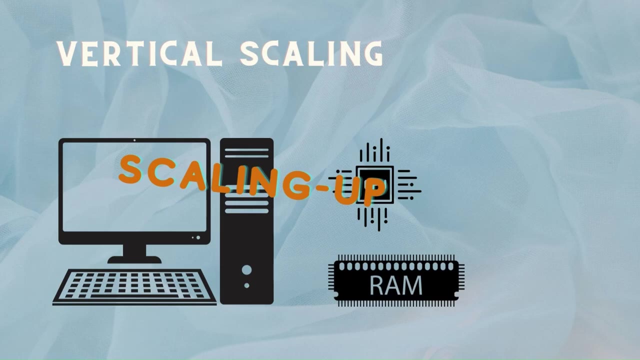 that may not always be necessary. Here are a few alternate approaches. First approach: vertical scaling, where you upgrade a single database server with more resources like CPUs, memory and storage. This is easier to manage than sharding, yet allows a significant expansion. 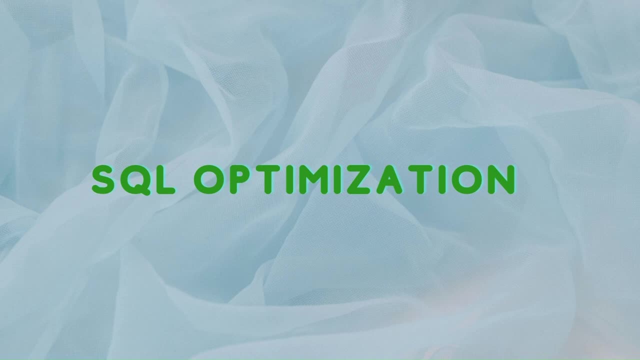 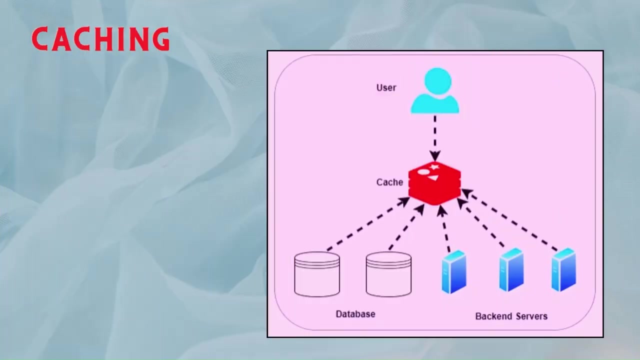 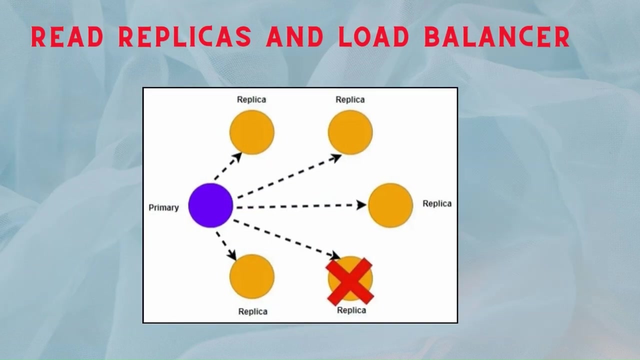 Second, SQL optimization, where SQL queries and database schema are fine-tuned for better performance. Third, caching: Employ in-memory caches such as Redis, to lessen database load by avoiding frequent queries. And fourth approach: use combination of read replicas and load balancers. 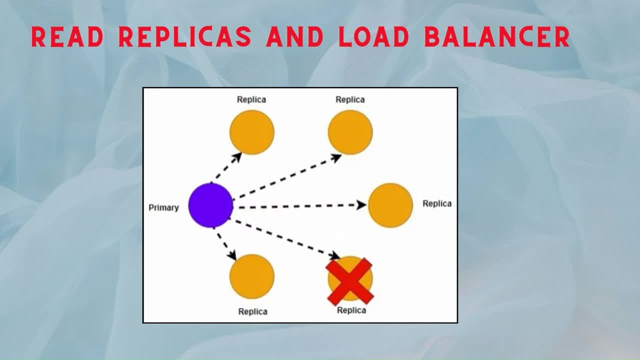 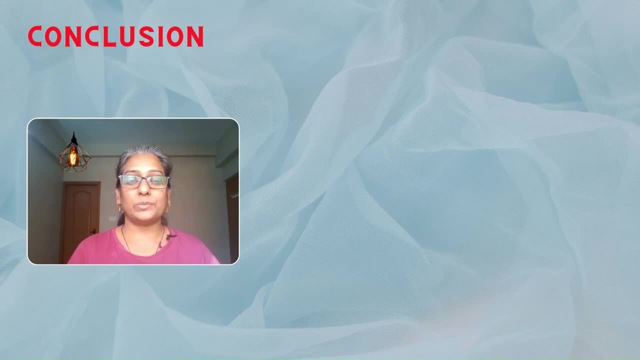 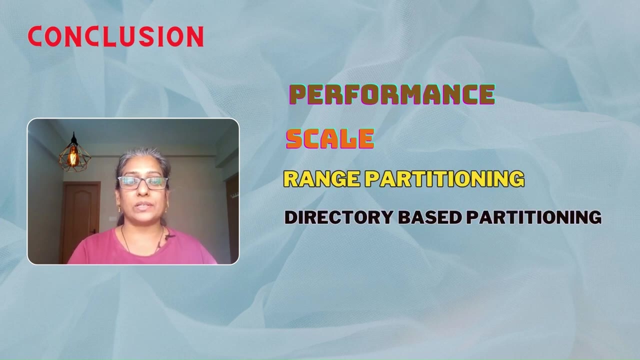 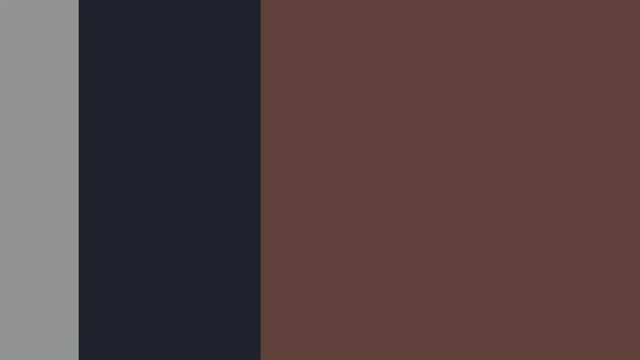 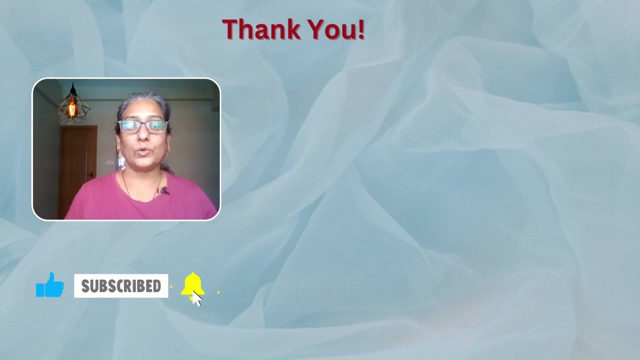 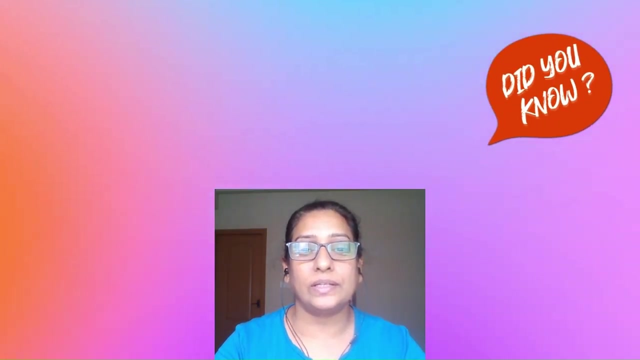 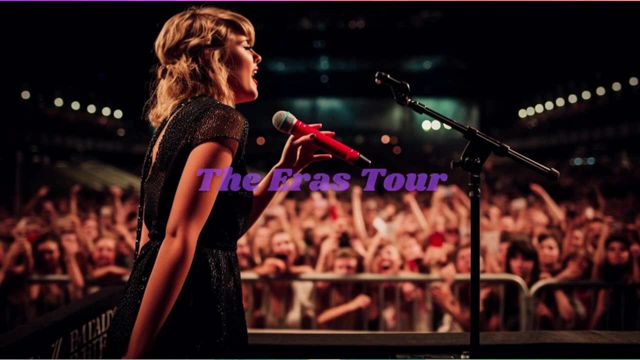 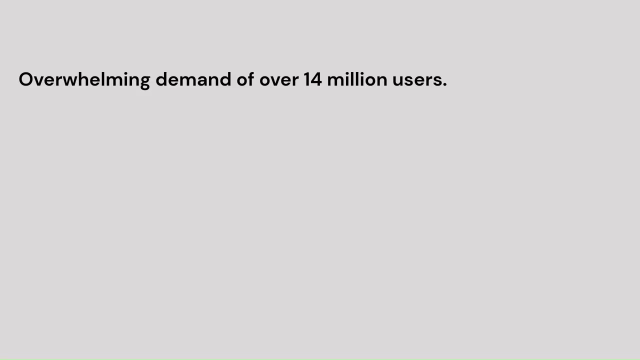 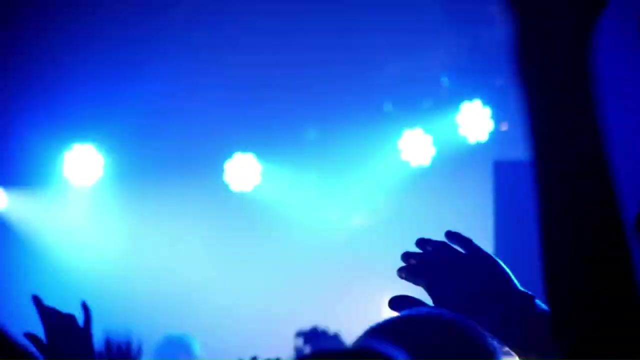 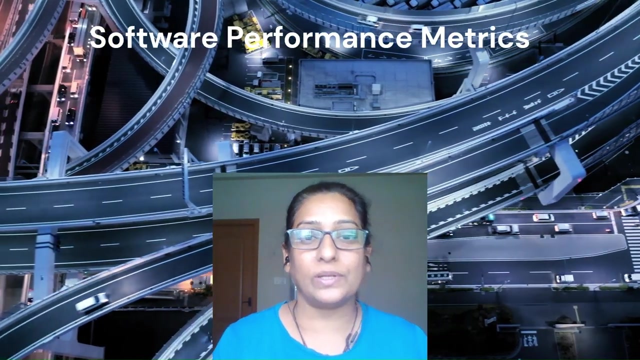 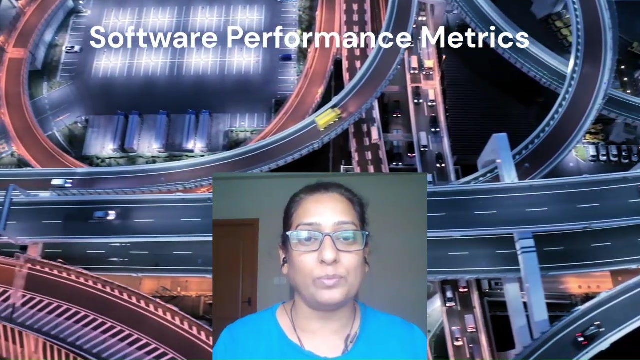 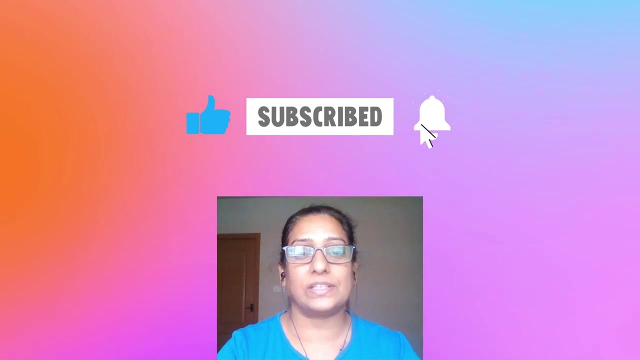 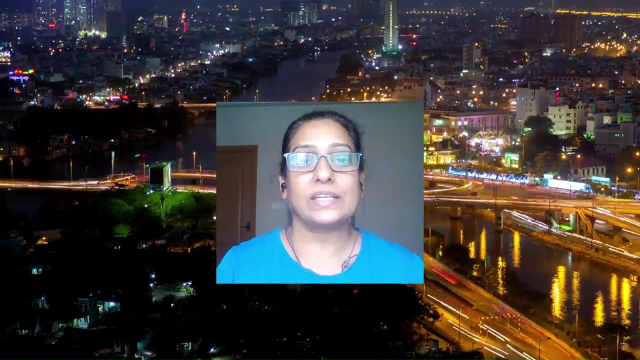 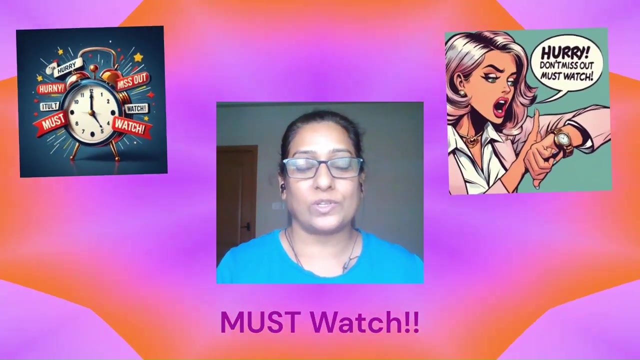 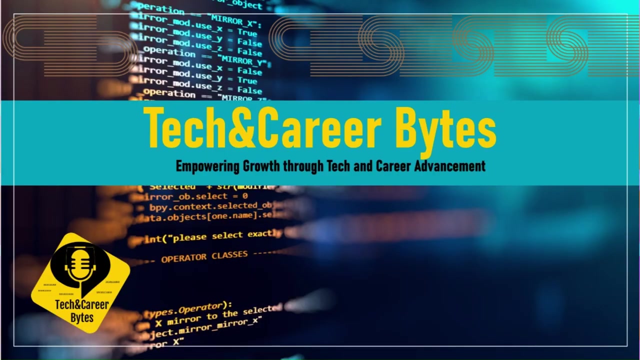 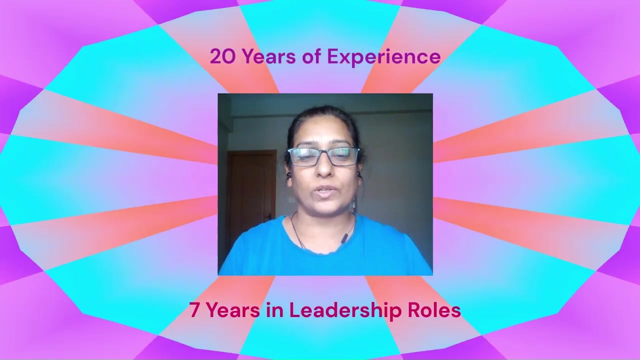 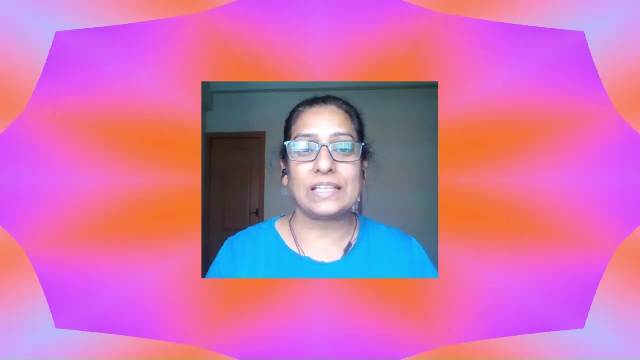 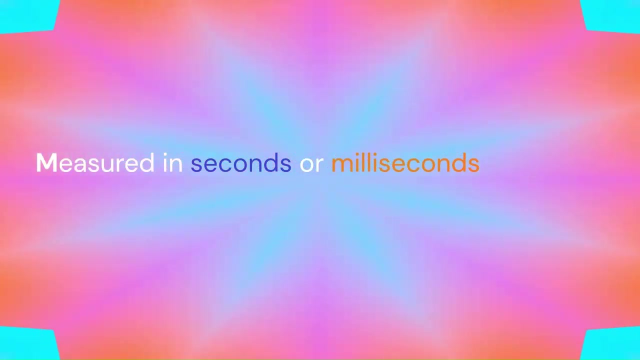 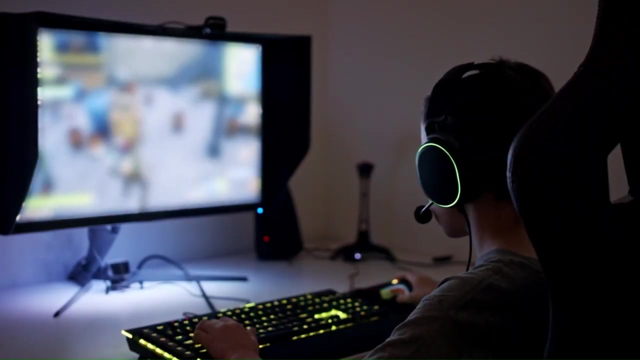 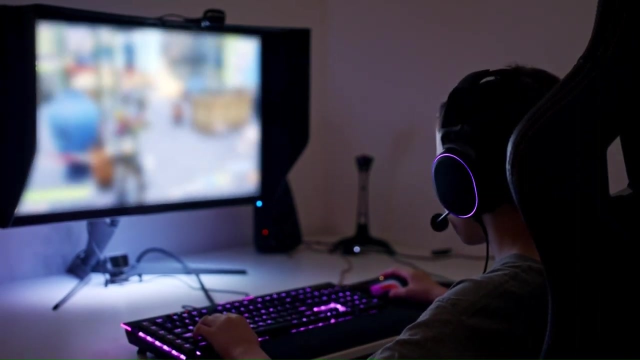 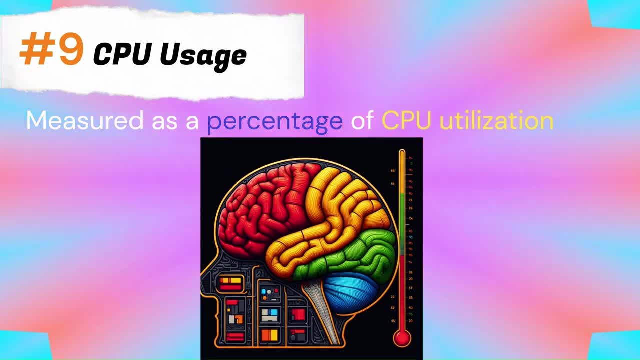 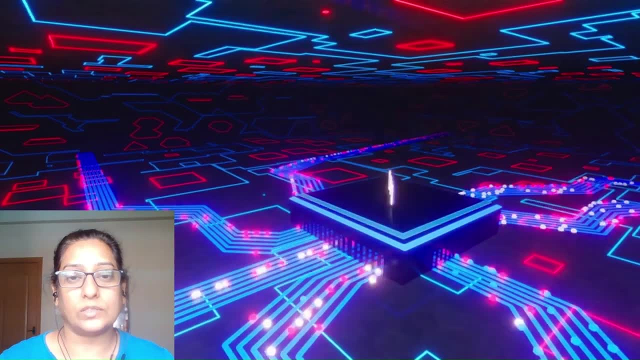 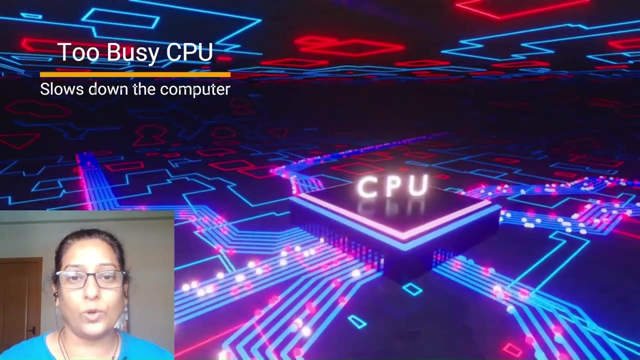 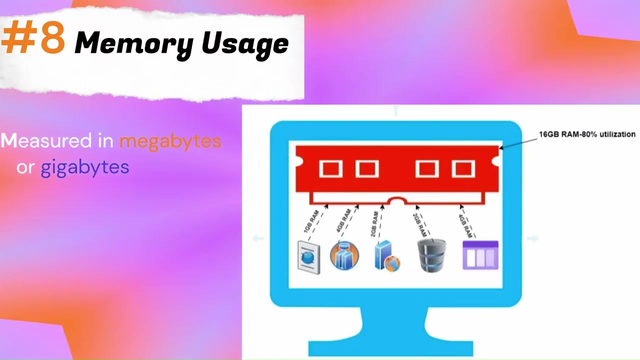 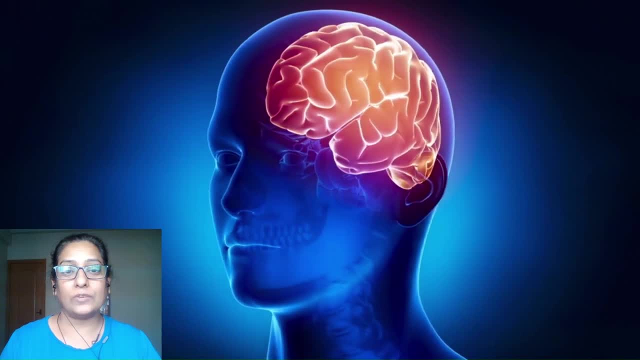 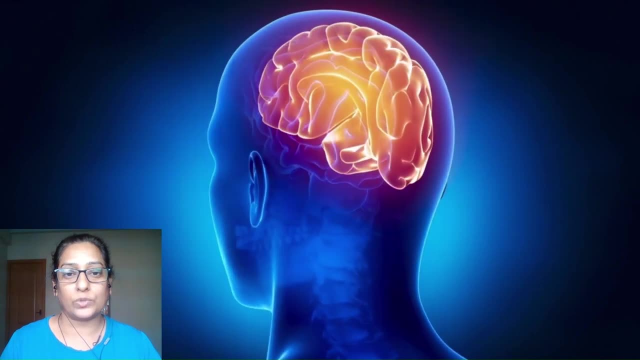 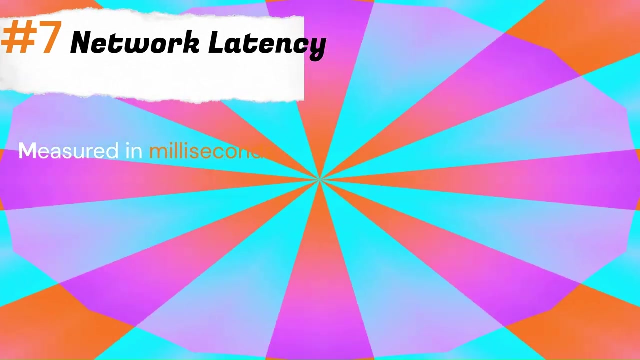 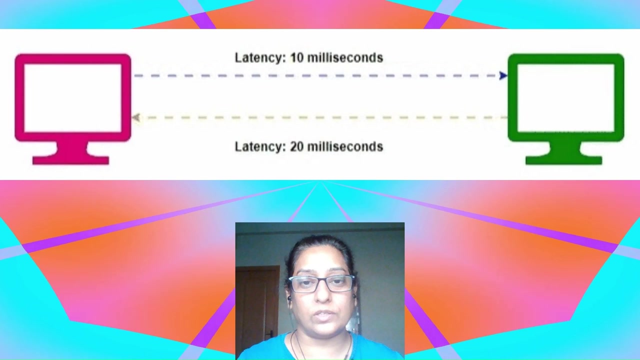 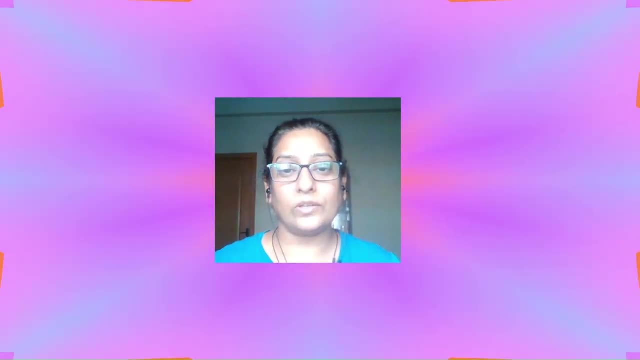 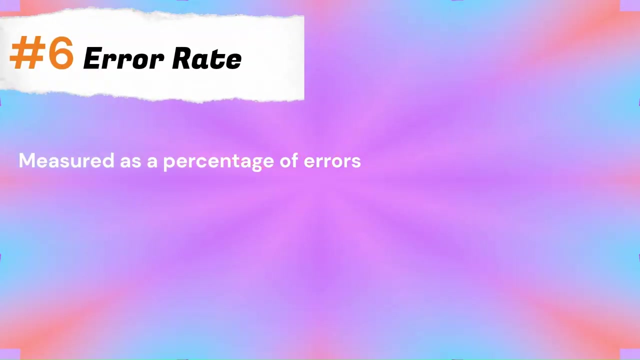 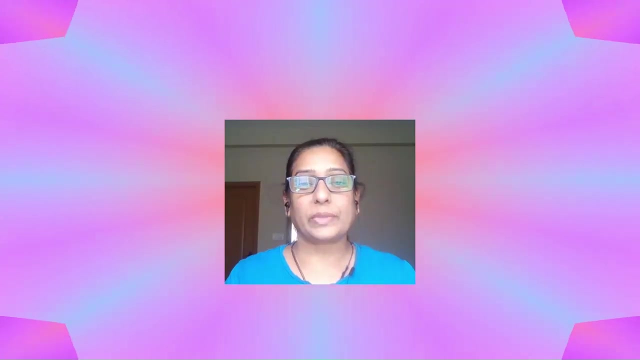 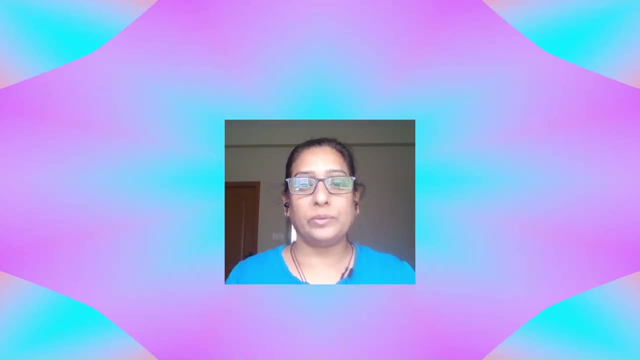 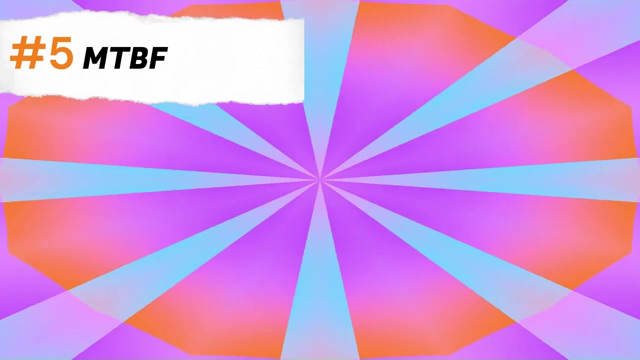 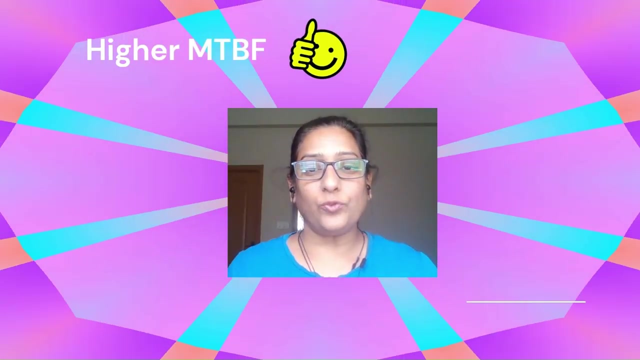 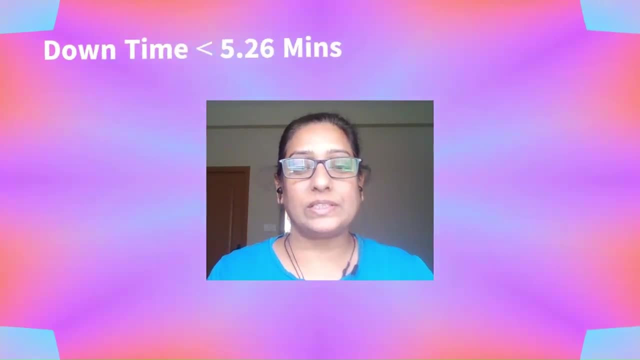 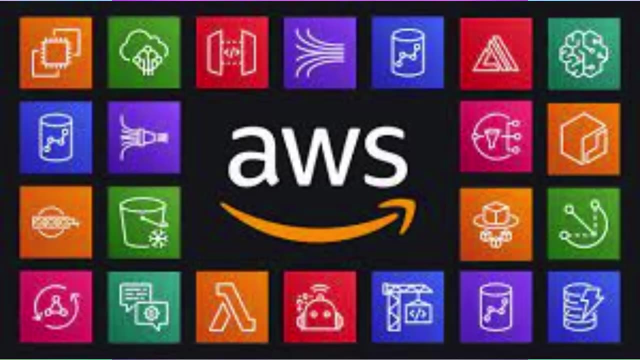 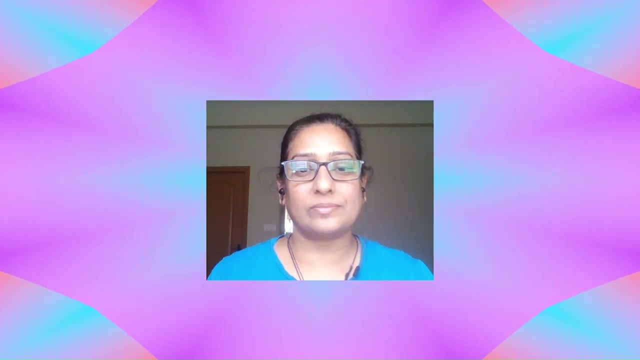 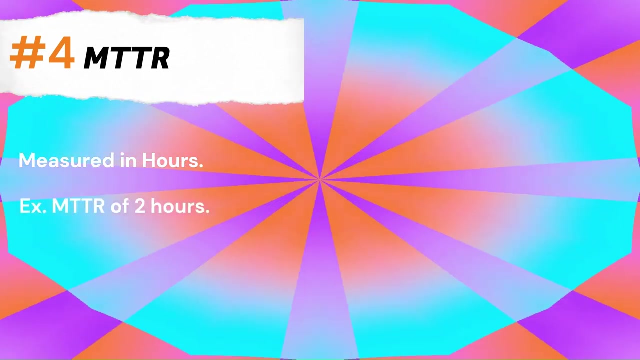 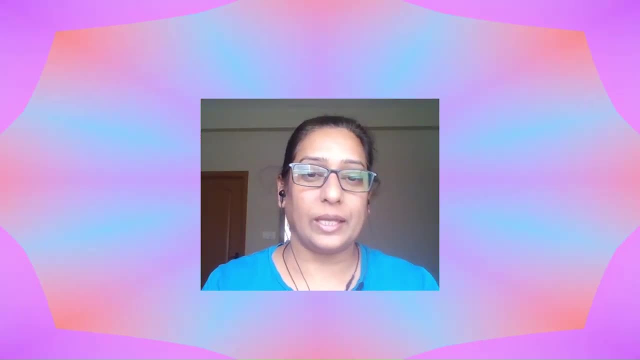 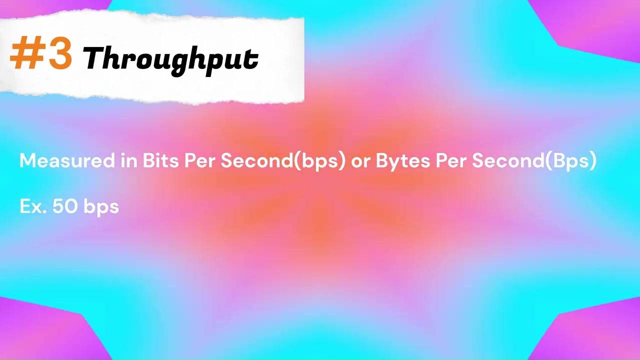 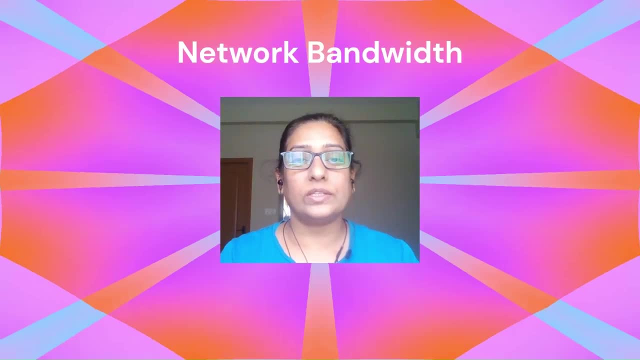 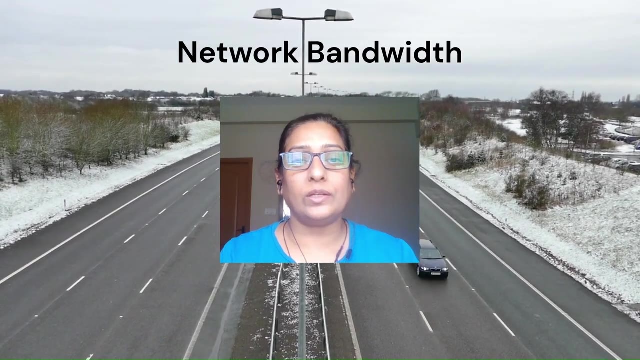 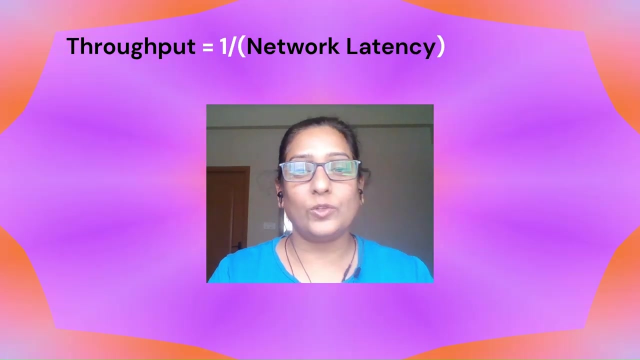 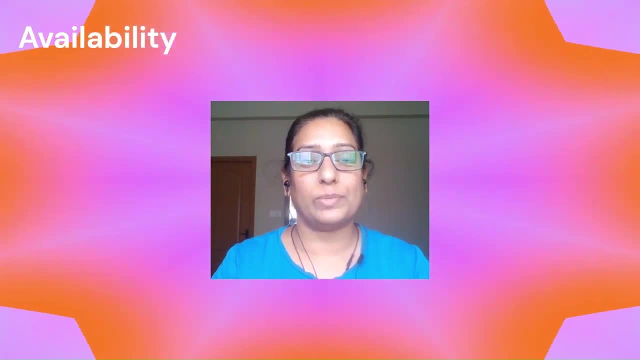 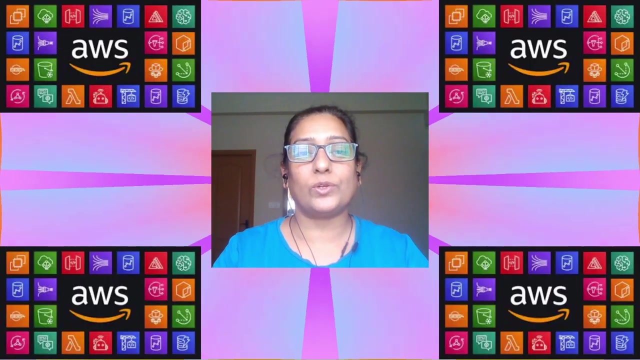 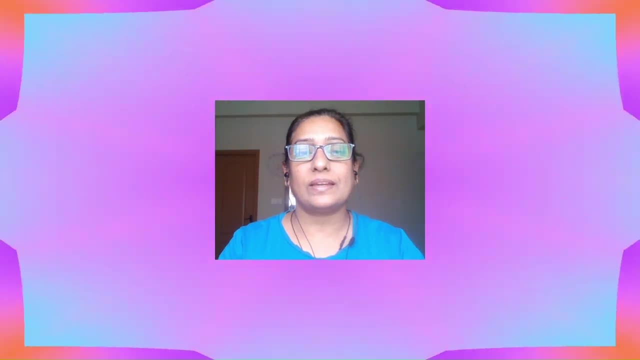 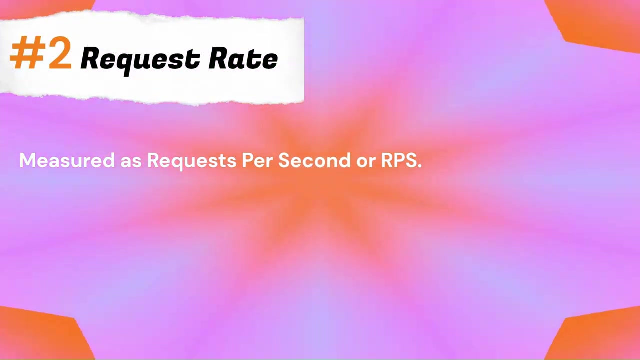 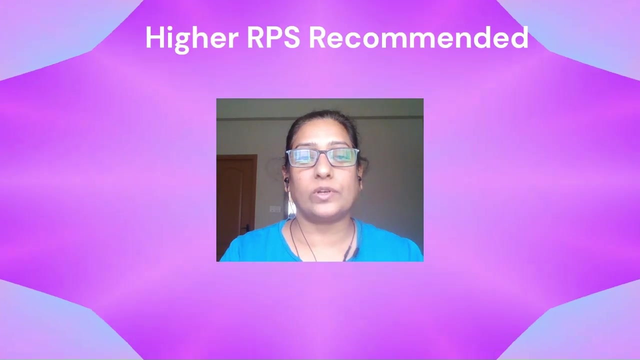 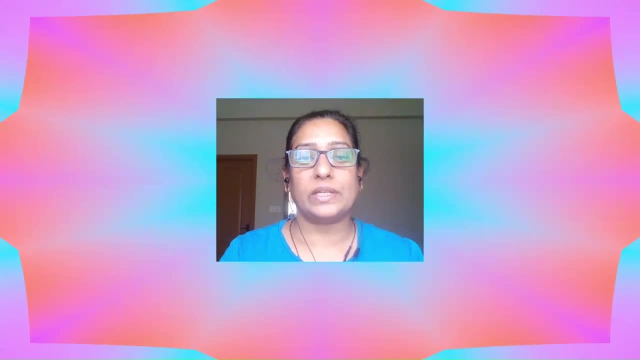 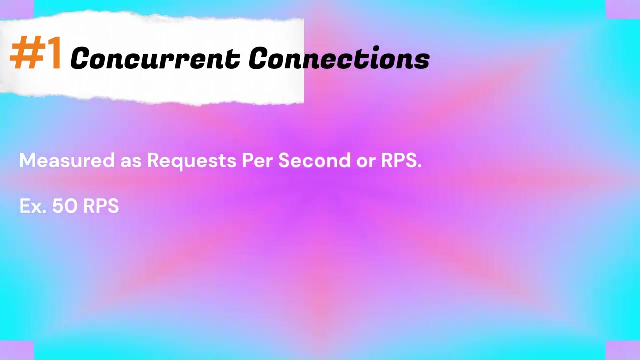 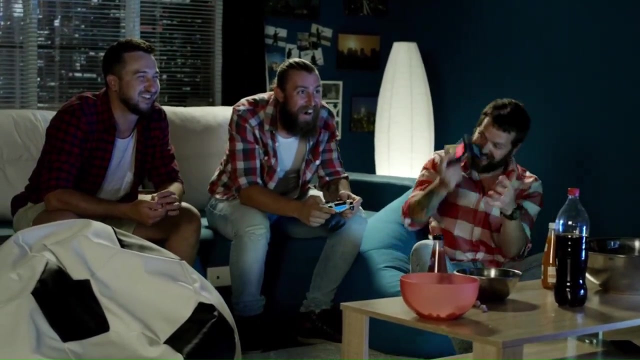 The more the RPS, the better it is, as your computer can do multiple things at once, And at number 1, we have the most important performance metric: Concurrent Connections. Concurrent Connections is like how many friends can play with you the game at the same time. 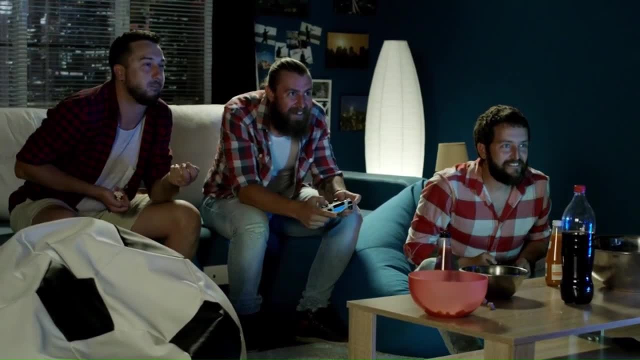 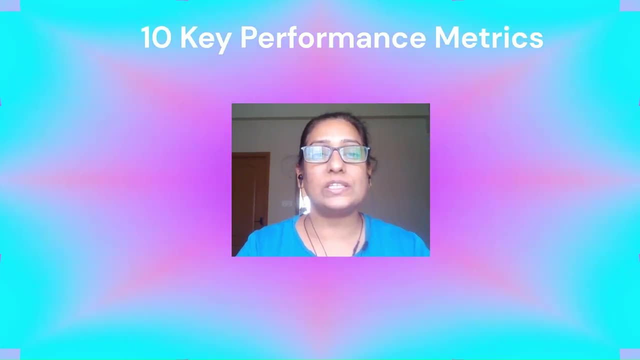 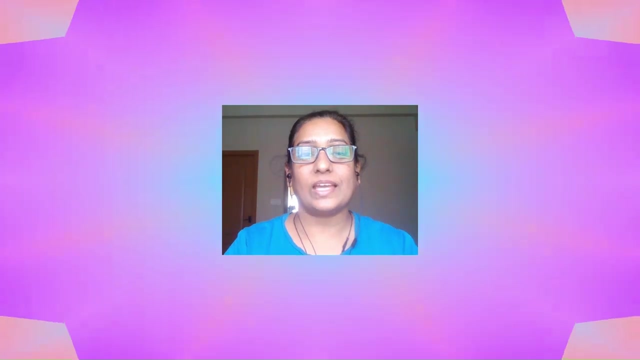 The more concurrent connections, the more friends can join you in your game. In today's video, we discussed 10 Key Performance Metrics. These performance metrics help a software engineer develop software that runs smoothly, is fast and has few problems as possible. If you like this video, then please do check out our other videos. 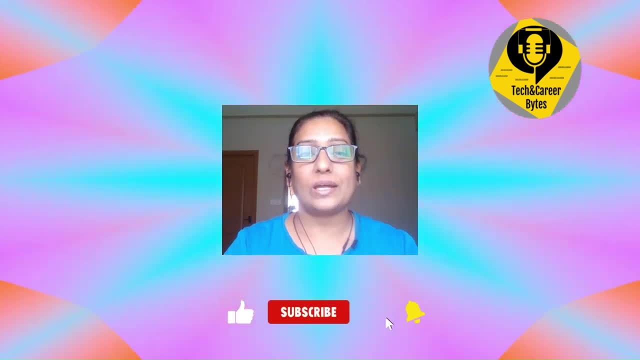 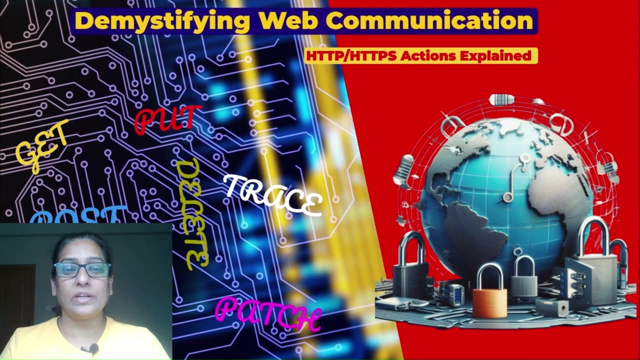 Don't forget to like, comment this video and subscribe to my channel. My name is Rupa and I thank you so much for watching this video. See you in the next video. Are you someone involved in web development, API design or working with web services? 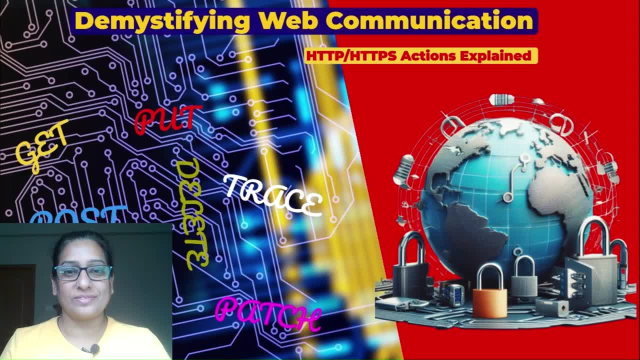 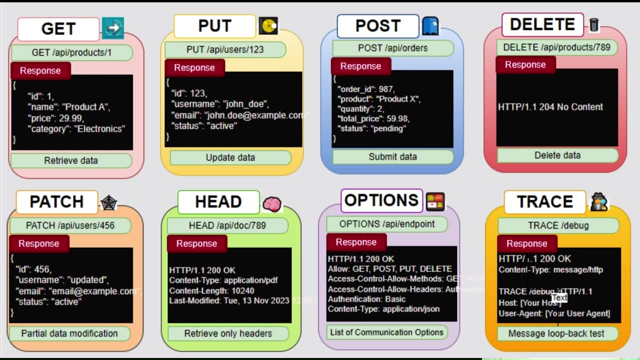 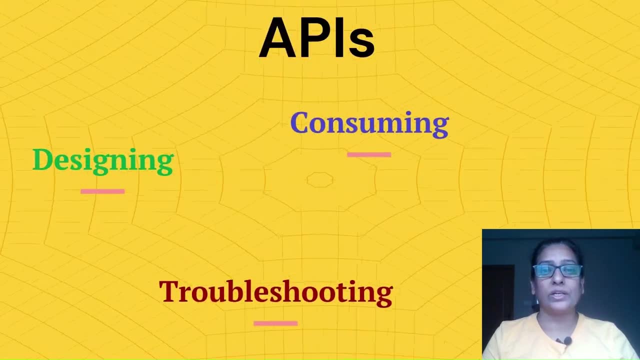 In that case, understanding HTTP actions or verbs is a must for you. In today's video, we will discuss top HTTP actions or verbs, along with examples. HTTP verbs form the foundation of communication in web development and are essential for designing, consuming and troubleshooting APIs and web services. 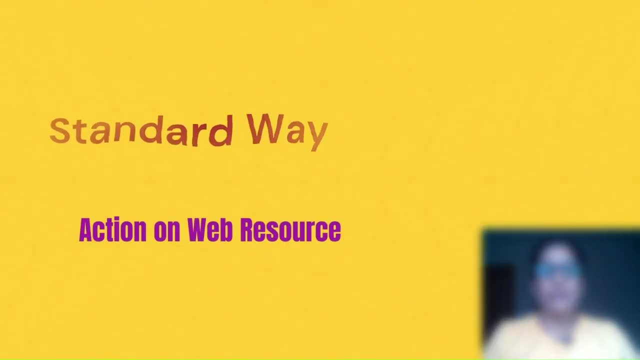 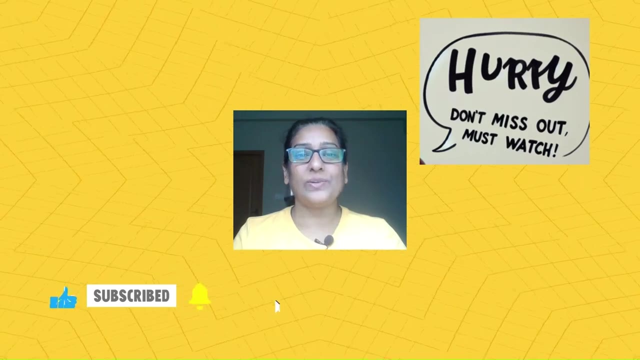 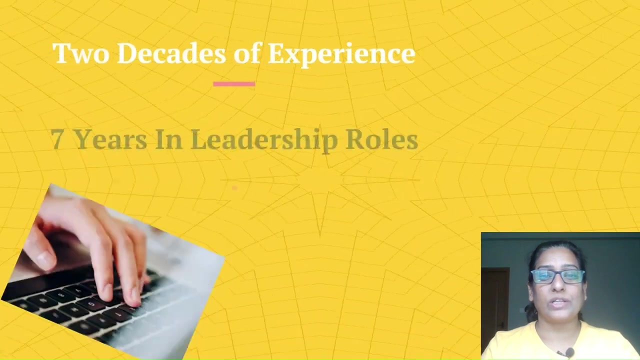 They provide a standard way to express the intended action on the resources over the web. This is really an interesting topic, So watch the video till the end. Hello everyone, welcome to Tech and Career Vibes. I am a software professional with more than 20 years of experience, including 7 years. 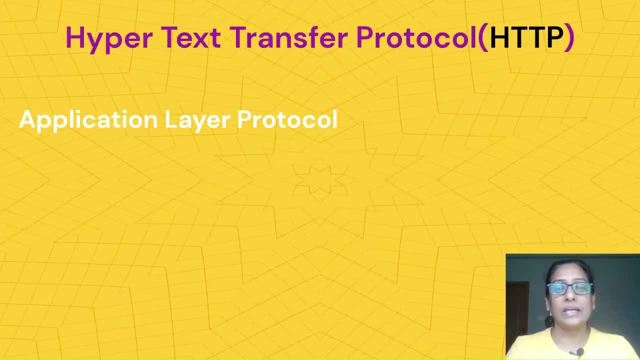 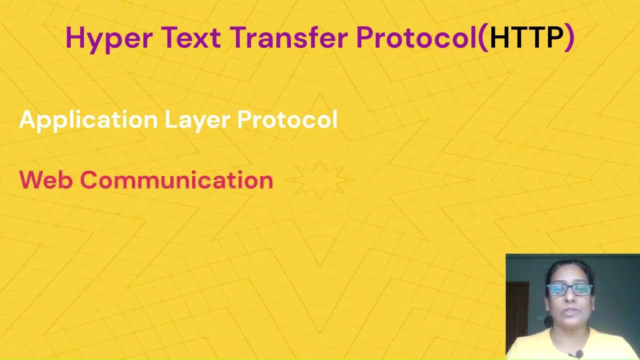 in leadership roles at a global product-based organization. HTTP stands for Hypertext Transfer Protocol. This is an application-led protocol that facilitates data transfer and communication on the world wide web. HTTP actions, also referred to as HTTP methods, are used to transfer data to the web. 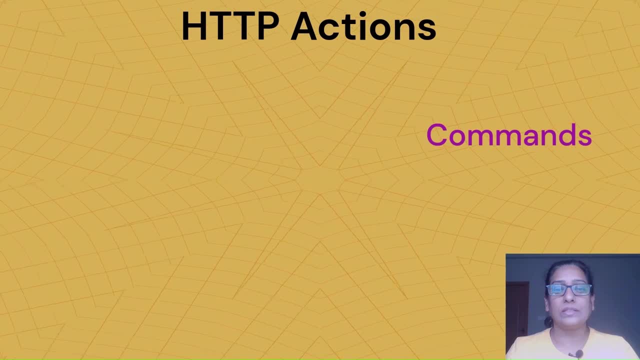 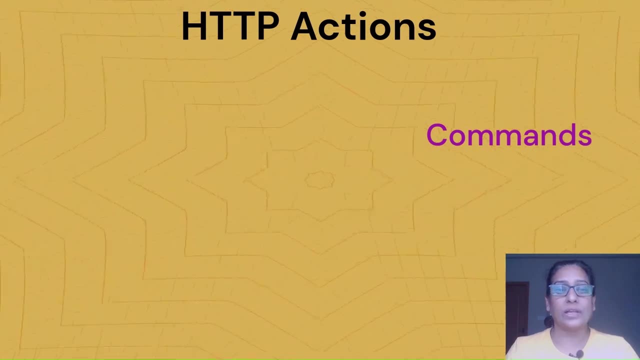 HTTP actions are used to transfer data to the web. This is a protocol that is used to transfer data to the web. HTTP verbs are the commands used in hypertext transfer protocol to specify the desired action on a resource. These actions define how the client and server should interact with the identified resource. 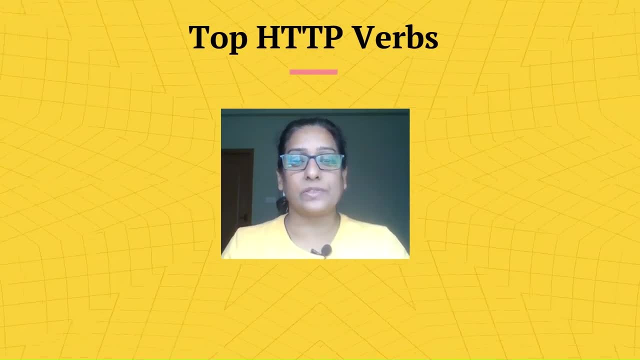 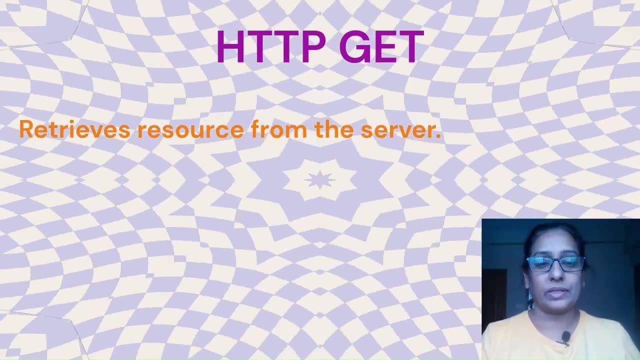 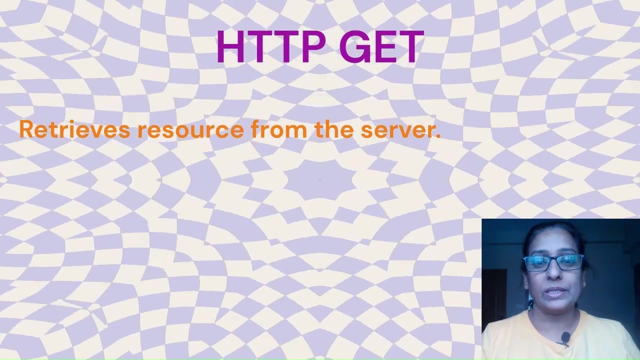 There are several HTTP verbs available. Let's discuss the frequently used, along with examples. Let's first discuss HTTP GET word. HTTP GET request retrieves a resource from the server. It is idempotent in nature, Which means multiple identical GETs. This means multiple identical GETs. 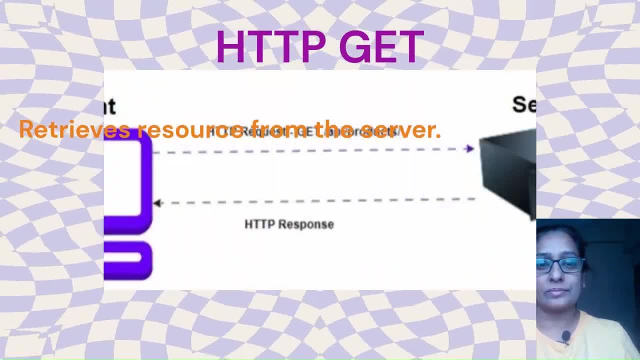 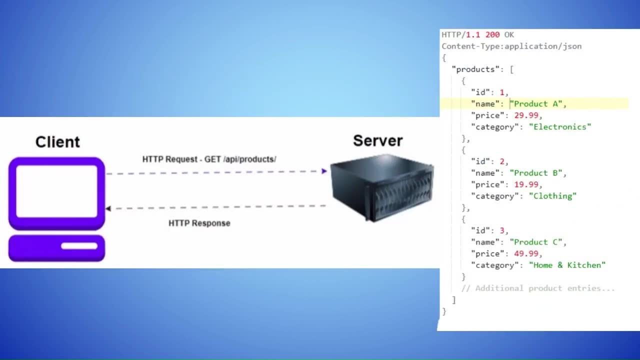 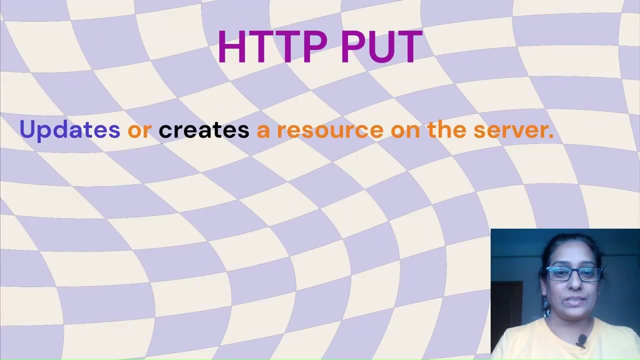 If one server receives an item with multiple identical GET requests returns the same result. For example, consider an HTTP GET request to retrieve the product's details. The response from the server will be a JSON object with an array of products. HTTP PUT updates or creates a resource on the server. 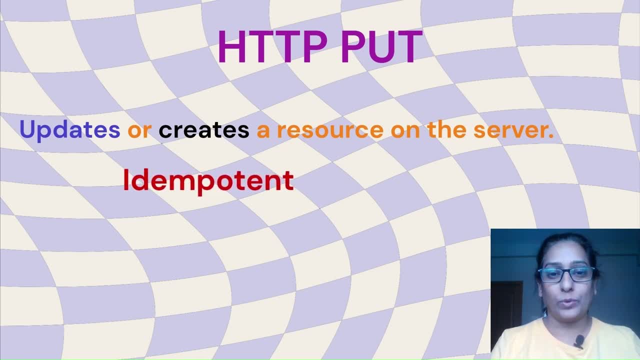 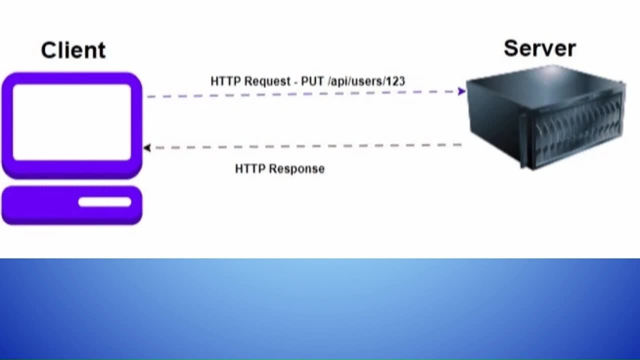 It is also idempotent with multiple identical PUT requests updating the same result. For example, consider the case of HTTP PUT. Consider this PUT request to update the user details for the user with ID 123.. If the user does not exist, then the PUT request creates that resource on the server. 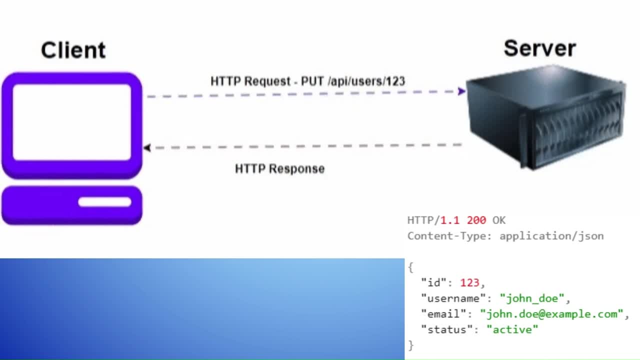 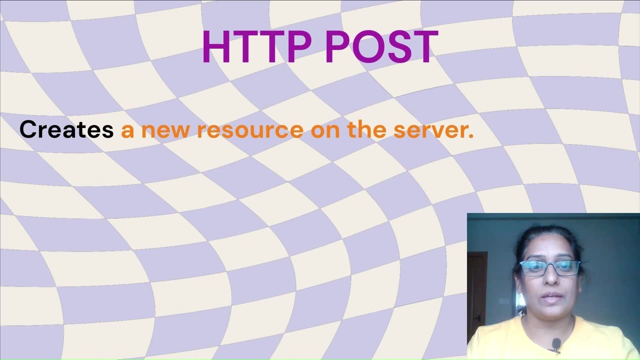 The response from the server will be a JSON object with updated user information. HTTP POST is used to create new resources on the server. It is not an idempotent action. That means if there are multiple identical POST requests then it will end up creating. 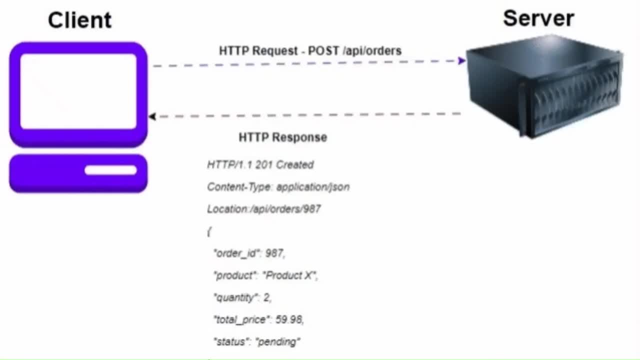 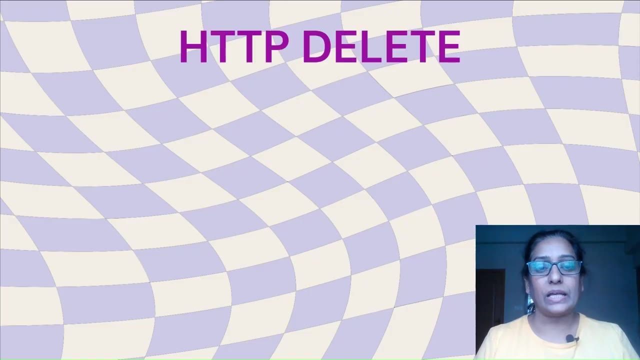 duplicate resources on the server. For example, consider this POST request to create an order on the server. The response from the server will be a JSON object with the details of the order created. Let's discuss HTTP DELETE. HTTP DELETE request deletes a resource on the server. It is an. 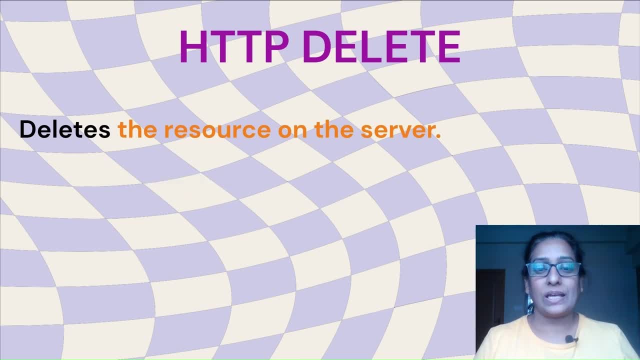 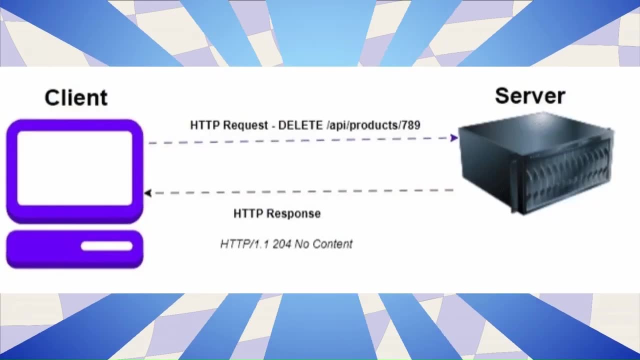 idempotent action. That means multiple identical requests impacts the same resource, That is, HTTP DELETE request deletes a resource on the server. It is an idempotent action. That means the same resource, if it exists, gets deleted. For example, consider the DELETE request to delete a product with ID 789.. 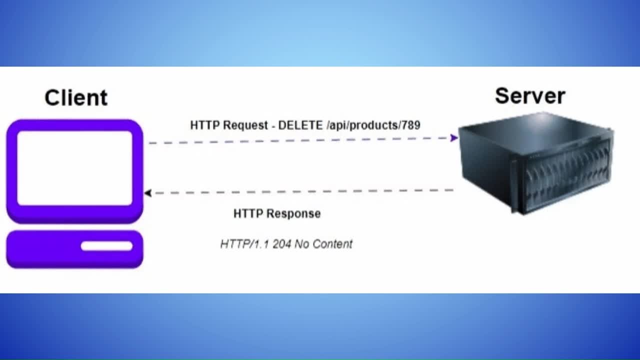 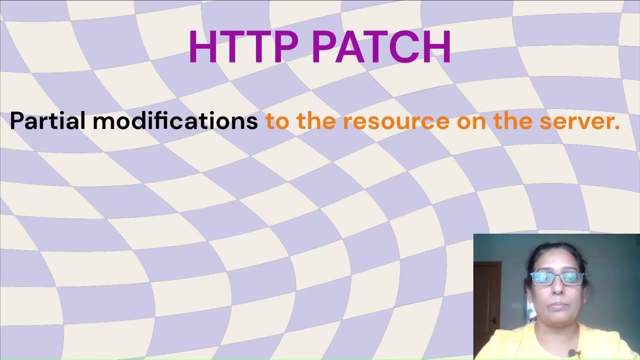 The response from the server will only indicate a success or failure and will not have any content in the response body. The PATCH request is used to apply partial modifications to the resource on the server. It is again an idempotent action. For example, consider the PATCH request to partially modify: 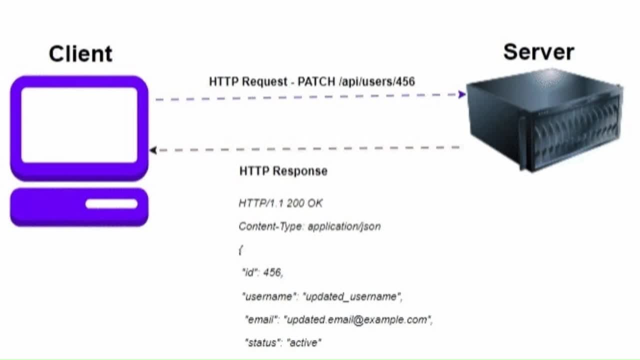 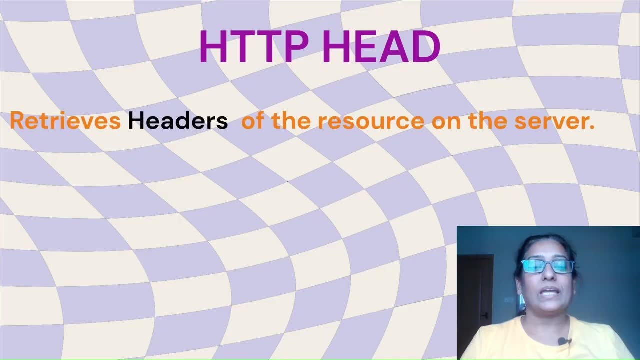 the user with the id 456.. The response from the server will be a JSON object with the updated user information. HTTP HEAD method is used to retrieve the headers of a resource without the actual response body. For example, consider the HTTP HEAD request to retrieve the headers of the document. 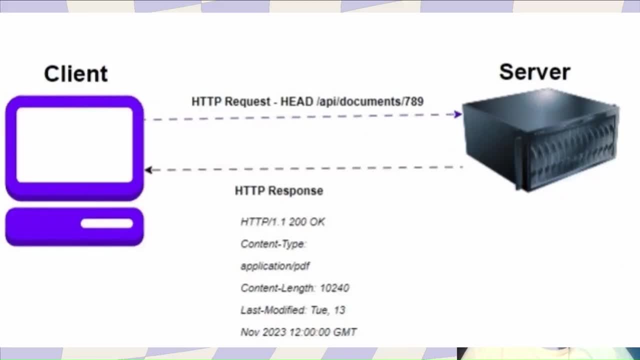 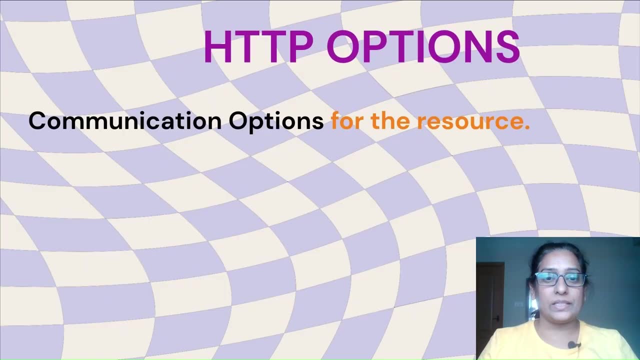 with id 789.. As the response will only have the headers information, the response from the server is typically minimal. The response from the server will only have the headers information. The response from the server is typically minimal. The HTTP options describes the communication options for the specified resource. 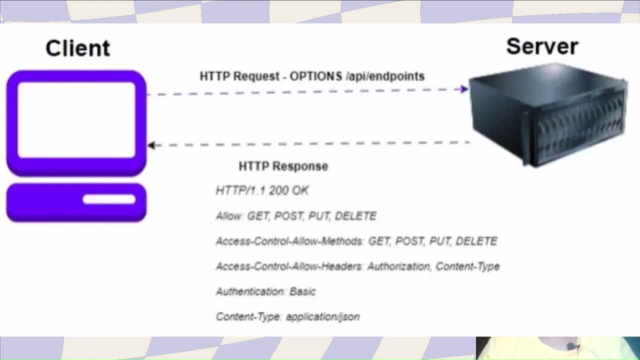 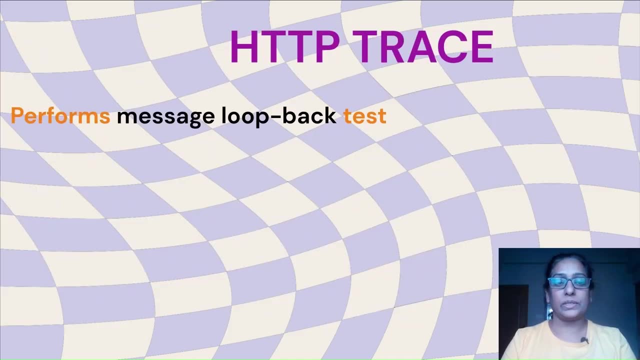 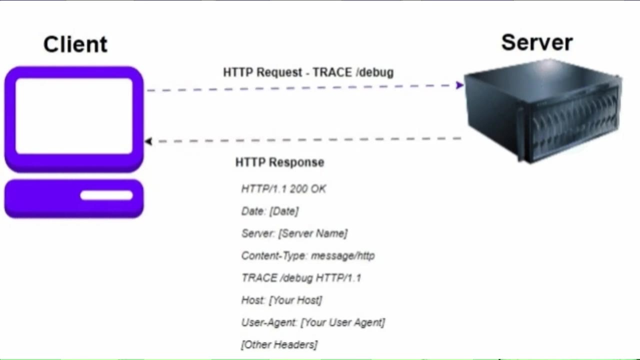 The response from the server typically includes information on allowed methods, headers and other potential capabilities for the specified resource. The HTTP TRACE method is used to perform a message loopback test. It is typically used for diagnostic purposes, allowing the client to see the modifications done by the intermediate servers. 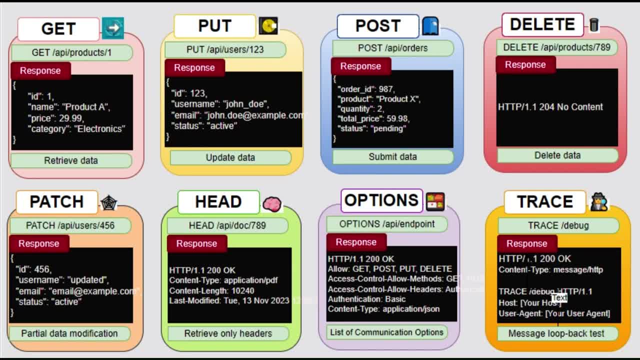 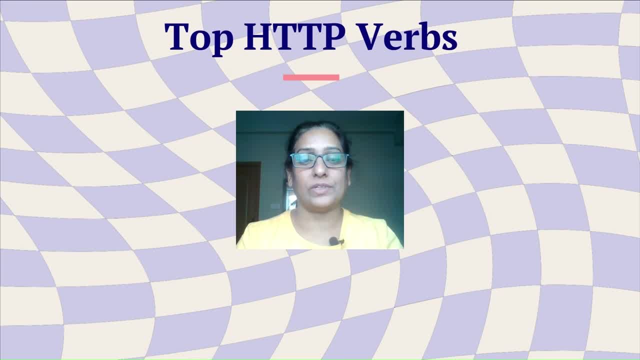 In today's video we discussed frequently used HTTP actions or HTTP works. I hope you learned something useful today. If you liked this video, then do check out our other videos Also. don't forget to like, comment this video and subscribe to my channel. 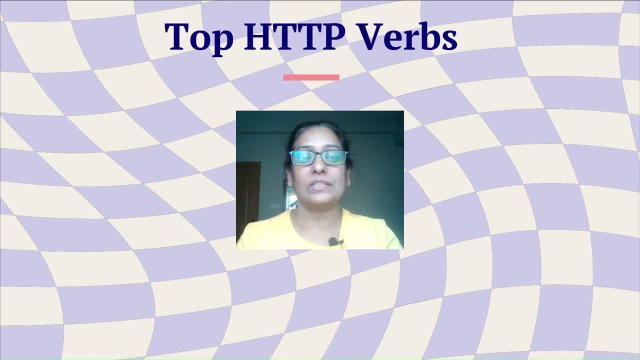 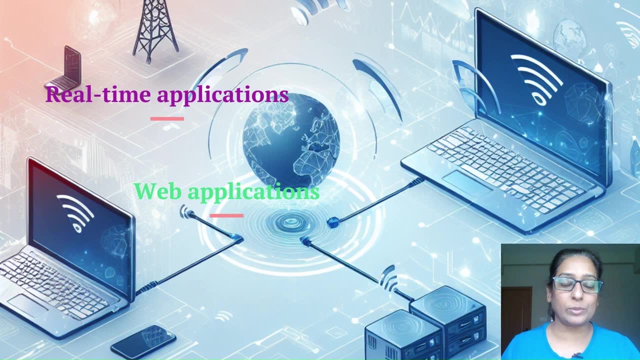 My name is Ruf garn and I thank you so much for watching this video. See you in the next Video. Understanding data pitch patterns is crucial for developers who are involved in building real-time applications, web applications or systems with dynamic data requirements. It helps the developers make informed decision about. 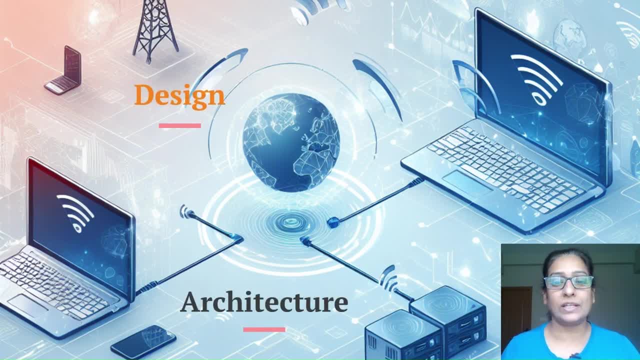 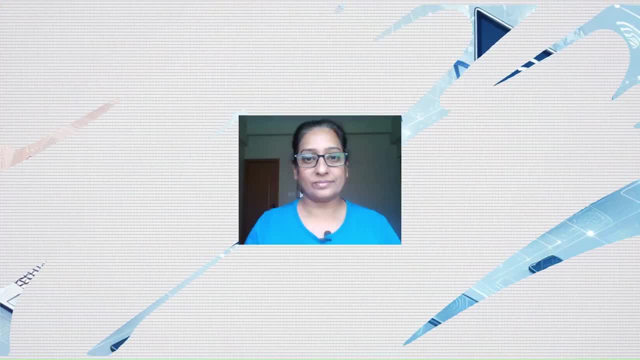 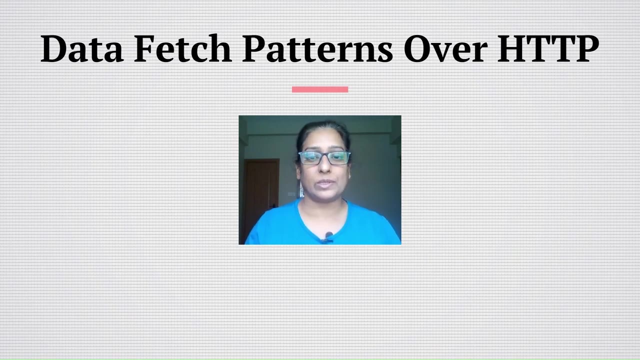 the design and architecture of the systems, and we all know that a well-architected system contributes immensely to the user satisfaction and success of the application. data communication between a client and a server can occur through various protocols and mechanisms, each serving its specific purpose. if you remember, in our previous video, we discussed 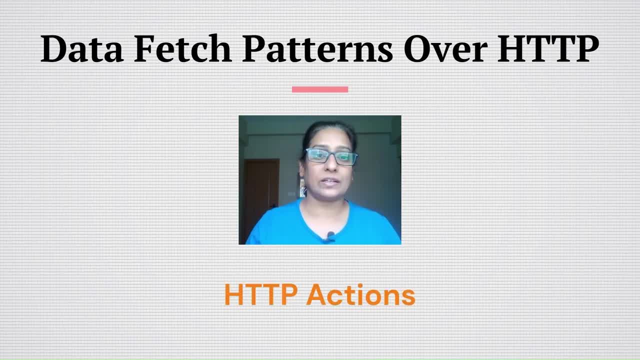 various http actions used for web communication and data transfer. if you have not yet watched that video, i strongly recommend you watch that video now. and in today's video we will focus on data communication or data fetch mechanisms between a client and server using http protocol. so let's dive in. hello everyone. welcome to tech and career files. i'm a software professional with 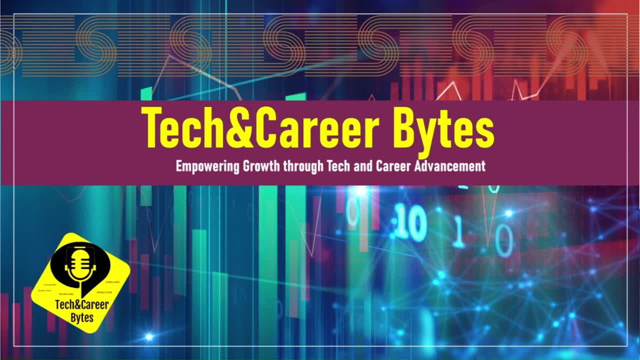 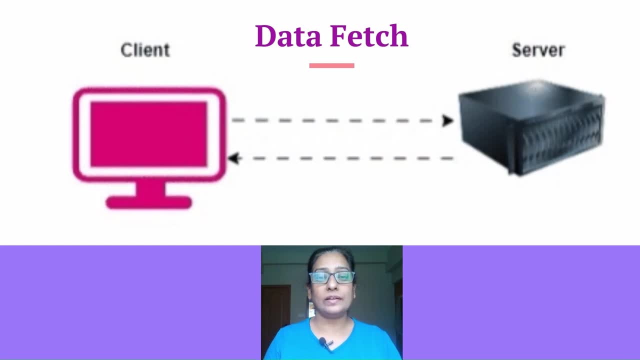 more than 20 years of experience, including seven years in leadership roles at a global product based organization. data fetch, as you rightly guessed, is a process of retrieving a data or information from a source, typically a server or a database, and then bringing it to an application or client for further processing. 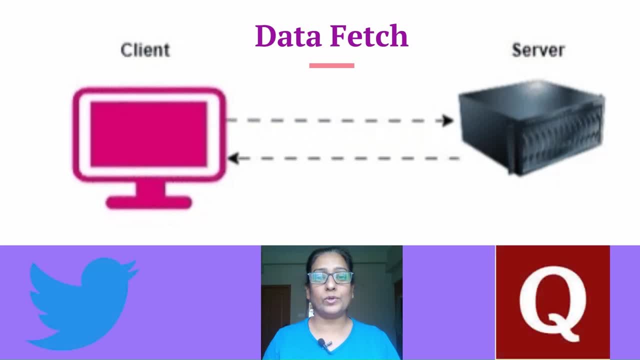 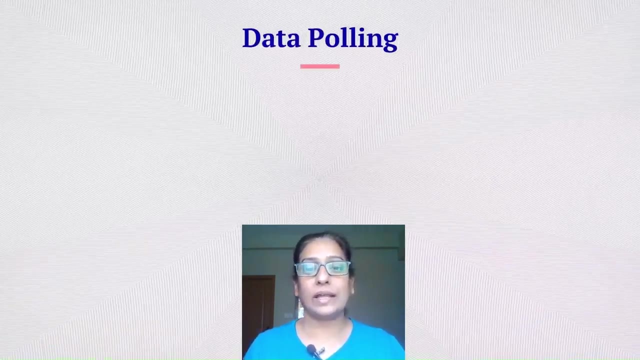 or display in applications with high read throughput such as quora or twitter. with millions of data fetch requests every second, the need for an effective communication structure becomes very crucial. let's discuss our first data fetch pattern: data polling. with the data polling, the client repeatedly requests the server for updates or new information. there are two techniques in data. 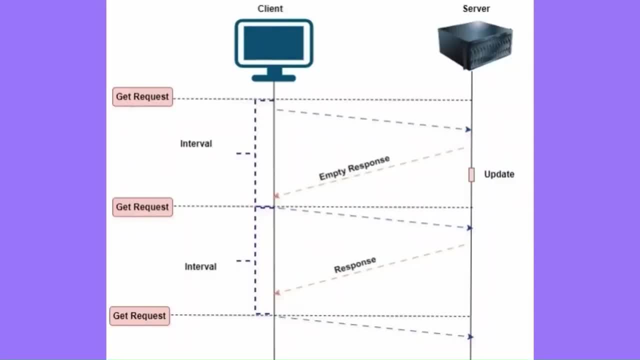 polling: long polling and short polling. in short polling, the client sends a request to the server at predefined intervals, usually less than a minute, asking for updates of the latest information. the server receives the request and processes it. if there is new information, the server responds to the client with the updated data. 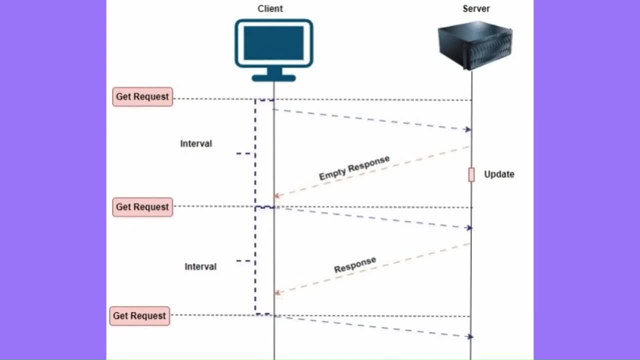 and if there is no new data, the server may respond with an empty message. the client repeats this process at regular intervals, regardless of whether there is new data or not. as you can see in the figure, even though the update is available, the client requests only at the specified interval. 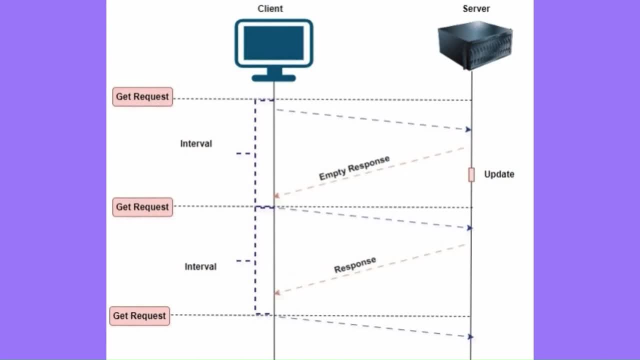 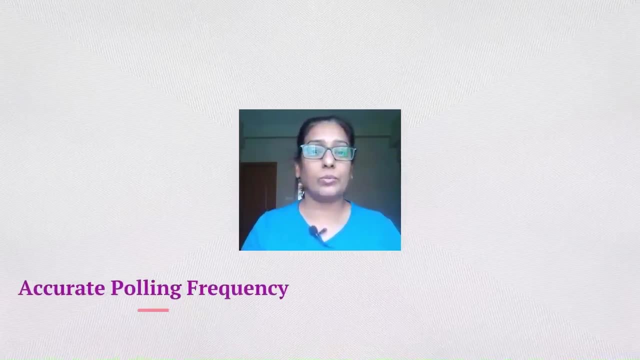 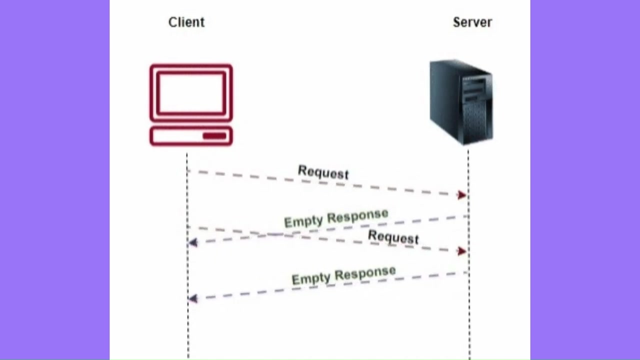 thereby delaying the data retrieval. short polling works well when the information availability time frame is known well in advance, so that the polling frequency can be set accurately. if the polling frequency is not accurate, then it has drawbacks like unnecessary request to the server when the updates are not. 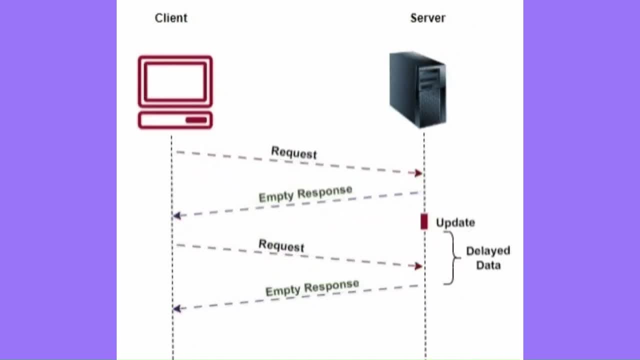 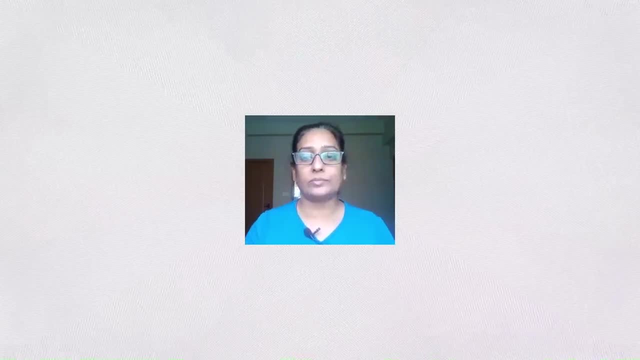 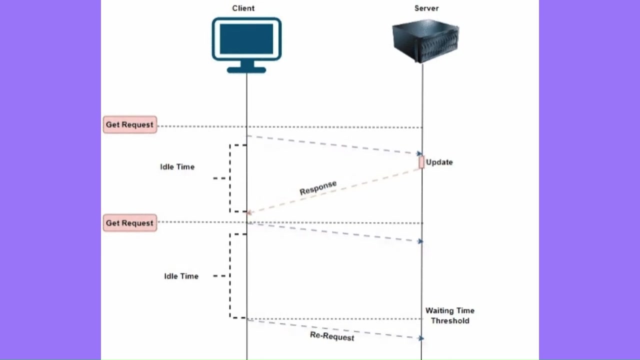 available or delay the data retrieval when the updates are available at the server but the client has not requested. let's now discuss our second data pooling technique: long point. long polling. similar to short polling, but the client stays connected and waits for a response from the server until new updates are available or a time out offers. this approach minimizes idle. 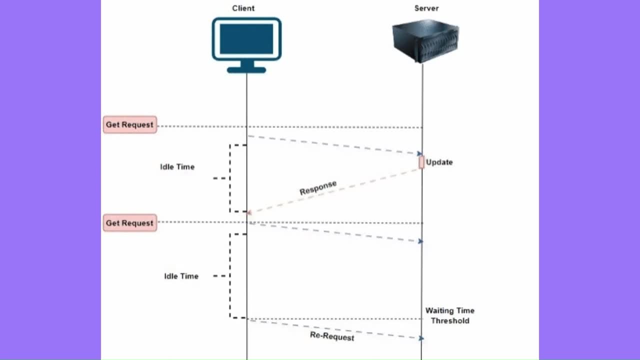 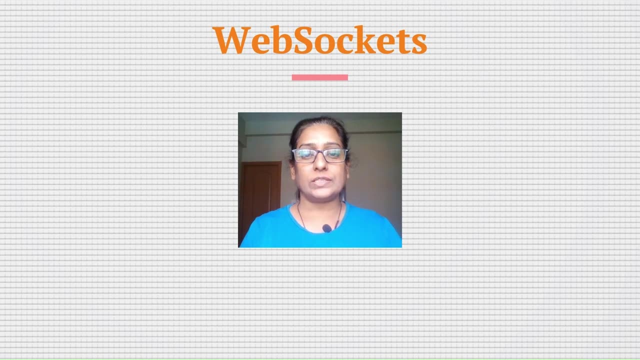 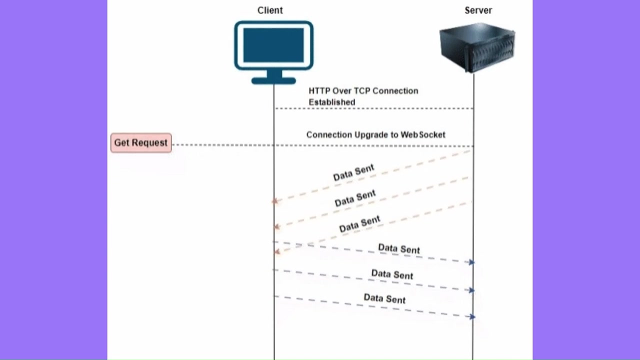 time, but it introduces connection management challenges. clients may need to reconnect multiple times after time outs to get new data. using web sockets is one another view of data communication between a client and a server. websocket is a persistent paul duplix communication protocol landing on a single tcp connection. the process of establishing a websocket- 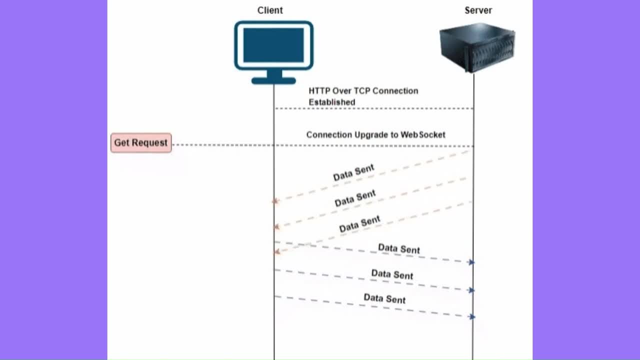 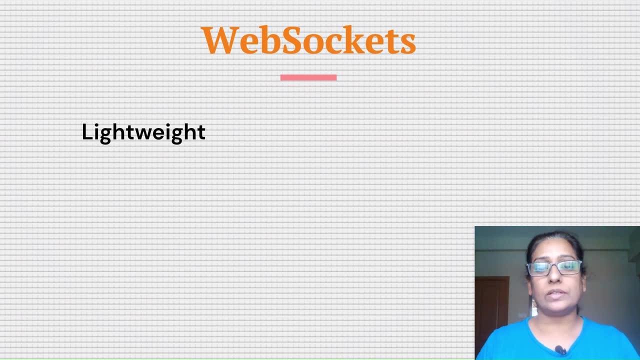 often involves an initial HTTP handshake over TCP, and then the connection is upgraded to the WebSocket protocol. WebSocket frames are more lightweight than the traditional HTTP requests and they support full duplex communication, meaning both the client and the server can send messages to each other. 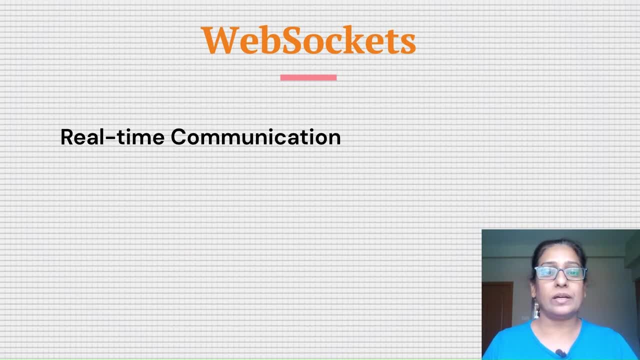 WebSockets addresses the limitations of data pooling techniques, enabling real-time communication between the client and the server without the need for continuous pooling. They are suitable for scenarios requiring low latency and high resource utilization. Let's compare the three approaches we just discussed. 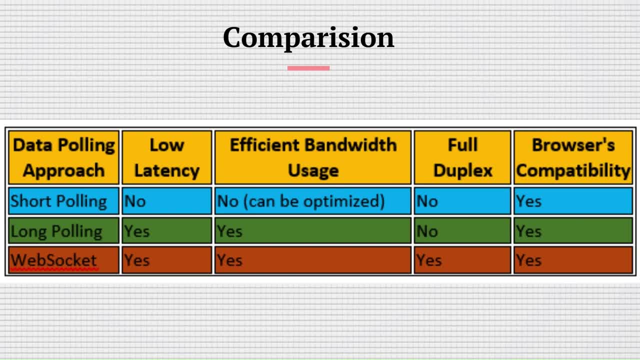 You can pause the video and think if this comparison makes sense based on what we learned so far. If there is anything you would like to discuss further, leave your thoughts in the comment section and I will get back to you In today's video. 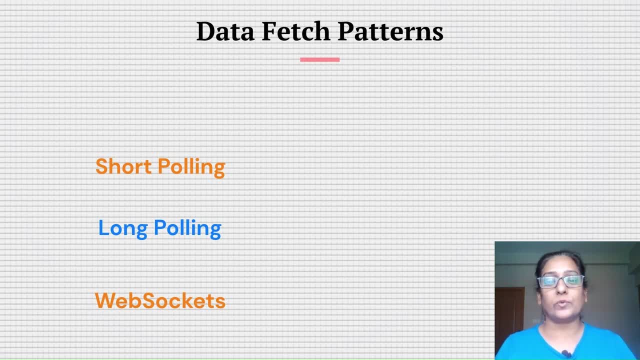 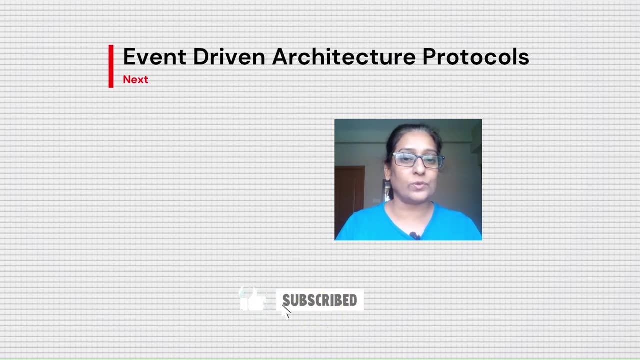 we discussed data fetch or data retrieval patterns based on HTTP request and response. If you like this video, do check out our other videos. Welcome to the WebSocket. Also, don't forget to comment this video and subscribe to my channel. My name is Rupa. 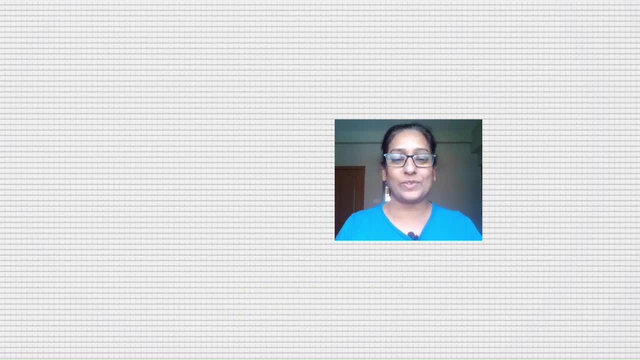 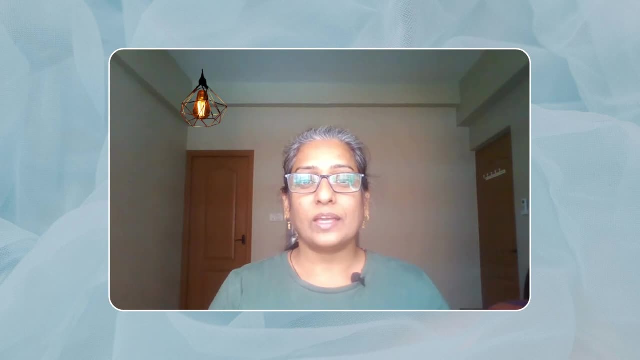 and I thank you so much for watching this video. See you in the next video. So how is it going so far? Lot of learning, isn't it? If you have any suggestions or questions, share it in the comment section. I will get back to you as soon as I can. 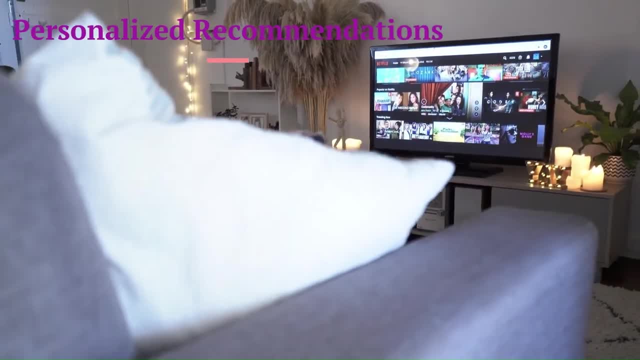 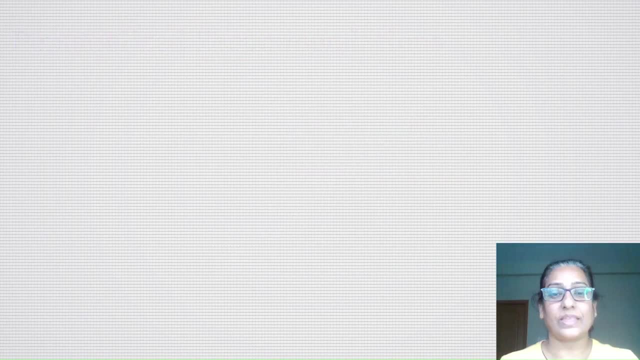 As you browse through your favorite Netflix shows, you might have noticed the curated recommendations. Have you ever wondered how Netflix shares these personalized recommendations to you? Let's find out. In today's video, we will discuss essential protocols like webhooks, server-sent events, WebSockets and WebSub. 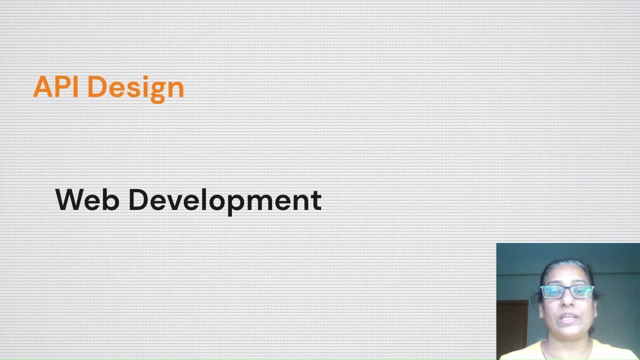 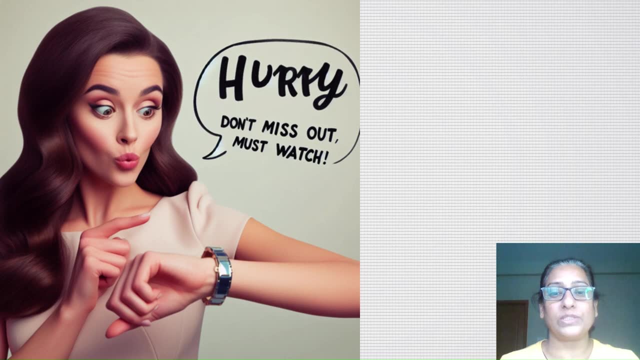 widely used in event-driven architecture. If you are someone involved in API or web development, then understanding event-driven architecture and these protocols is very crucial, So don't miss out on valuable insights. Watch this video till the end, Hello everyone. 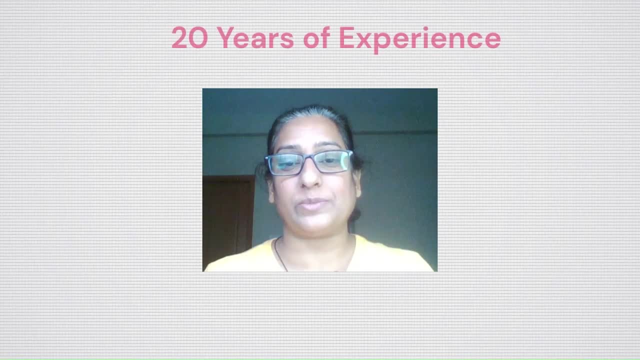 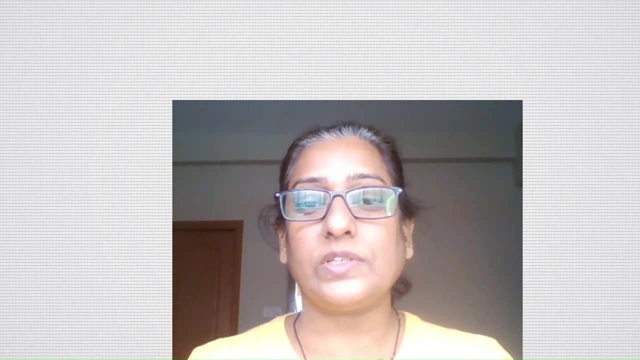 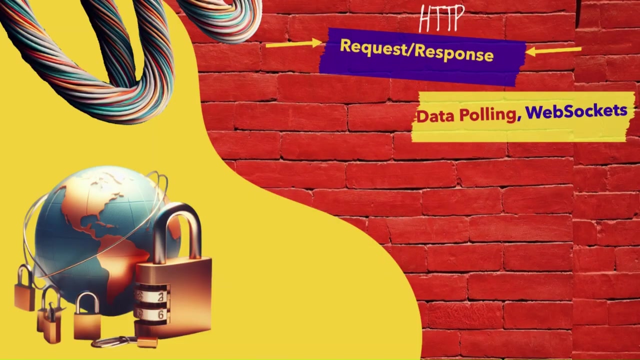 Welcome to Tech and Career Bites. I'm a software professional with more than 20 years of experience, including seven years in leadership roles at a global product-based organization. HTTP request-response-based data-pitch mechanisms involve continuous requests or open connections, as seen in short-pooling and long-pooling respectively. 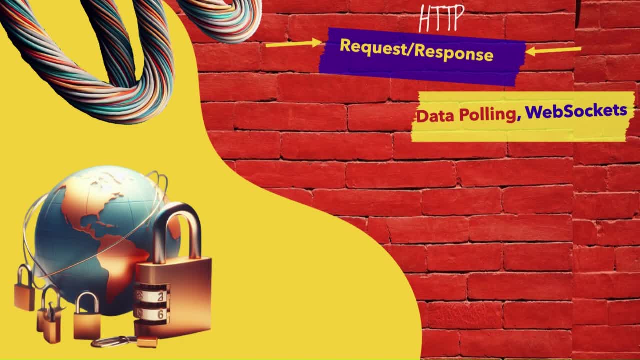 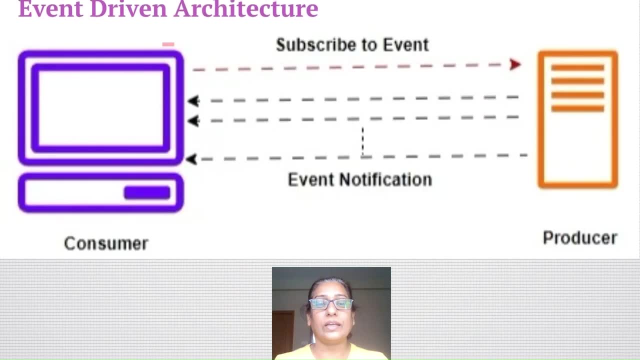 We have discussed these mechanisms at length in our previous video. If not watched, then I suggest you watch that video. The link is available in the description box. also, Event-driven architecture takes a different approach by allowing systems to react to events as they occur. 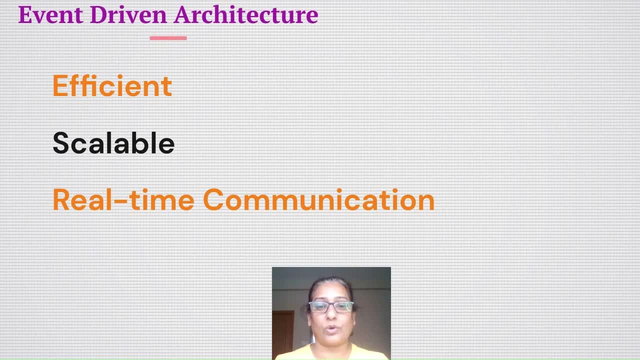 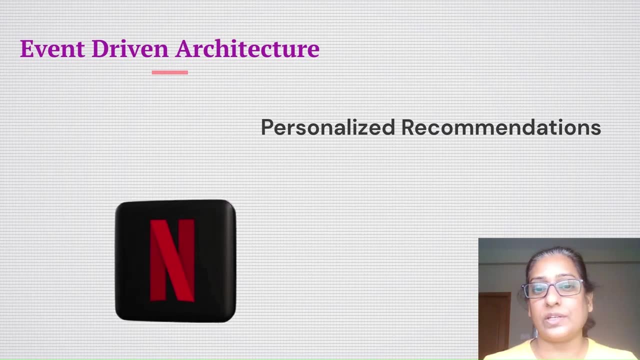 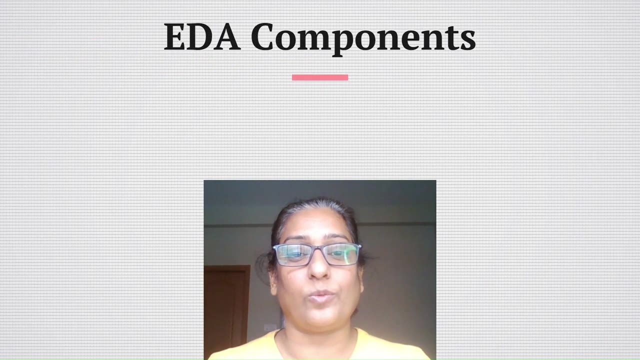 This promotes a more efficient, scalable and real-time communication model. Netflix utilizes an event-driven approach for managing its recommendation system. Events such as user interactions and viewing history trigger recommendations in real time. Event-driven architecture comprises several key components that collaborate to create a responsive and event-driven system. 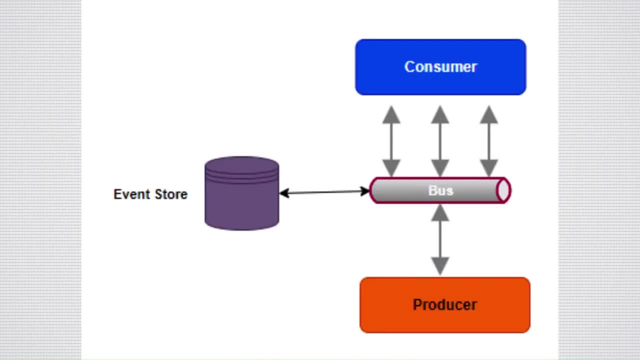 These components include event producers, event consumers, eventbuzz and eventboss. These components include event producers, event consumers, eventboss and eventboss. These components include event producers, event consumers, eventboss and eventboss. Event Producers are the entities responsible for generating events based on changes or 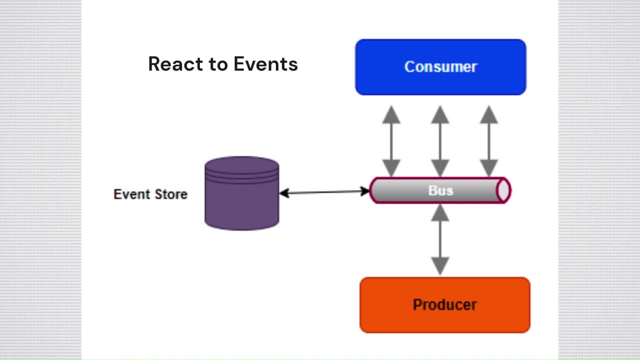 triggers within the system. Event Consumers are the components designed to react to specific events by initiating predefined actions or processes. Event Bus is the communication channel that facilitates the flow of events between producers and consumers. It acts as a mediator, ensuring seamless event distribution. 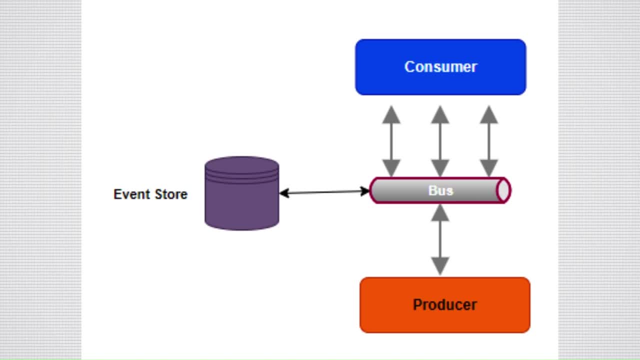 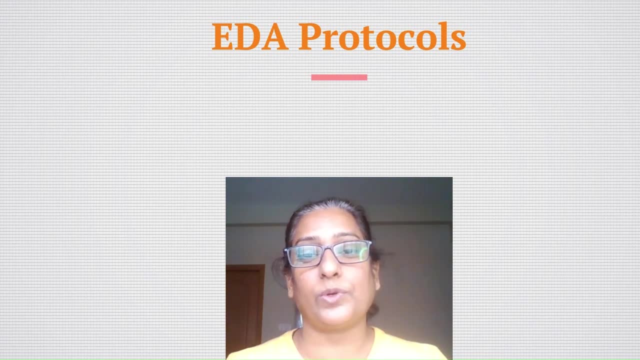 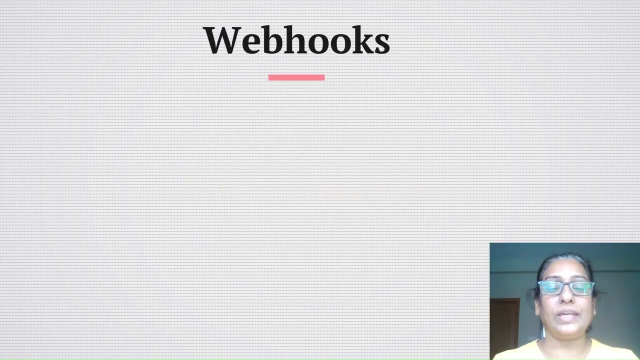 Event Store is a repository that records and manages the historical log of events, providing a valuable resource for auditing, debugging and system analysis. Let's discuss some widely used protocols in event-driven architecture. First Protocol – Webhooks. Webhook is a one-way event-driven communication. 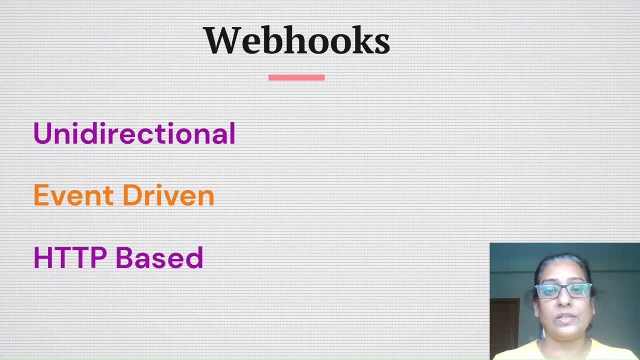 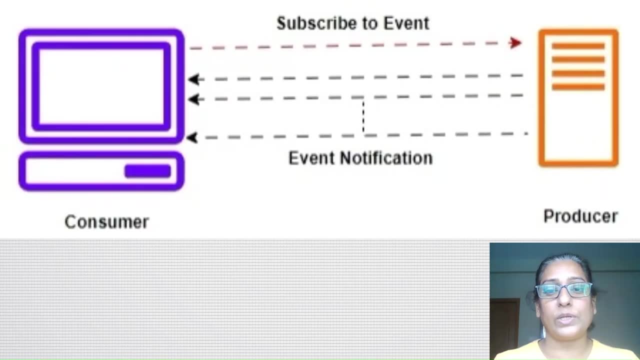 protocol based on HTTP. It enables applications to send real-time information when a particular event gets triggered In a webhook protocol. the consumer first subscribes to a particular topic with the producer. After the subscription, the producer automatically notifies the user that the event has been. 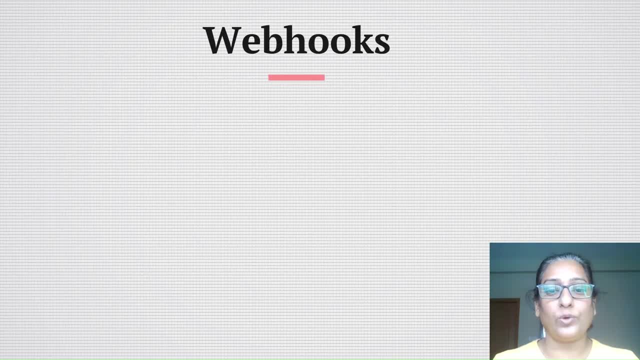 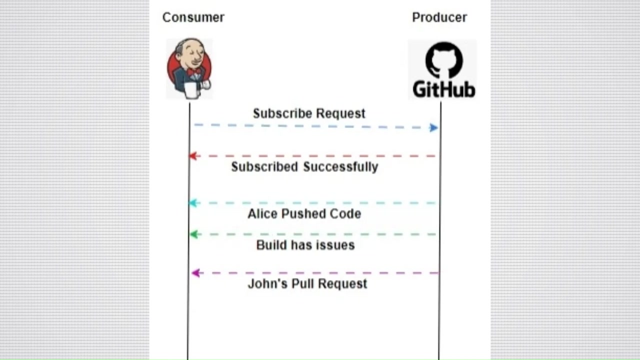 triggered the consumer when new events occur. It is important to note that the webhook protocol is usually used when server-to-server or application-to-application real-time communication is required. Let's understand how it works with an example. Suppose you have a continuous integration system or a deployment pipeline and you want 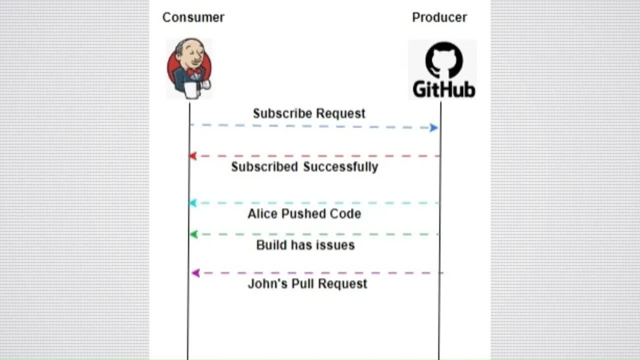 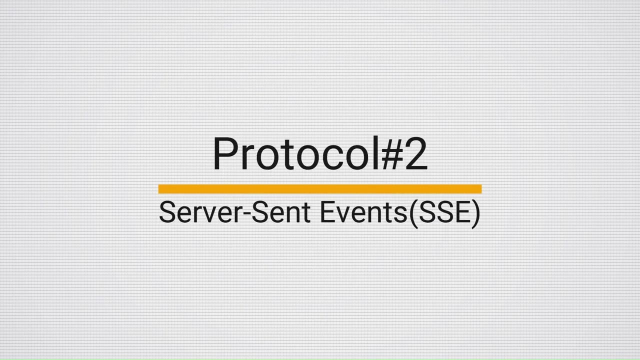 to receive real-time updates whenever certain events, like code push, pull request or any issues occur in your GitHub repository. In this scenario, you can use webhooks To establish communication between GitHub and your CI-CD system. Second Protocol – Server-Sent Events or SSC. 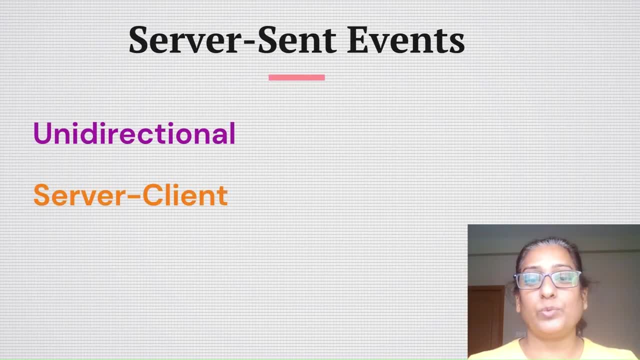 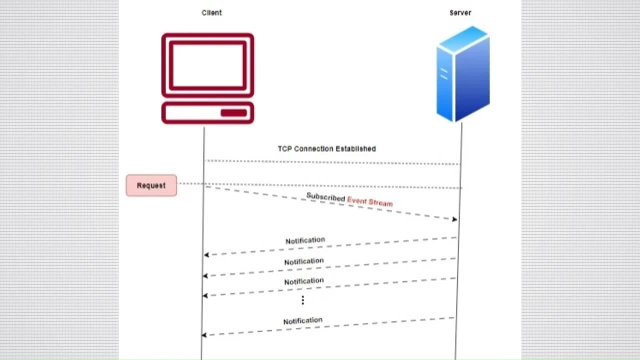 Server-sent events are unidirectional server-to-client server-push approach and are part of HTML5 specification. In server-sent events, communication is initiated by the client To establish a connection for receiving events. the client make the request to a specific. 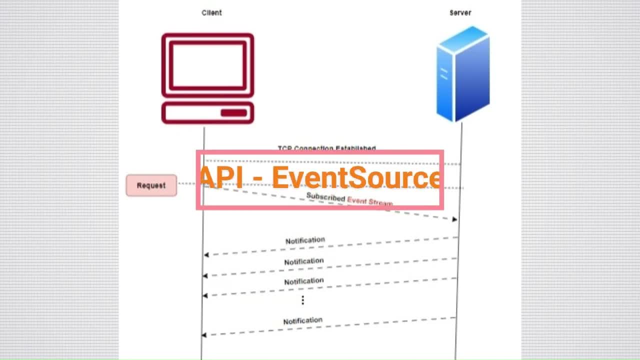 URL. This is typically done using a JavaScript API called event-source. When making the request, the client makes a request to a specific URL. This is typically done using a JavaScript API called event-source. When making the request, the client makes a request to a specific URL. 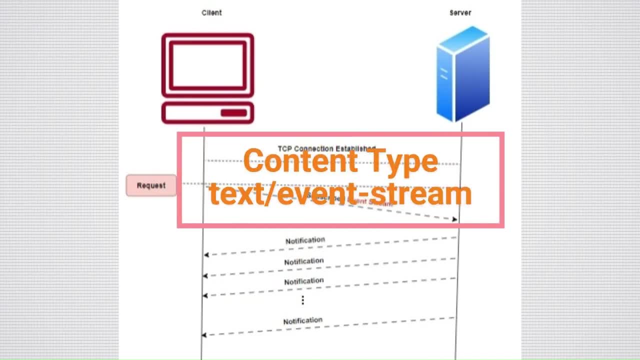 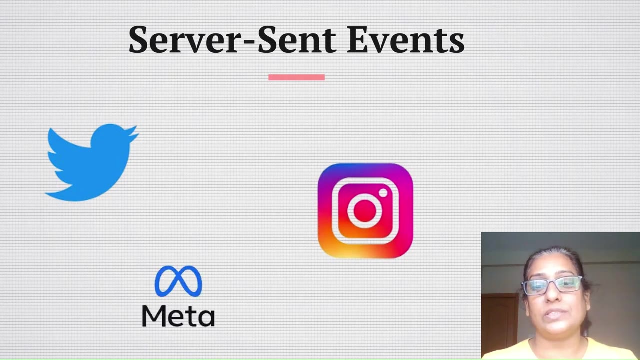 The client specifies the content type it can handle and text event stream. This is done through the HTTP accept header. SSC approach is mainly used for the notification system, where clients get notified by the server upon update. Twitter, Instagram and Meta are using the SSC for real-time newsfeed updates. 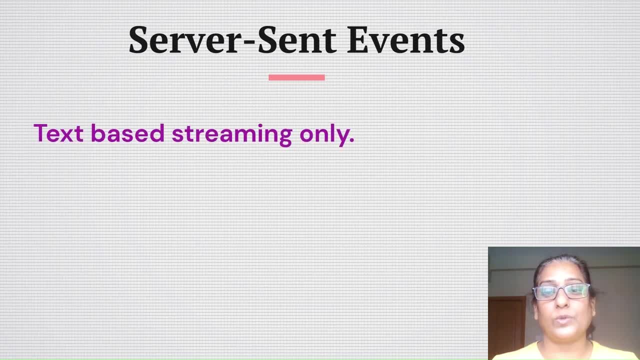 It's important to note that server-sent events supports only text-based streaming, making it unsuitable for audio or video streaming. Second Protocol – Server-Sent Events or SSC. Server-Sent Events or SSC. Server-Sent Events are only made for text based streaming. 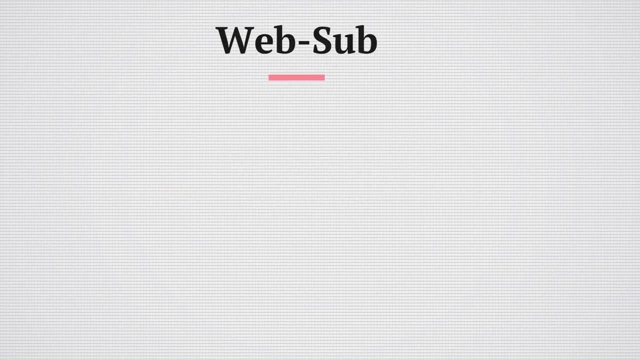 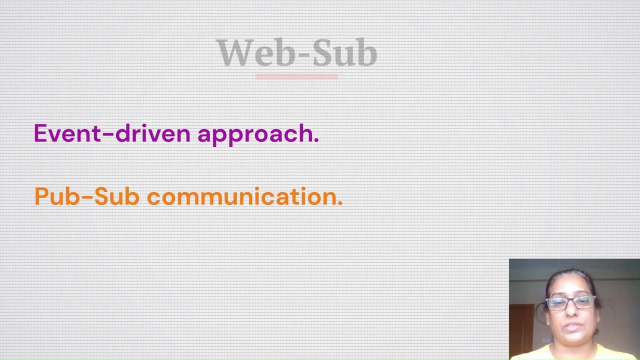 It's important to note that server-sent events supports only text based streaming, making it unsuitable for audio or video streaming. call Websub. Websub presents an event-driven architecture approach for distributed publisher subscriber communication. Its core components include a publisher hub and a subscriber. 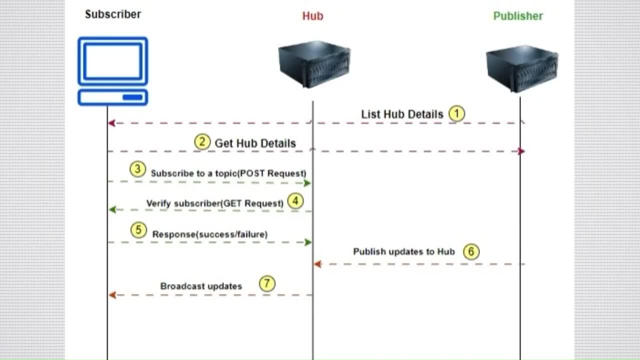 A hub acts as an intermediary or middleman in the communication flow between publishers and subscribers. It facilitates the distribution of content from publishers to the subscribers and decouples publishers and subscribers, ensuring seamless content delivery. One example of a hub is the Google's product PubSubHubBub, or also called PushHub. Websub facilitates multiple clients. 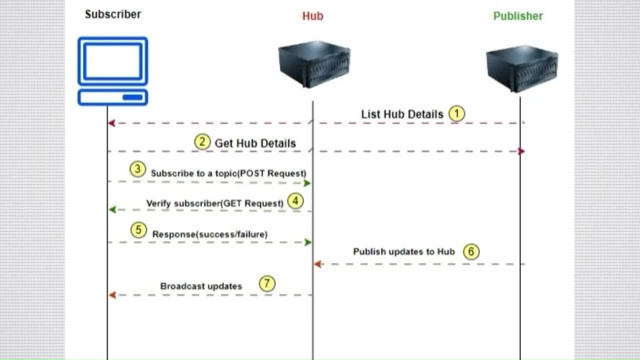 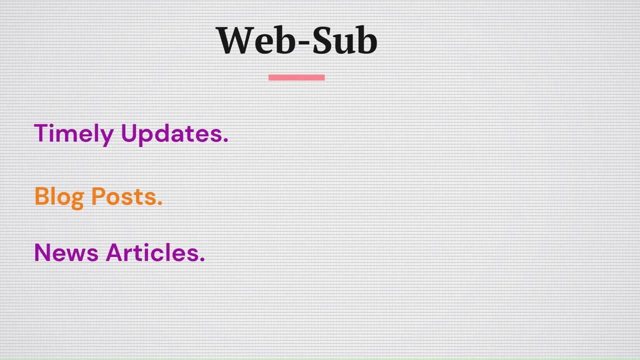 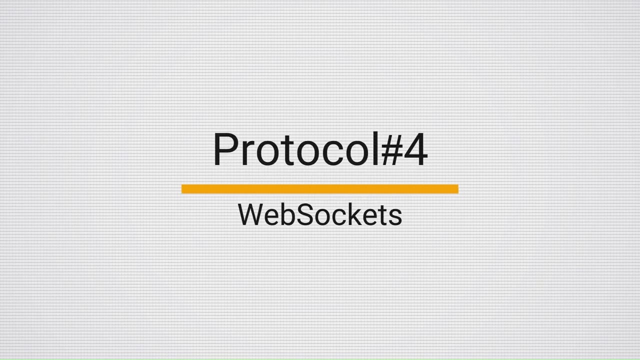 receiving updates from the same producers, with built-in security features. It is specifically tailored for scenarios where timely updates to web content, such as blog posts or news articles, are essential. It is commonly used in content distribution and syndication For both and the last protocol, WebSockets. WebSocket protocol enables bi-directional 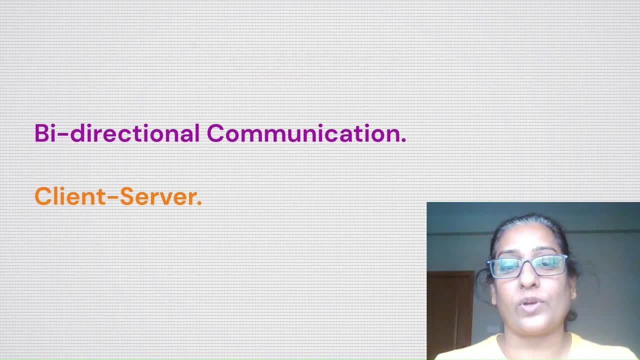 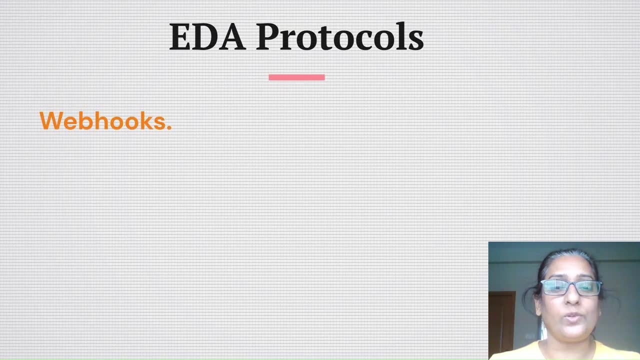 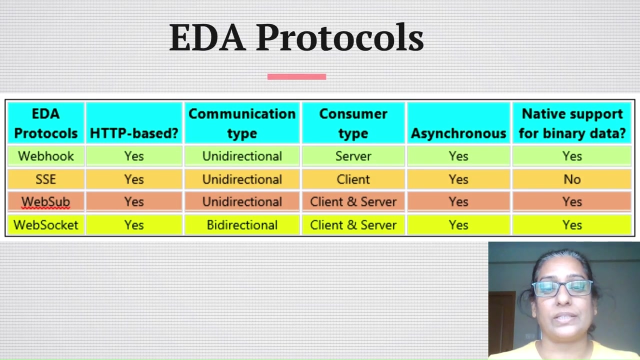 communication between the clients and the servers. We have discussed WebSocket at length in our previous video. I suggest you watch that. In this video we discussed protocols used in event-driven architecture. The choice of protocol depends on the specific communication needs of your application. Each protocol has its own unique attributes. SSE is suitable for text payloads. 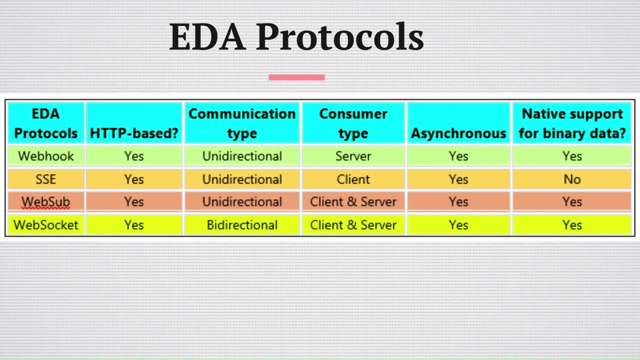 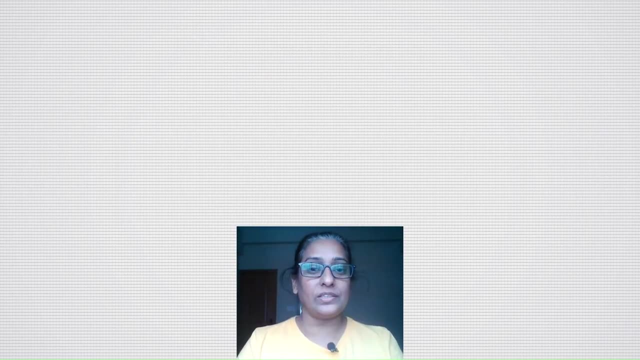 to clients. WebSub excels in scenarios involving both clients and servers, and WebSocket enables unrestricted bi-directional communication. Understanding these protocols empowers developers to select the most suitable approach for efficient and real-time communication in diverse applications. If you liked this video. 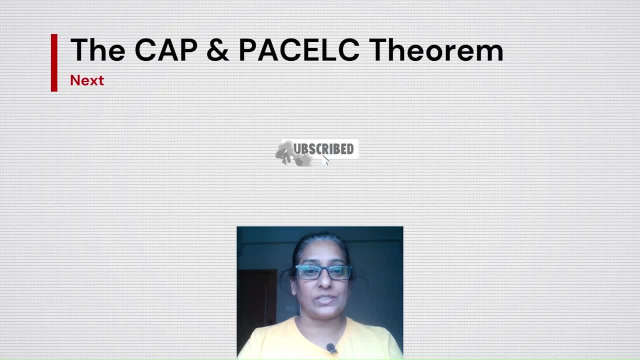 then do check out our other videos. Don't forget to like, comment this video and subscribe to my channel. My name is Rupa and I thank you so much for watching this video. See you in the next video. Today we will explore the CAP theorem: strong and eventual consistency. 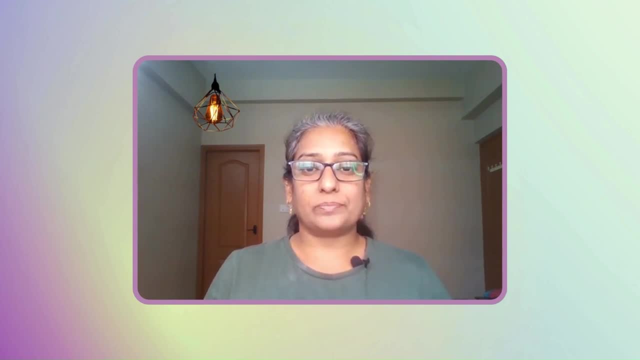 and the PACLC theorem, with some real-world examples. The CAP theorem states that in the design of a distributed system, it is impossible to guarantee all the three properties- consistency, availability and partition tolerance- simultaneously. But do you know that this statement is misleading? That's right, It is misleading. 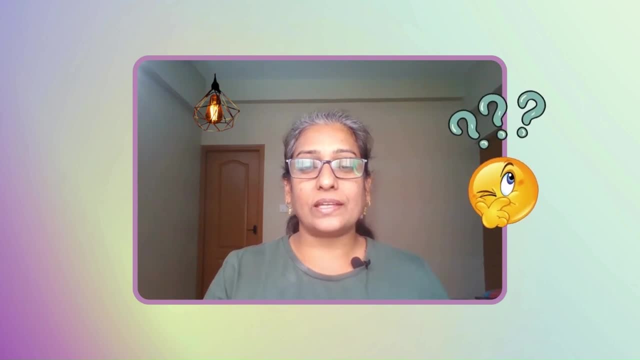 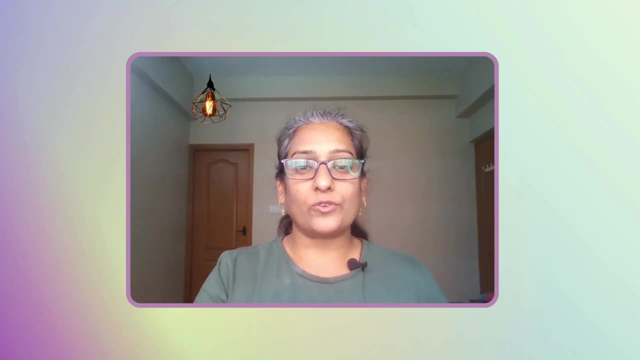 Let's discuss that in detail and understand why we are saying it is misleading. Hi there, Welcome to Tech and Career Points. I'm a software professional with over two decades of experience, including seven years in leadership roles at a global product-based organization. Let's first understand the three properties: consistency- 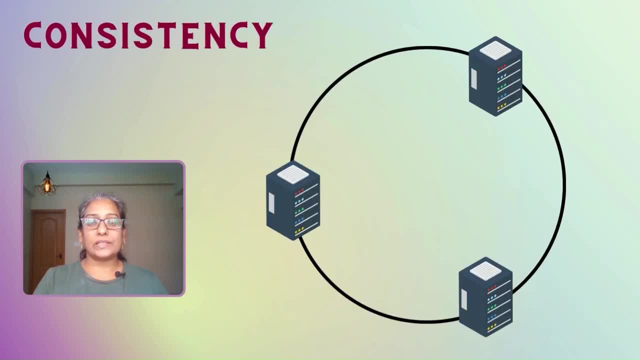 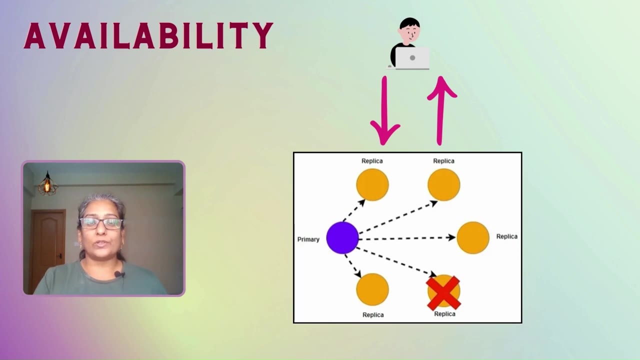 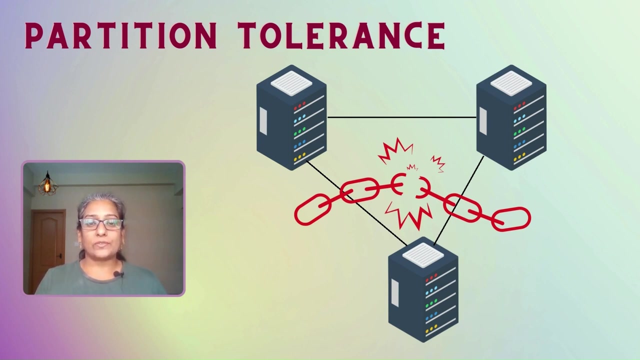 availability and partition tolerance. Consistency ensures all nodes in a distributed system see the same data simultaneously. This is crucial for data integrity. Availability means every request gets a response regardless of node failures or network partitions, And partition tolerance allows the system to function despite network issues. Network partition happens when the nodes 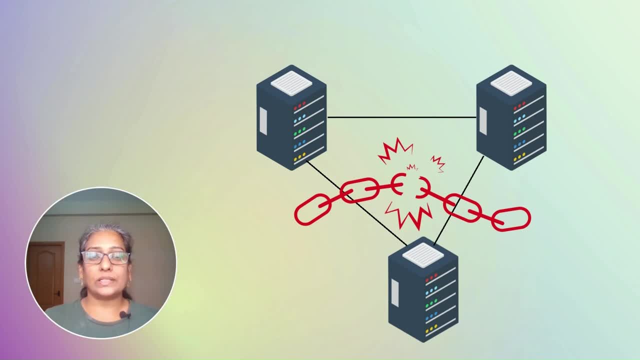 lose connection, causing them to split into separate groups that can't share any data In any distributed system. network partitions are inevitable, Whether we like it or not. they will happen When the network is functioning correctly. the system can provide both consistency and 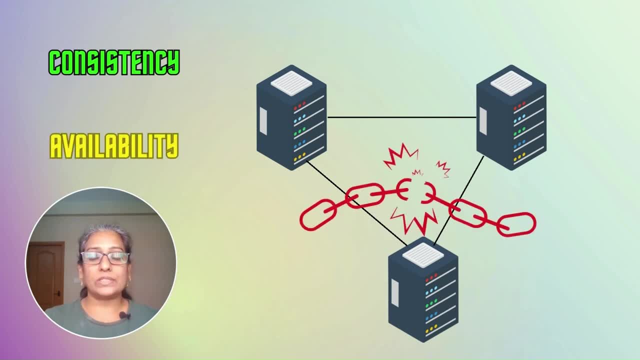 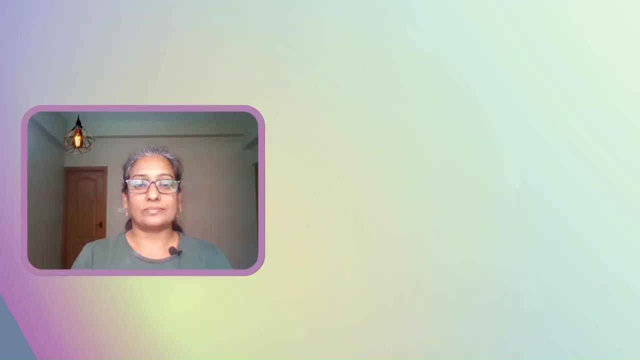 availability And when the network partition happens, we must choose either consistency or availability. Thus, a better way of phrasing the CAP theorem would be consistent or available when the network is partitioned. A system can either be consistent or available when the network is partitioned. 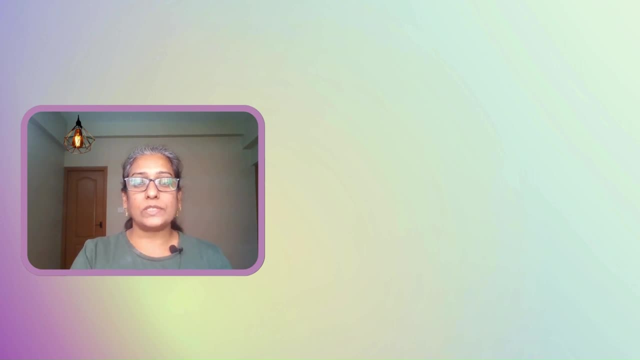 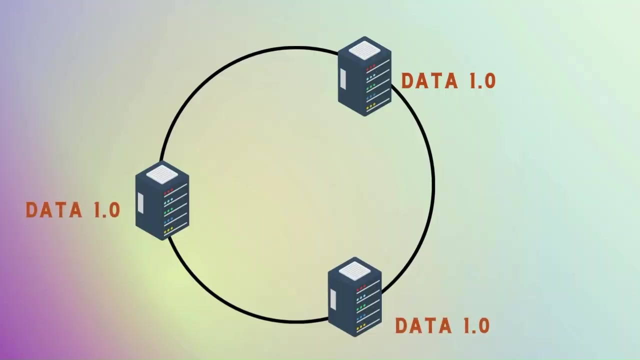 That makes sense right Now. if a system chooses consistency over availability, it means that it prioritizes maintaining a consistent view of the data and may sacrifice availability during network partitions. This is because when the communication between nodes fail, the data in each of these nodes may become out of sync. One or more nodes. 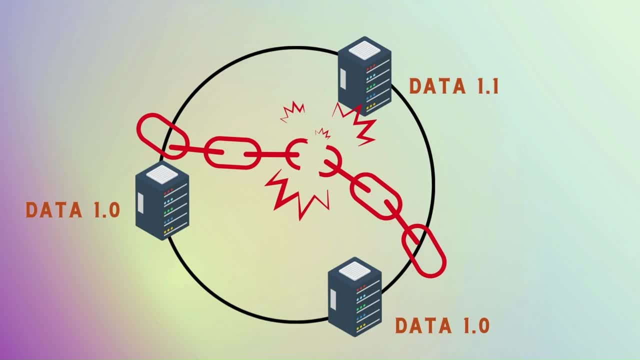 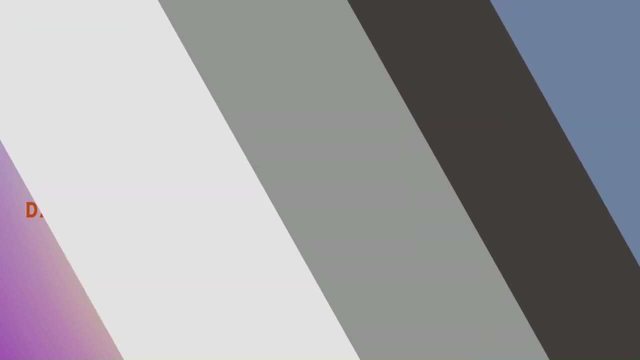 may have latest data, while the other may have still data. In this case, as we do not want to compromise on the data consistency, the system may refuse to respond to requests until consistency is restored, thereby compromising system availability. Let's understand this better with a real-world. 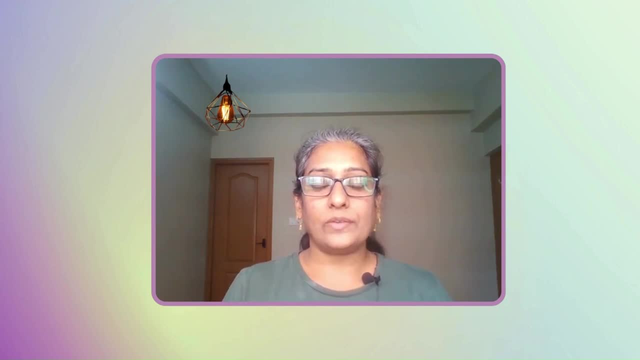 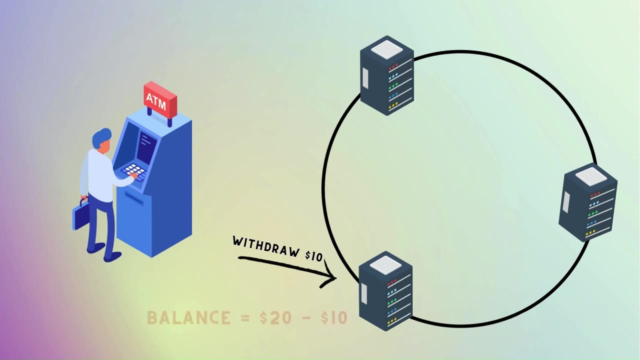 example. Think of a bank where having the right account balance is really important. If a user has an ATM and the transaction gets recorded on one part of the system but not on another because of a problem, the user might see different account balances when checking their balance. 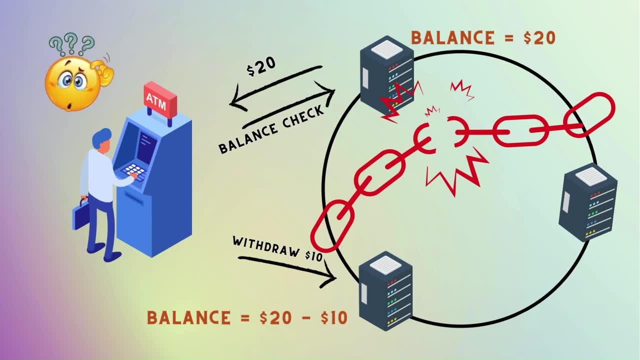 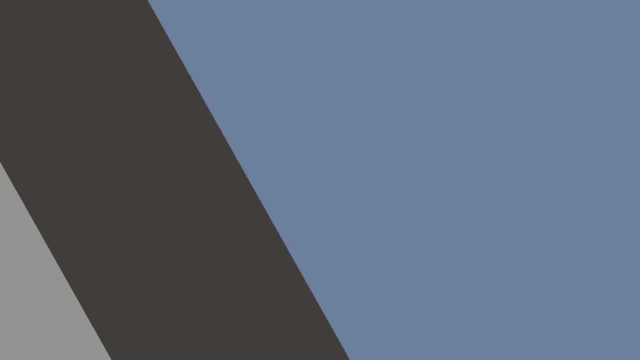 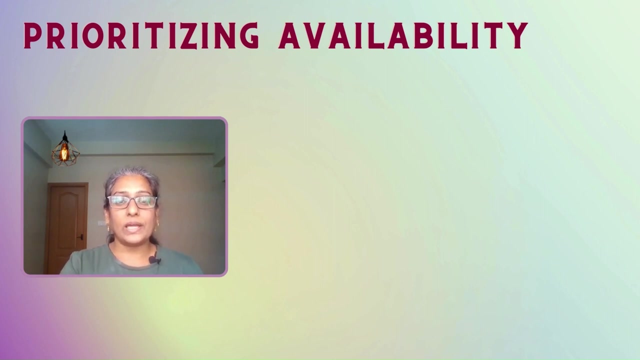 This is not a good experience, isn't it? The user may panic To avoid this during a network partition. if a user tries to withdraw funds, the system might temporarily reject the transaction until the connection is restored. If a system chooses availability over consistency, it means that it prioritizes remaining 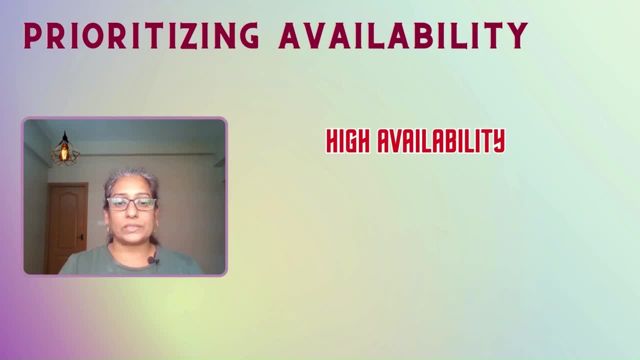 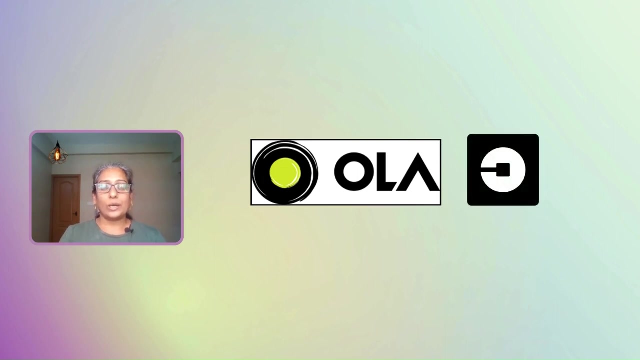 responsive and available even during network partitions, but may compromise strong consistency guarantees. In this situation, the system might temporarily allow different or conflicting data states until the consistency is restored. Think about OLA and ODA. They focus on being available so that the users can book the rides easily and the drivers can. 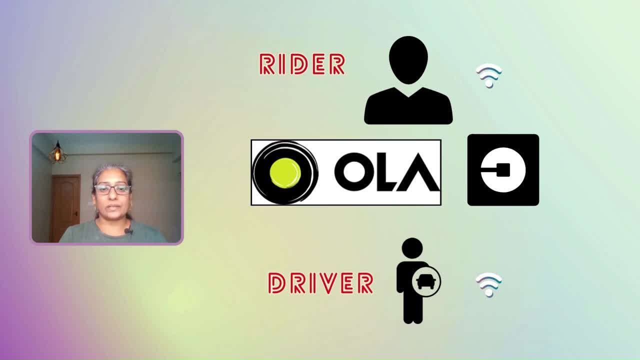 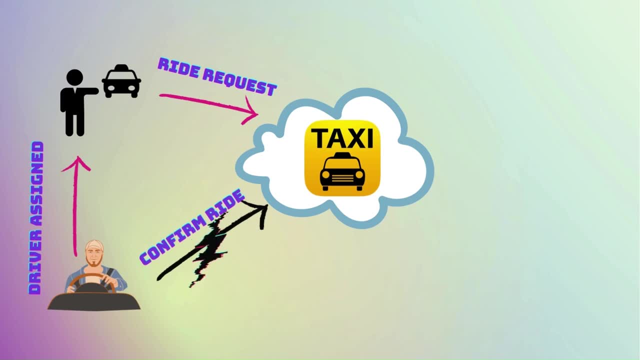 accept those requests even in areas with bad internet. During a network problem, if a driver accepts a ride but loses connection before confirming, the system might let them accept another ride to keep the service going. This could cause issues like double bookings or conflicting. 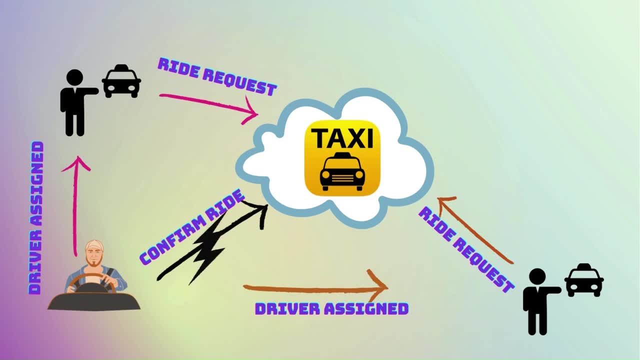 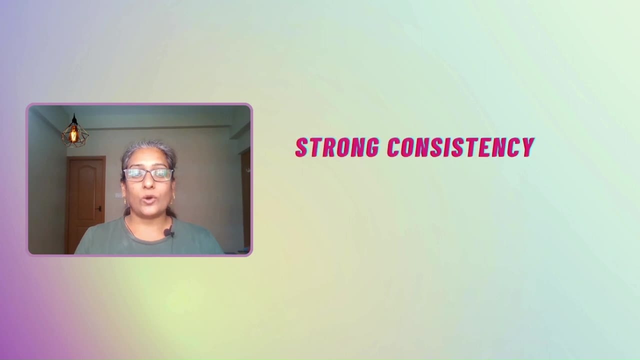 ride statuses until the connection is fixed. Even with these problems, the priority is keeping the service available for users without interruptions. A distributed system prioritizing consistency over availability offers strong consistency, and a system that prioritizes availability over consistency offers eventual consistency. Let's dive deeper into these two consistency models: strong consistency and eventual consistency. 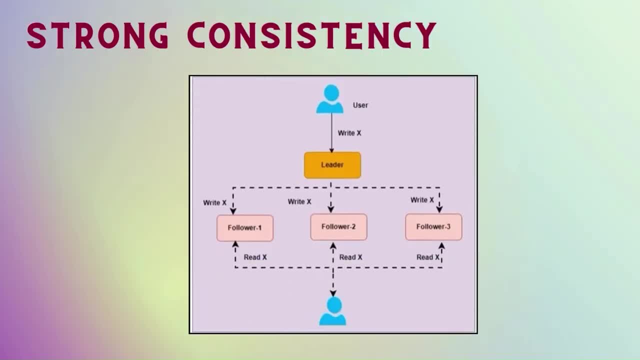 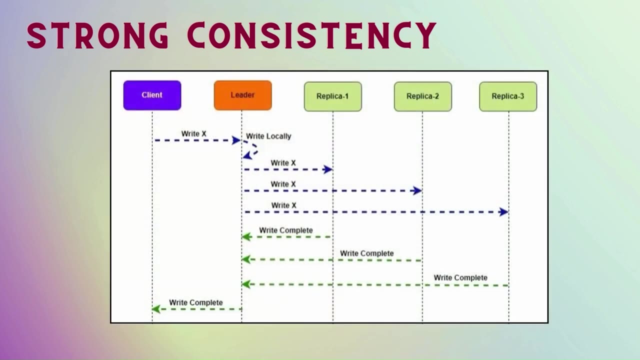 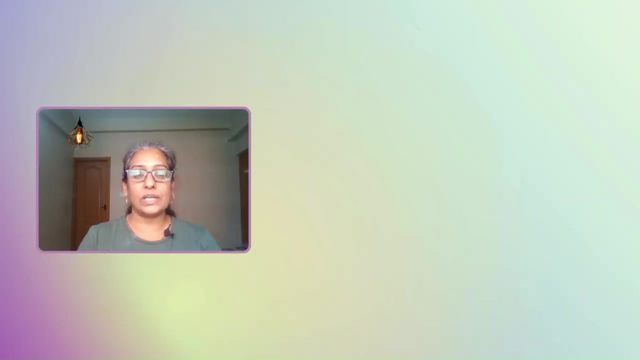 In a system that guarantees strong consistency, every node in the system sees the same data at the same time, regardless of where the data is accessed. Achieving strong consistency often requires synchronous replication and coordination among nodes. Synchronous replication and coordination among nodes results in increased latency and decreased 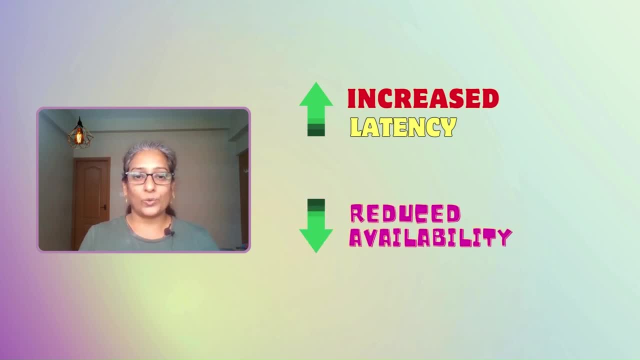 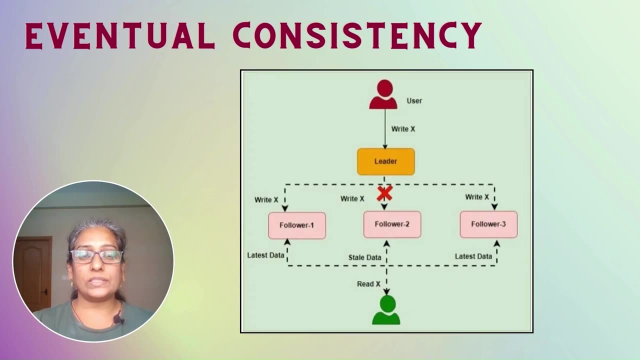 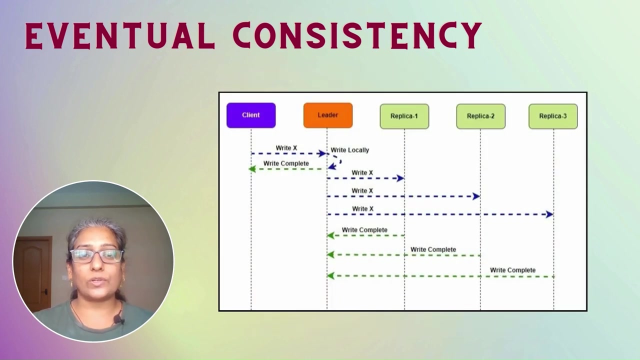 availability during network partitions. To know more, watch our video on replication. Eventual consistency is less strict than strong consistency and allows temporary inconsistencies during asynchronous updates across nodes. This approach focuses on keeping the system available and working even if there are network problems. 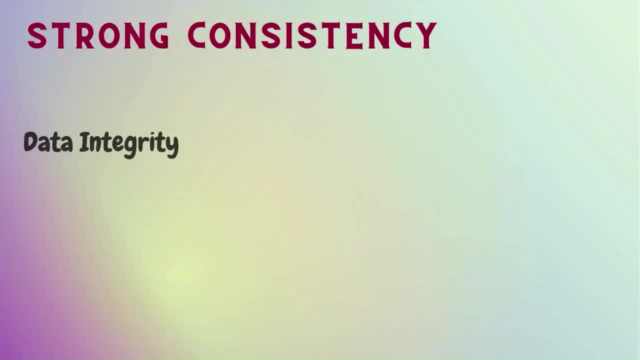 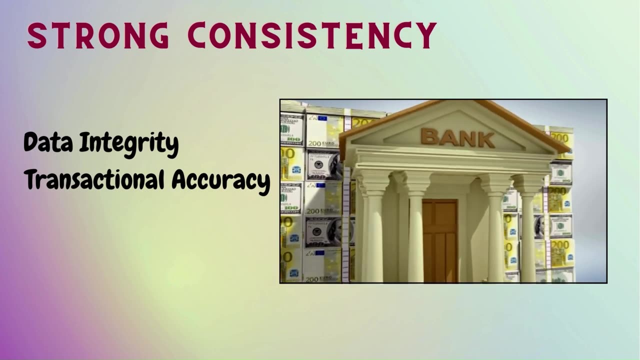 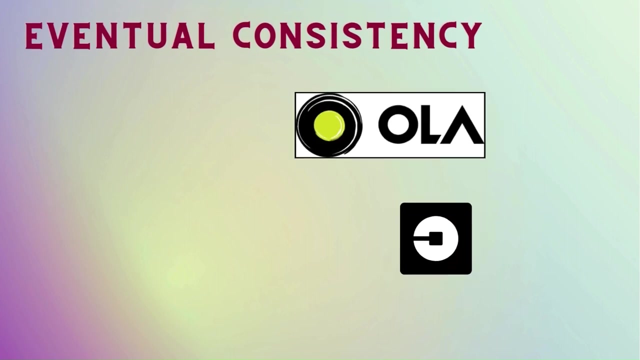 As we discussed earlier, applications that prioritize the data are not always consistent. Data integrity and transactional correctness, such as financial systems, may opt for strong consistency despite potential availability trade-offs. On the other hand, applications like Uber or Ola may prioritize availability and responsiveness. 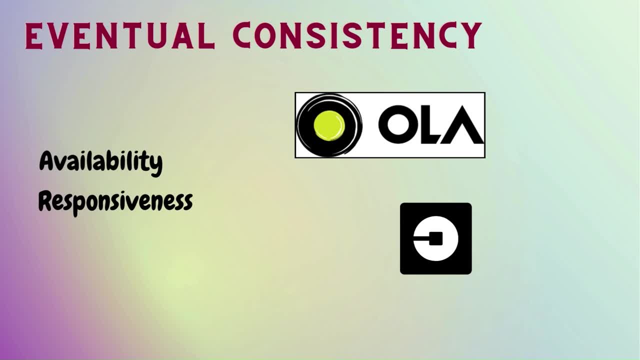 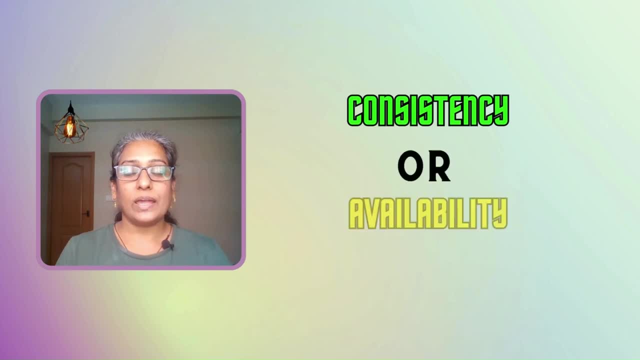 over strict consistency, making eventual consistency a more suitable choice. Just because the CAP theorem says either consistent or available does not mean we can't use the CAP theorem. This is not true. We can't achieve both consistency and availability. Confusing right. 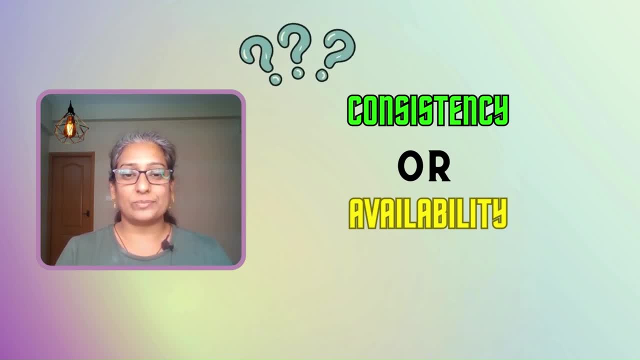 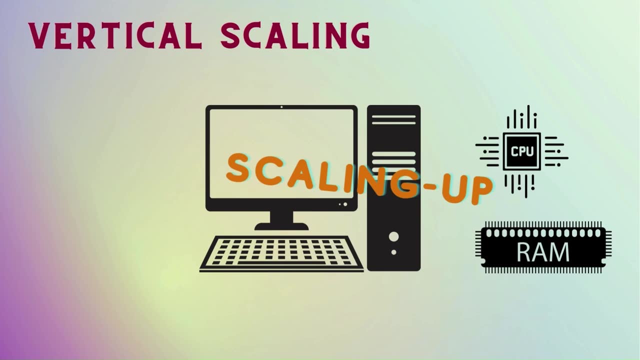 Let's discuss. By focusing on scaling up data centers vertically instead of spreading them out horizontally, we can have both consistency and availability, But the system won't be truly distributed anymore. Since network partitions are unavoidable in distributed systems, it's crucial to decide. 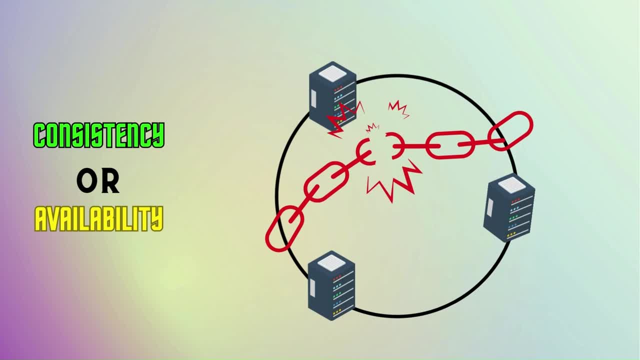 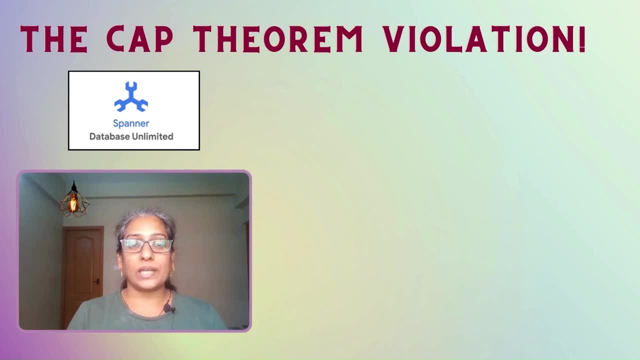 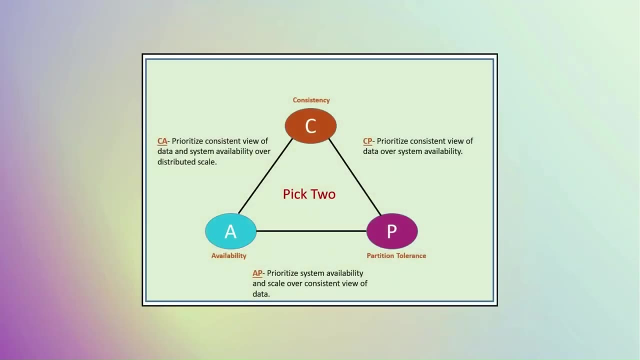 on the tight balance between consistency and availability. How do we know the consistency? Let's discuss. Google's Spanner Database seems to be an exception, though violating the CAP theorem. How Let's understand that Google's Spanner Database system is an interesting case study when it comes to the CAP theorem. 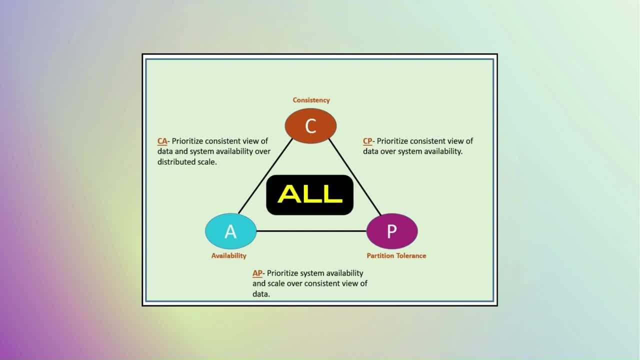 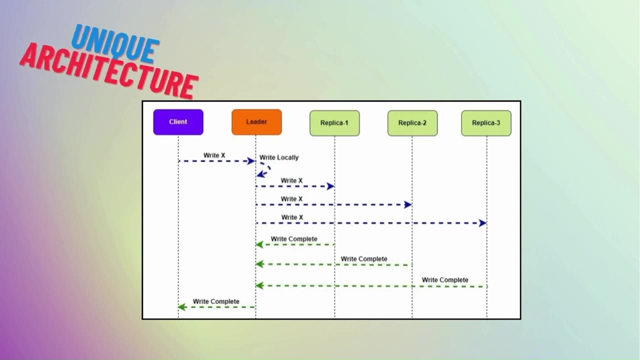 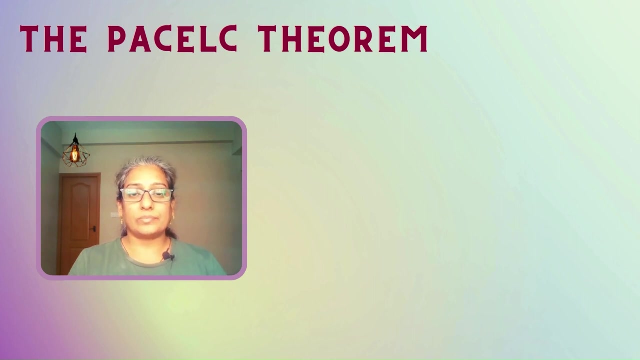 It aims to provide high availability and partition tolerance, while maintaining a strong consistency across its geographically distributed data centers. It achieves this by implementing a unique architecture and leveraging synchronously replicated data across multiple data centers. Now let's discuss the PAC-LC theorem. 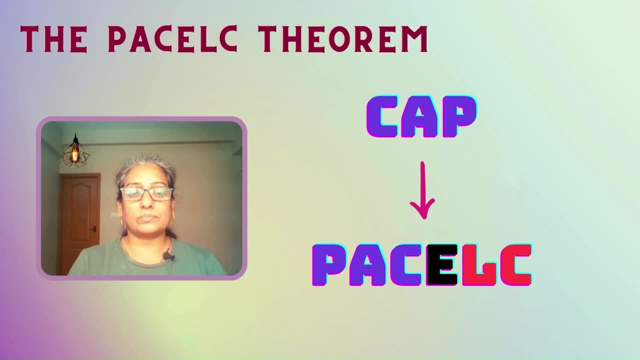 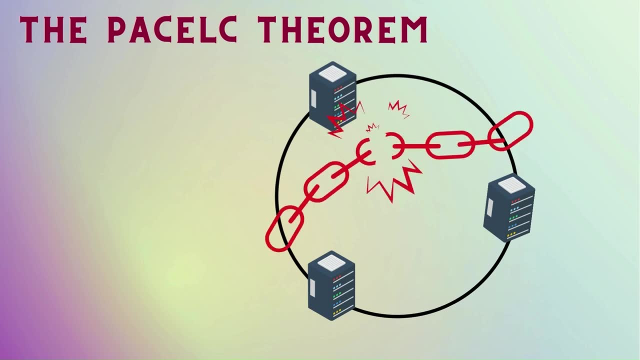 The PAC-LC theorem is an extension to the CAP theorem. The PAC-LC theorem states that during network partitions, a distributed system must choose a system between availability and consistency, as per the CAP theorem, Else when the system is functioning normally without partitions. 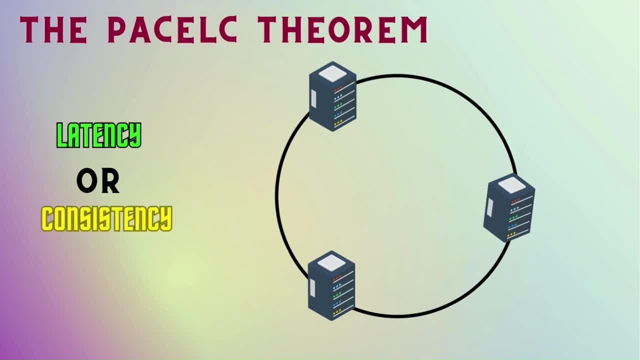 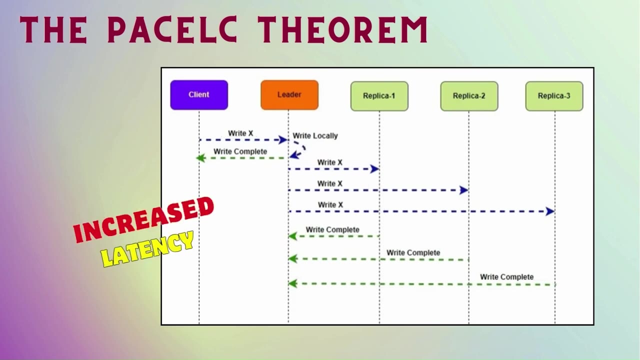 it must choose between latency and consistency When consistency is prioritized. in the absence of network partition, latency tends to suffer, because ensuring consistency often requires synchronous replication and coordination among nodes, which can increase the time it takes for operations to complete. To know more about synchronous replication, 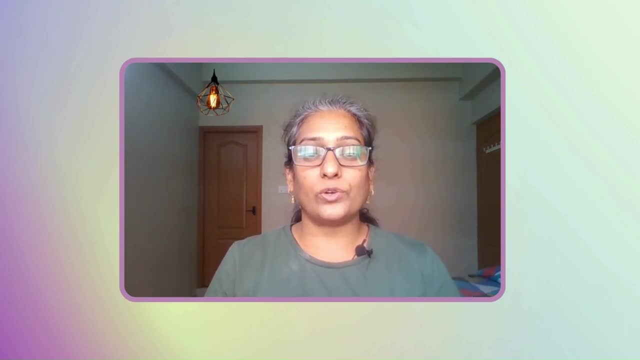 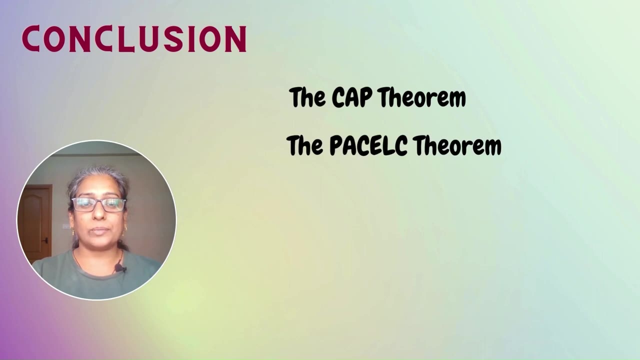 and its impact on availability. watch our video on replication. In conclusion, understanding the CAP theorem and PAC-LC theorem helps system designers make informed decisions, ensuring the creation of robust and resilient distributed systems. What will you prioritize in your next project- Consistency or Availability? 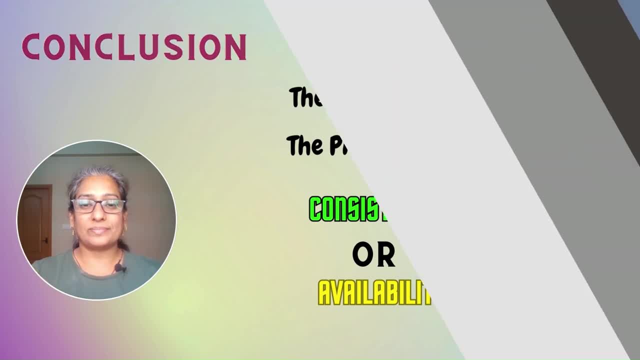 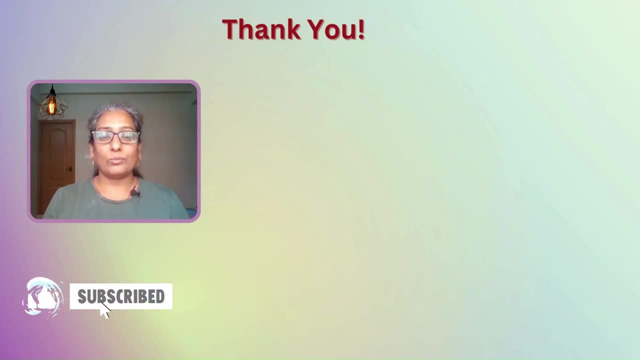 Do let me know in the comment section If you found this video helpful. give us a thumbs up and subscribe to our channel for more interesting tech topics. Also, do check out our other videos on software performance optimization, case studies, system design, big data, coding and career growth. 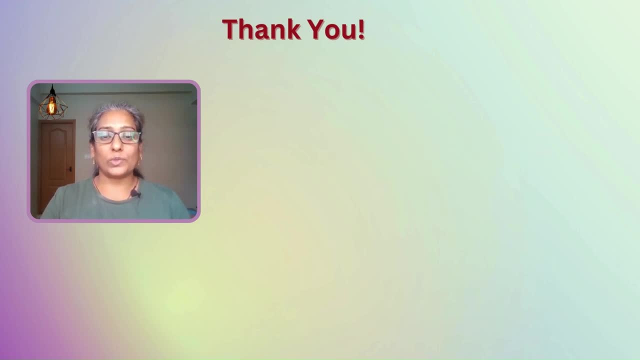 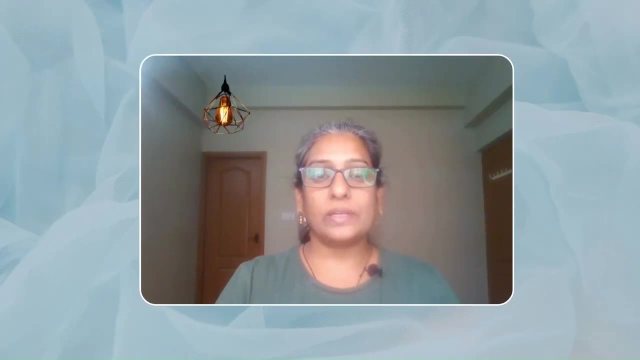 My name is Rupa and I thank you so much for watching this video. See you next time. Annoyed by slow-loading websites during busy times? Frustrating, isn't it? Well, there is a secret weapon companies use to stay speedy. 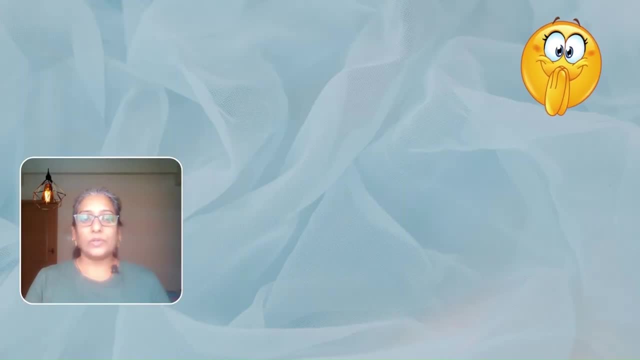 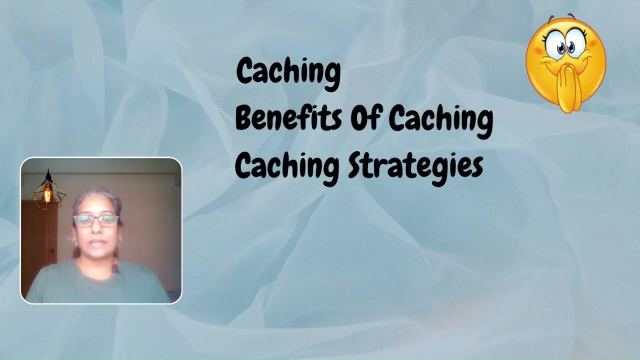 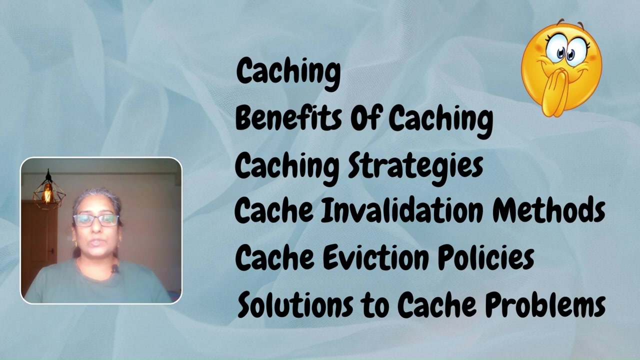 Caching. In today's video, we are going to cover almost everything about caching, including its benefits, caching strategies, cache invalidation methods, cache eviction policies and solutions to some common cache-related problems. It's going to be a lot of learning. 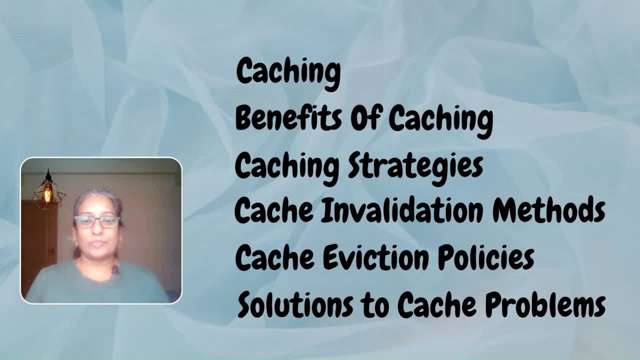 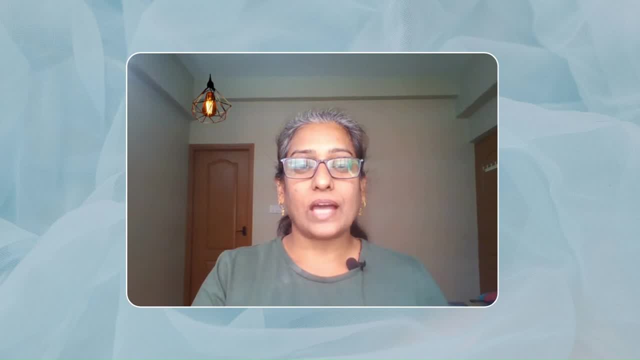 and fun learning, So keep watching till the end. Hi there, welcome to Tech and Career Points. I'm a software professional with over two decades of experience, including seven years in leadership roles at a global product-based organization. In today's world, users expect lightning, fast-forwarding. 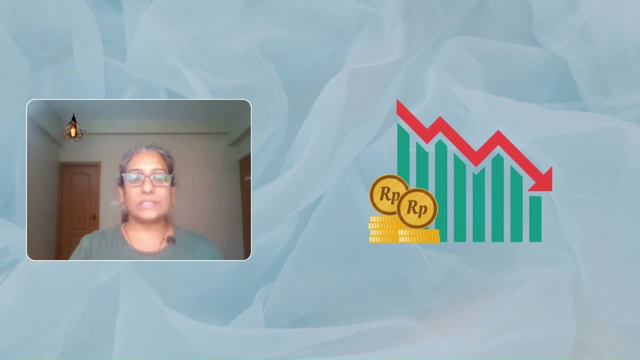 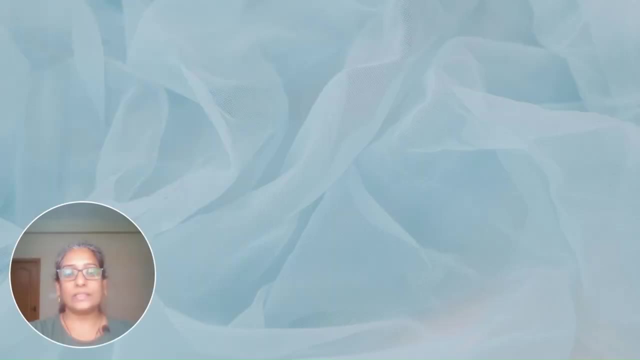 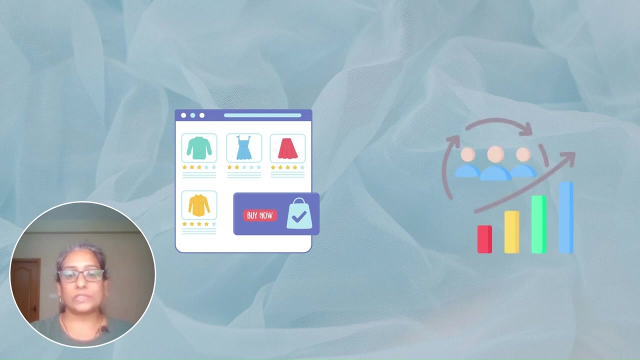 right-to-lost websites. But as the traffic peaks, the performance can suffer, And that's where caching comes in. Consider a popular e-commerce platform experiencing a surge in user traffic during a festive season sale. As the number of users increase, so does the volume of database queries. 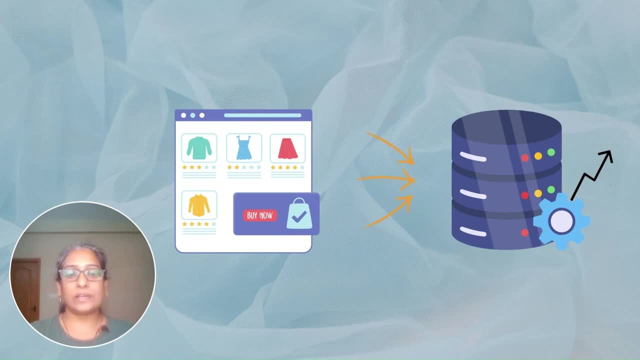 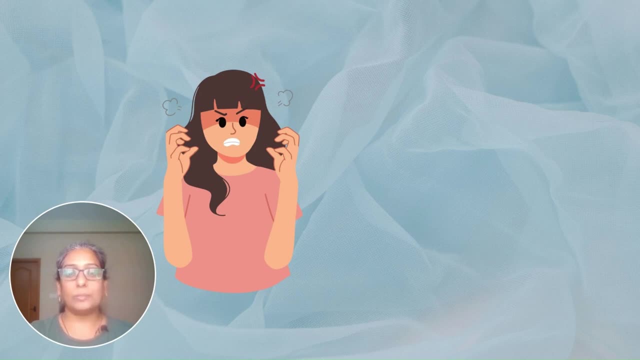 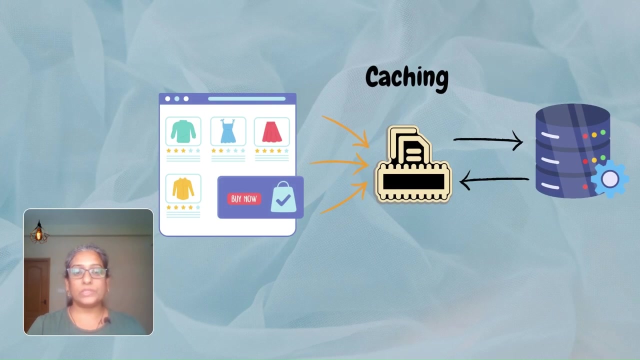 resulting in sluggish performance and delayed response times. This performance data is linked to the search results. This performance degradation impacts the user experience and may lead to lost sales opportunities for the business. To mitigate the performance issues caused by increased database queries, the e-commerce 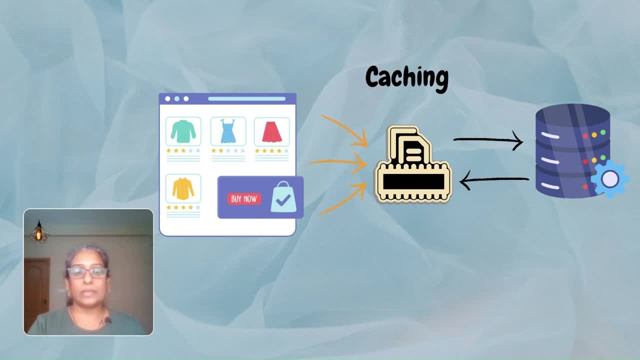 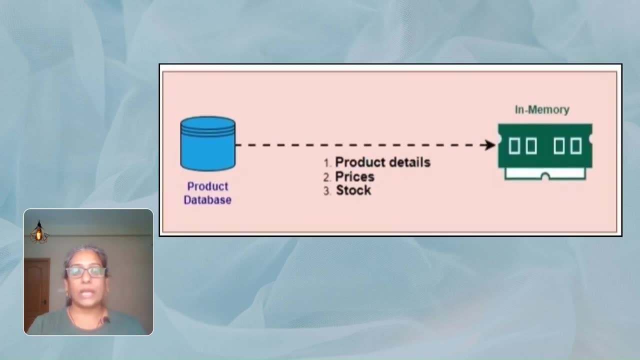 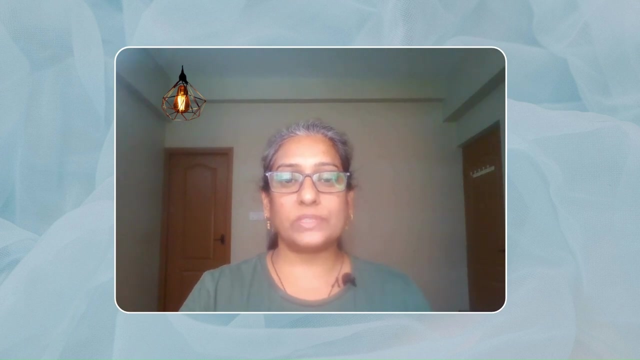 platform decides to implement caching. By caching frequently accessed information such as product details, prices and availability, the platform aims to reduce the database queries and deliver faster response time to users browsing the website or making purchases. But will the caching really help the e-commerce platform mitigate the performance issue? 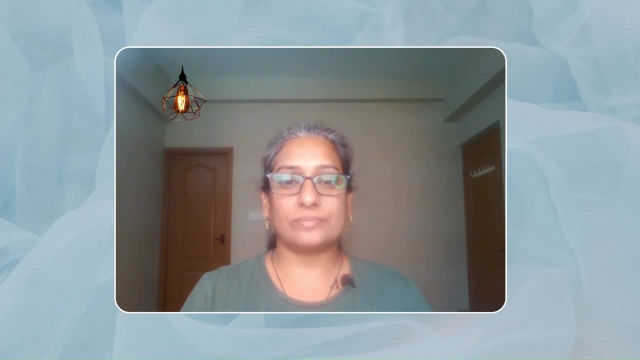 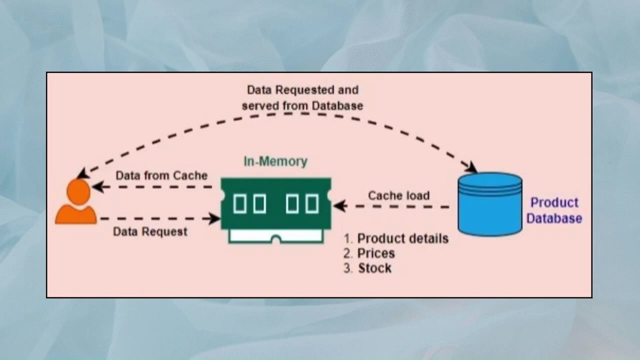 Let's understand how caching works. When a user visits the e-commerce platform to view product listings, the system first checks the cache for the requested product information. If the data is found to be correct, the caching is completed. If the data is found to be correct, the caching is completed. 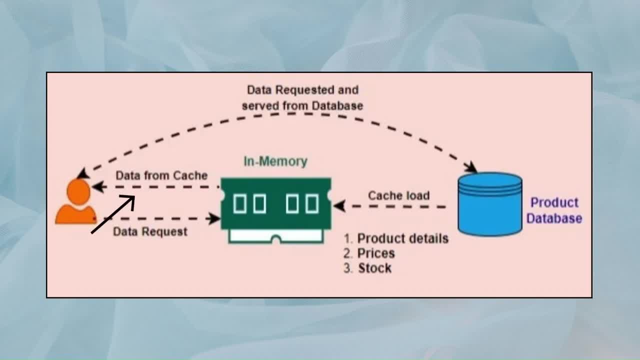 If the data is found to be correct, the caching is completed. If the data is found in the cache, it is retrieved quickly and served to the user, resulting in a seamless browsing experience. However, if the data is not present in the cache, the system retrieves the information. 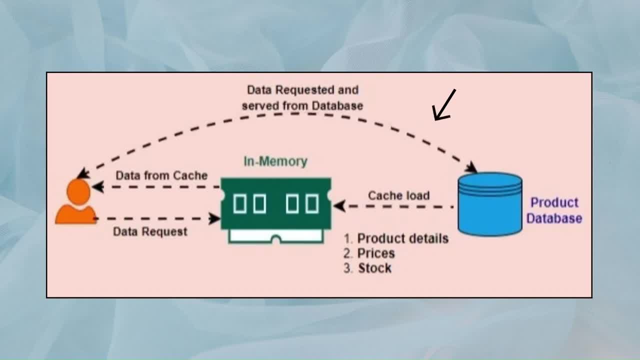 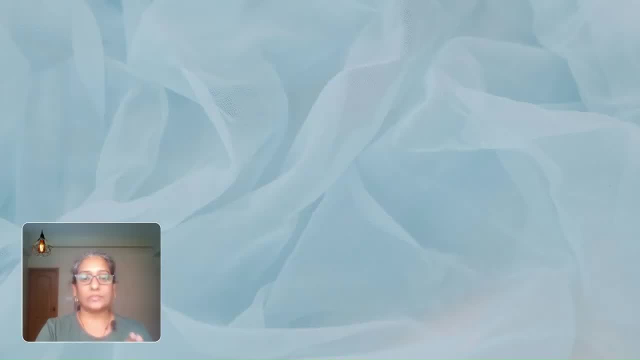 from the database, serves it to the user and updates the cache to prevent future incidents of not finding the data in the cache. If the data is found in the cache, it is called cache hit and if not, it is called cache miss. 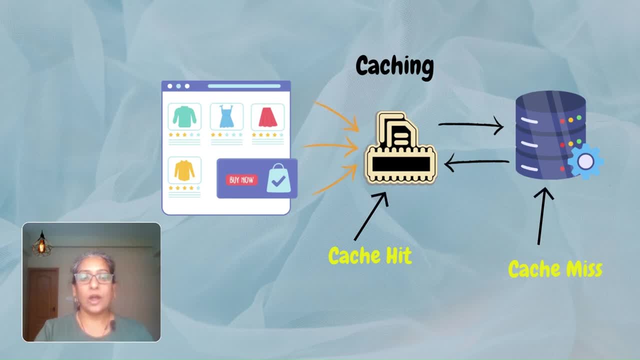 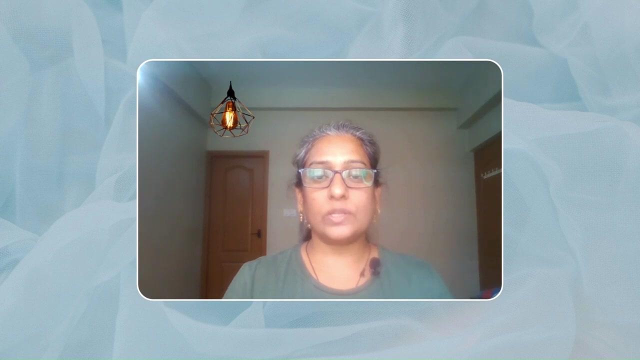 How does the desired data get loaded to the cache And how do we ensure synchronization between the cache and the database? There are several caching strategies that help us keep the data in sync. Let's explore them. Caching strategies are the approaches to manage how data is stored and retrieved in a cache. 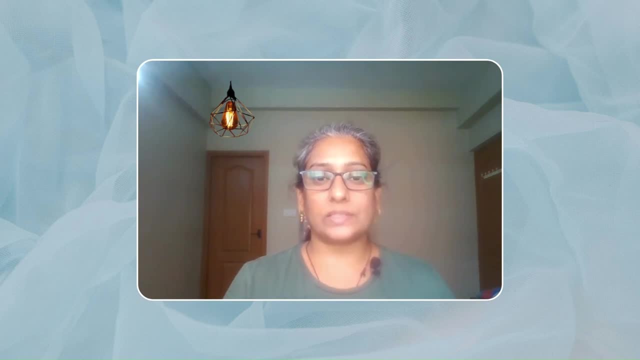 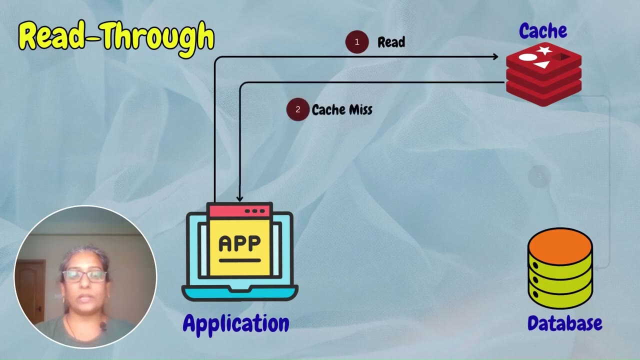 Let's understand a few commonly used caching strategies. In a read-through caching approach, when a cache misses the cache, the user will be able occurs. the system automatically fetches the data from the database, updates the cache and returns the data to the user using memcached for caching of frequently accessed database queries in a web. 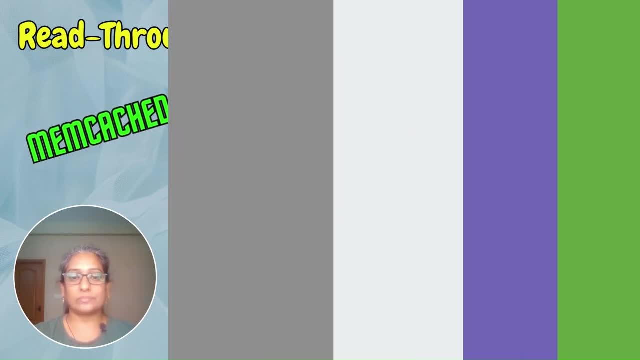 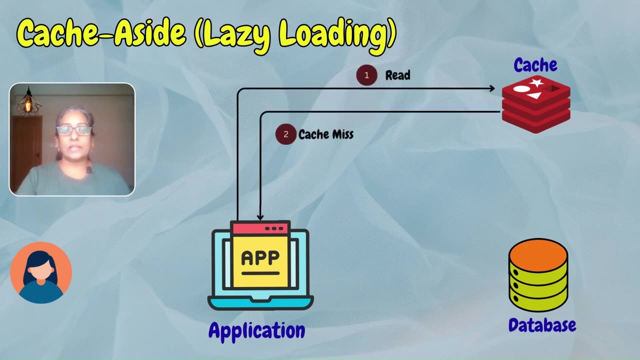 application is an example of read through cache in cache aside caching. when a cache miss occurs, the application directly fetches the data from the database, updates the cache and returns the result to the user. mongodb caching. frequently access to user profiles in a social media platform is an 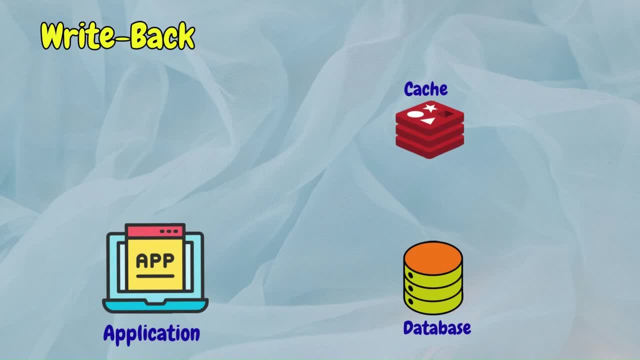 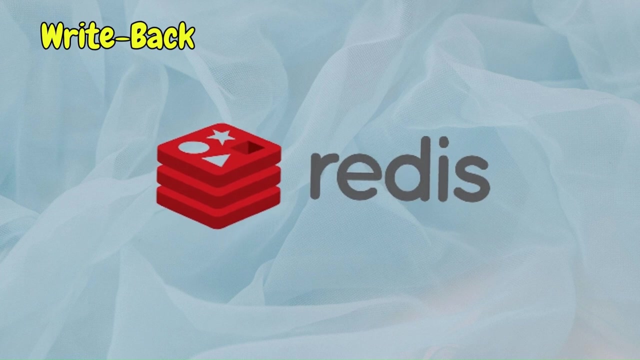 example of this caching. with writeback caching, data is returned to the cache first and then asynchronously return to the underlying storage at a later time. this strategy improves write performance by reducing the latency associated with synchronous disk writes. a database system caching write operations in memory before committing them to disk to improve overall system responsiveness and 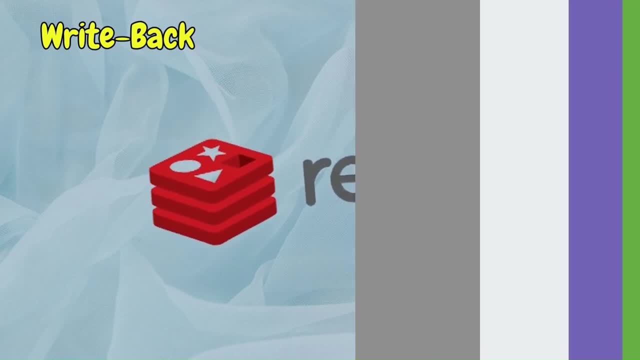 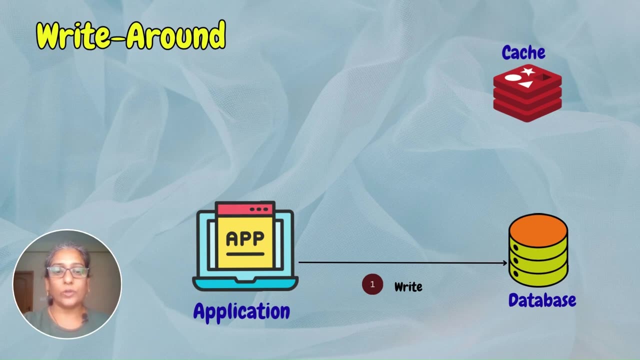 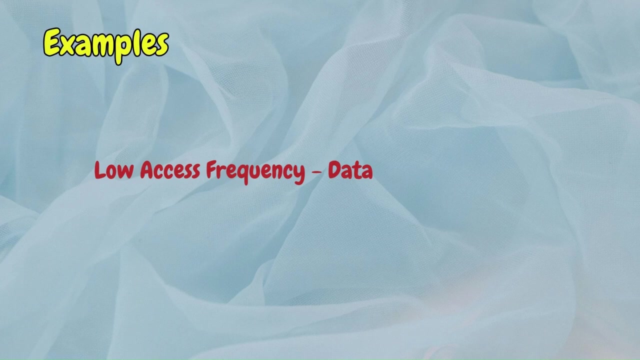 and throughput is an example of this caching. in write aside caching strategy, the data is directly written to the underlying storage without being cached initially, only subsequent read request for the same data trigger caching. this approach is beneficial for data with low access frequency or data that doesn't have a caching function. 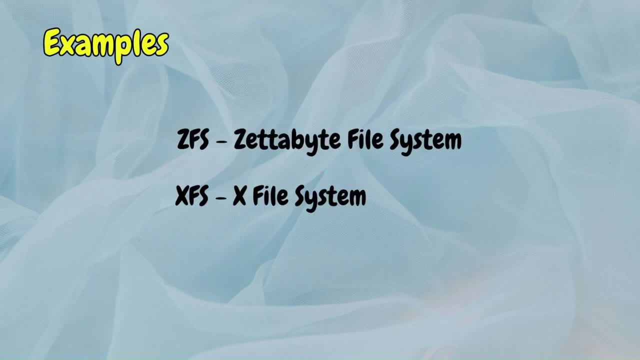 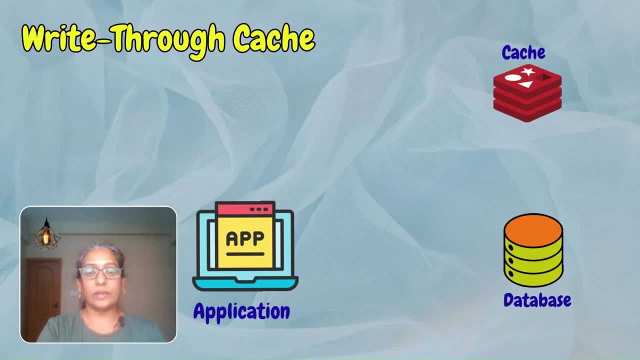 not benefit from caching. an example of this caching would be a file storage system where large files are written directly to disk without being cached. to optimize cache utilization for frequently accessed files in write through cache, every write operation to the database is also written to the cache simultaneously. this ensures that the cache is always up to date with 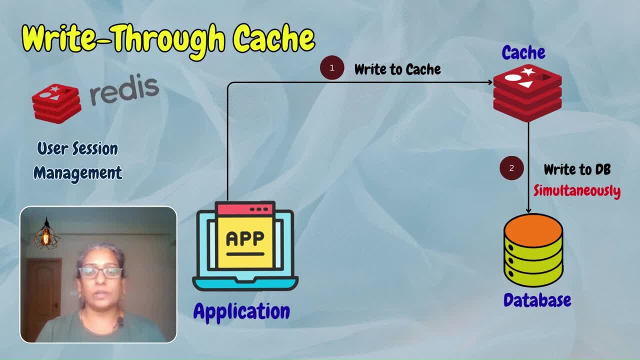 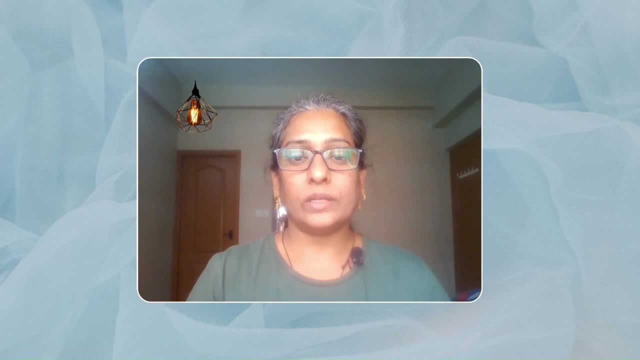 the latest data ready's cache with the latest data is always up to date with the latest data with write through caching for user session management is an example of this. okay, now that we have loaded the data in the cache, how do we ensure that it is still valid and not? 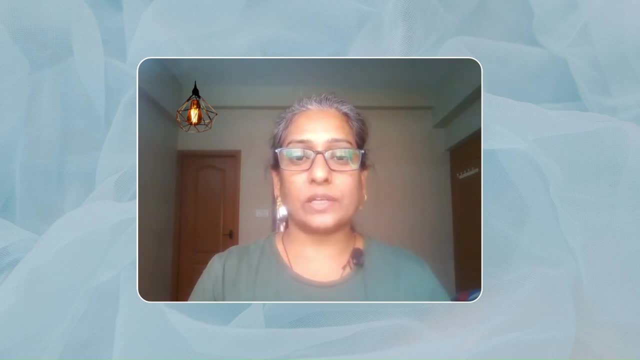 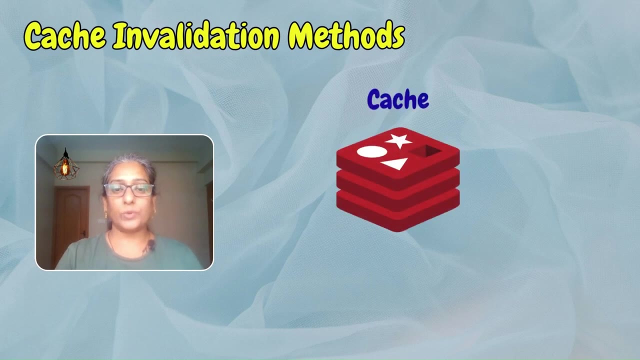 outdated. cache invalidation methods confirm that the cached data is in sync with the original source. cache innovation is the process of removing or updating the cache data when it becomes outdated. this ensures the accuracy of the cache data. cache invalidation methods are broadly classified into two: time based invalidation and event based invalidation. let's understand each of them in detail. 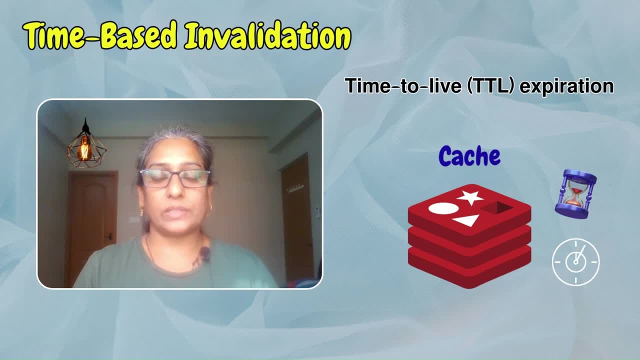 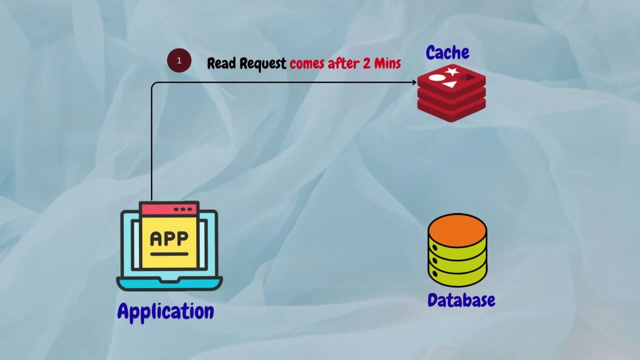 time to live. expiration is a time based invalidation method. this method involves setting a time to live value for cached content, after which the content is considered stale and cached content is considered stale. and cached content is considered stale and must be refreshed when a request is received for the content. the cache checks the time to 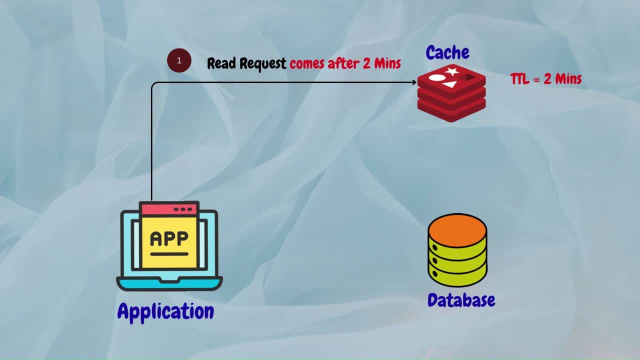 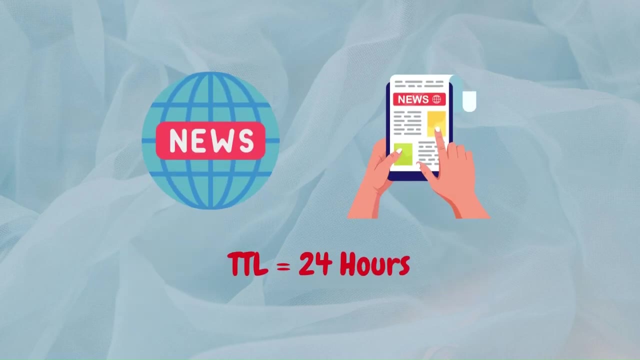 leave value and serves the cached content only if the value has not expired. if the value has expired, the cache fetches the latest version of the content from the origin server and caches it, for example, in a news application. articles in the cache may have a ttl of 24 hours. 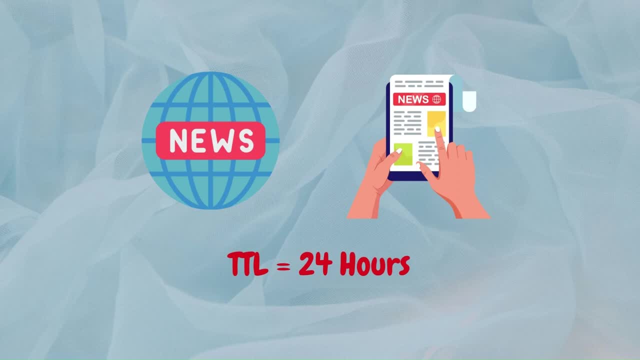 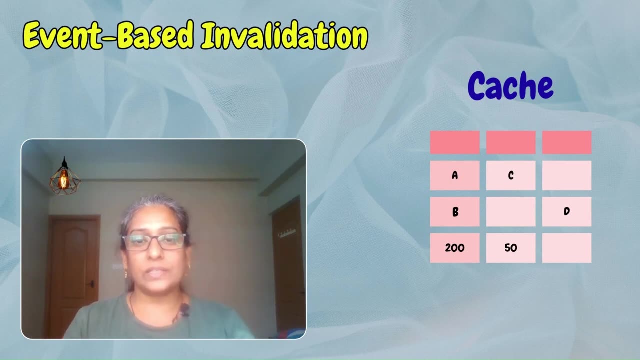 After 24 hours, the articles expire and are removed from the cache. In event-based invalidation, the cached entries are invalidated based on specific events or triggers, such as data updates or deletions. Let's discuss some commonly used event-based invalidation methods. 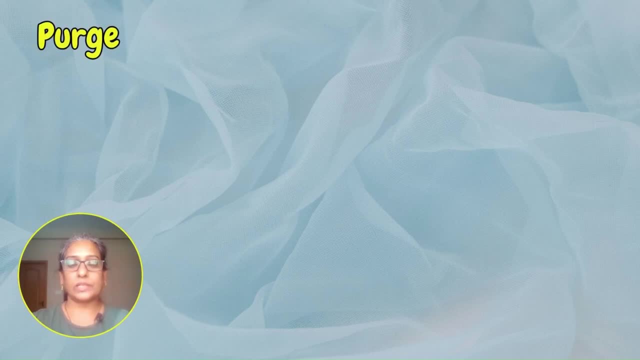 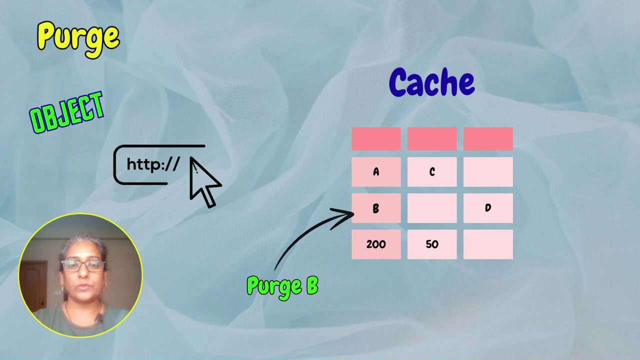 The purge method removes the cached content for a specific object URL or a set of URLs. It is typically used when there is a change or update to the content and the cached version is no longer valid. When a purge request arrives, the cached content is removed immediately. 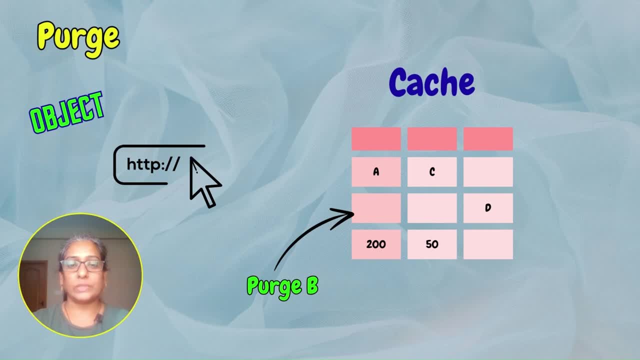 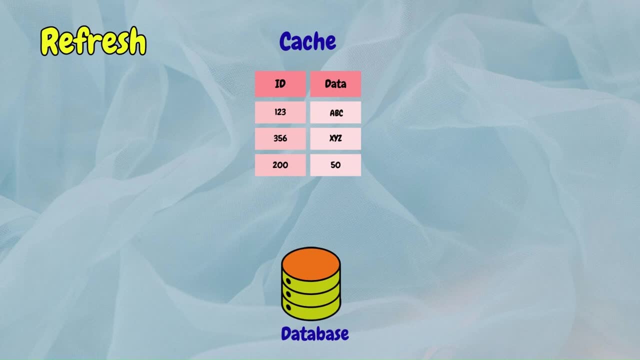 and the next request for the content will be served directly from the origin server. Refresh method fetches a request to remove the cached content from the origin server. even if cached content is available, When a refresher request is received, the cached content is updated with the latest version from the origin server. 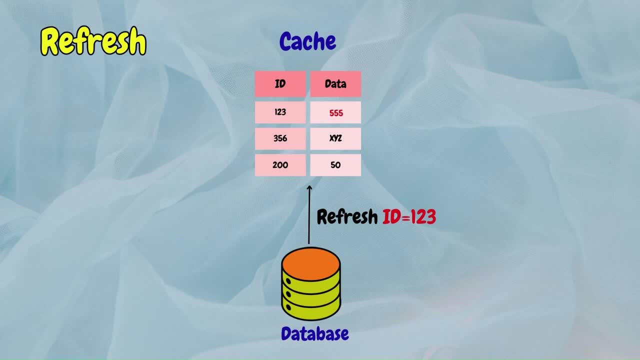 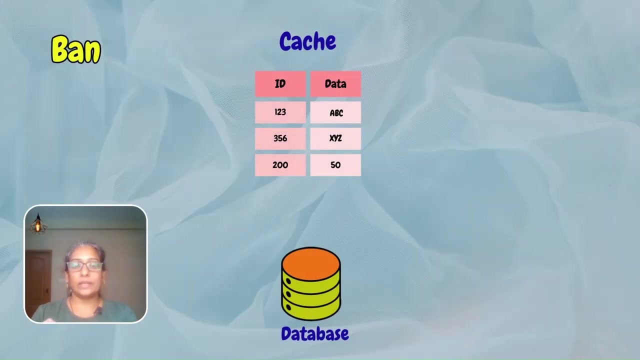 ensuring that the content is up to date. Unlike a purge, a refresh request does not remove the existing cached content. Instead, it updates it with the latest version. The ban method invalidates the cached content based on a specific criteria, such as a URL pattern or a header. 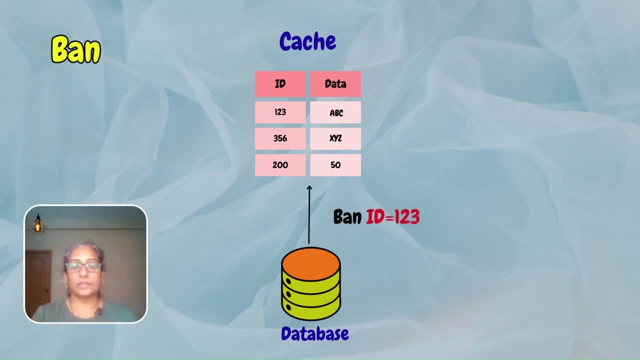 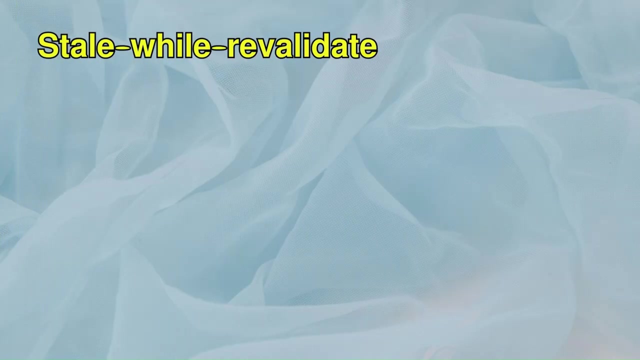 When a ban request is received, any cached content that matches the specified criteria is immediately removed and any subsequent requests for the content are served directly from the origin server Stale, while revalidate method is used in web browsers and CDNs to serve stale content from the cache. 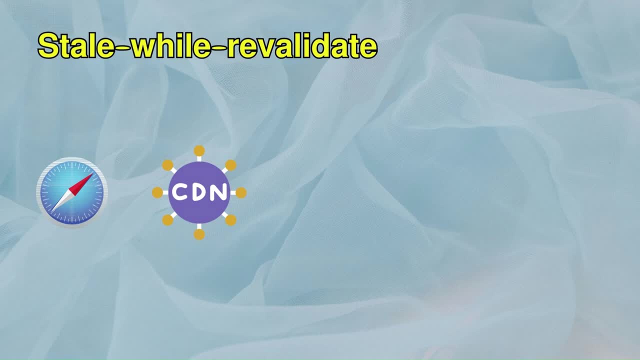 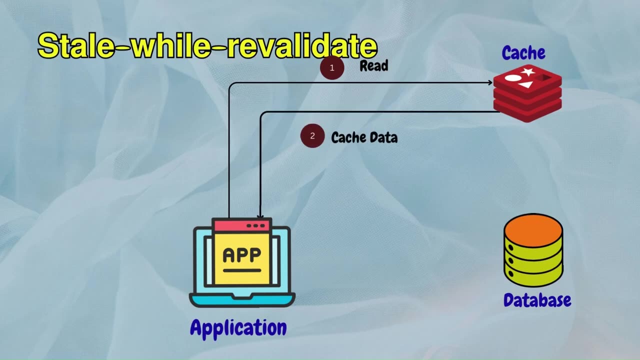 while the content is being updated in the background. When a request is received for a piece of content, the cached version is immediately served to the user and an asynchronous request is made to the origin server to fetch the latest version of the content. Once the latest version is available, the cached version is updated. 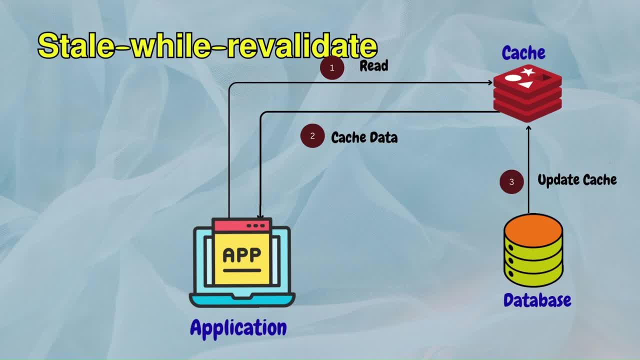 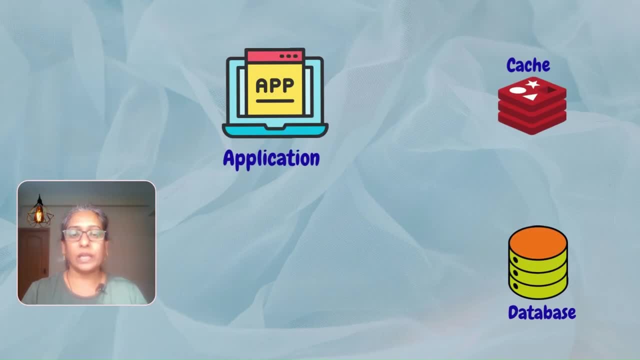 This method ensures that the user is always served content quickly, even if the cached version is slightly outdated. After the cache invalidation, it appears that the cache is full and has latest data, But the cache misses have increased tremendously. So what steps should be taken next? 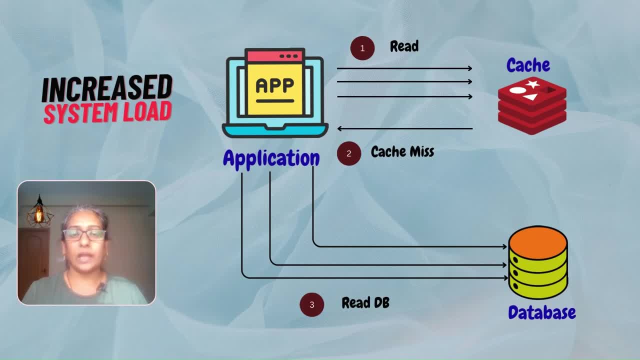 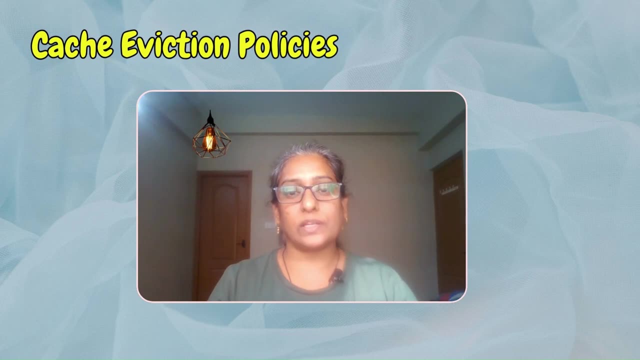 We need to make room for new entries in the cache and reduce cache misses. This process, known as cache eviction, is crucial for optimizing the cache performance. Cache eviction policies determine which items are selected for removal based on a certain criteria. Let's discuss few cache eviction policies. 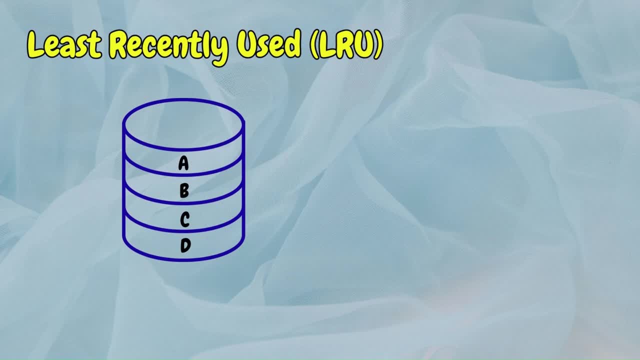 LRU removes the least recently accessed items when space is needed for new entries, For instance in a web browser's cache. using LRU, if the cache is full and a user visits a new web page, the least recently accessed page is removed. 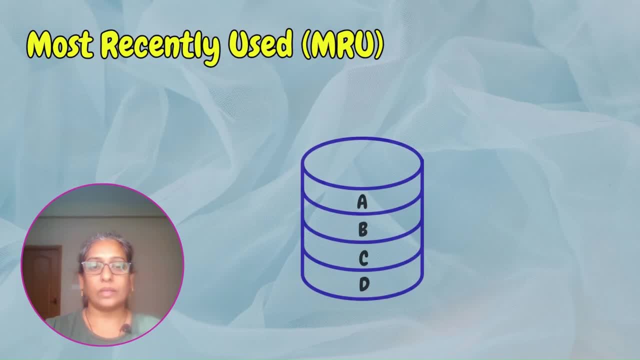 To make room for the new one. MRU evicts the most recently accessed items to free up space when necessary, For instance, in a mobile app cache. when the cache is full and the user tries to access a new feature, the most recently accessed feature is evicted to accommodate the new data. 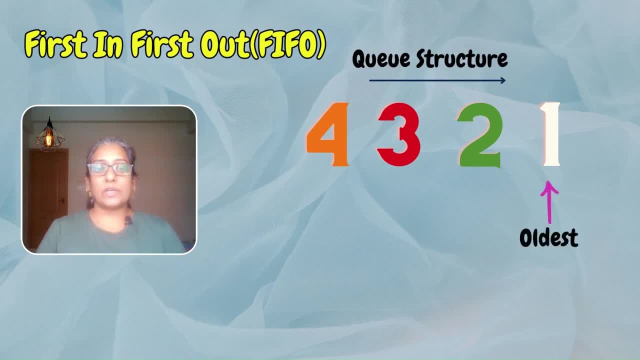 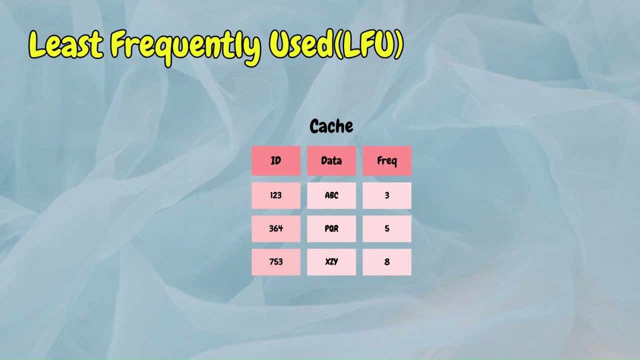 In a first-in-first-out cache, the oldest items are removed first When space is required, For example in a messaging app. when the cache is full and a new message arrives, the oldest message in the cache is evicted. Least frequently used caching removes items that are accessed the least frequently. 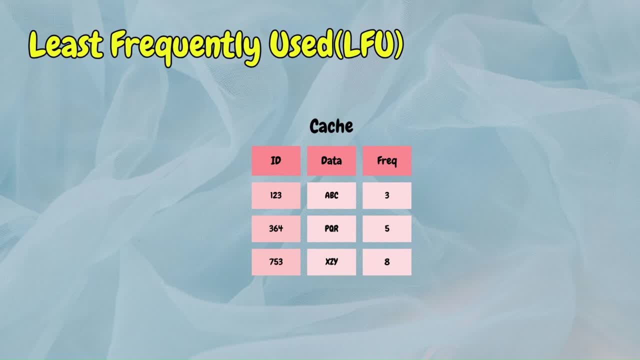 LRU keeps track of access frequency and when space is limited, it removes items with the lowest access count. For example, if the cache is full and the user tries to access a new feature, the most recently accessed feature is evicted. LRU keeps track of access� 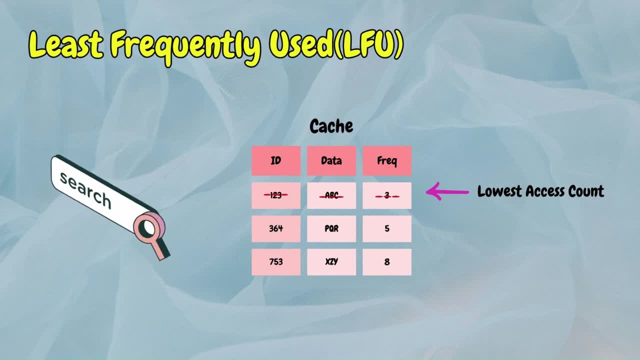 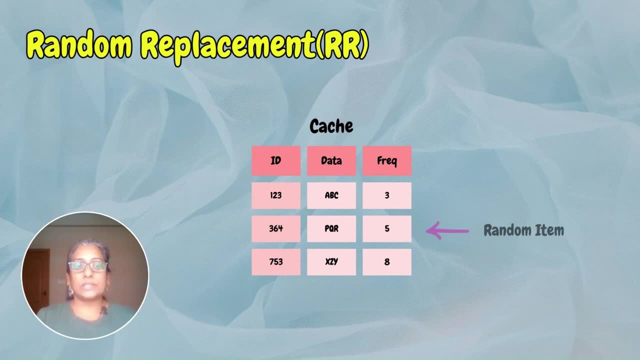 For example, in a search engine cache, � less frequently� search queries may be evicted to make room for popular ones. Random Deplacement Caching selects items for eviction without considering access patterns. For instance, in a game app cache, when new game assets are to be cached, 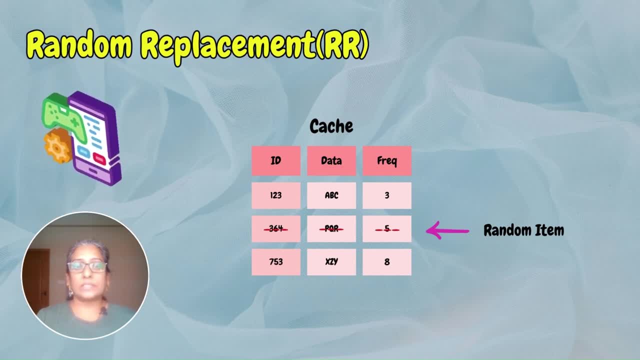 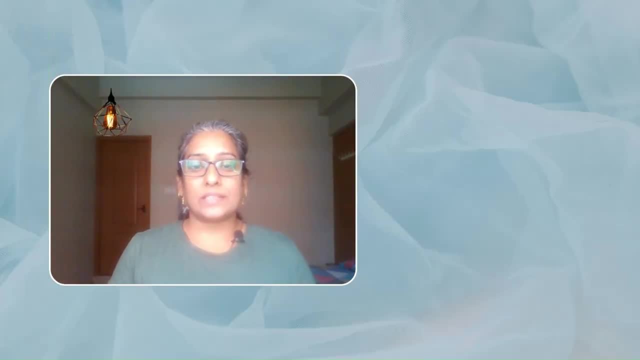 RR randomly selects existing assets to replace. Each cache eviction policy has its advantages. For example, if you want to access a concept by using the search engine. For example, if you want to access a concept by using the search engine. If you want to access a concept by using the search engine. 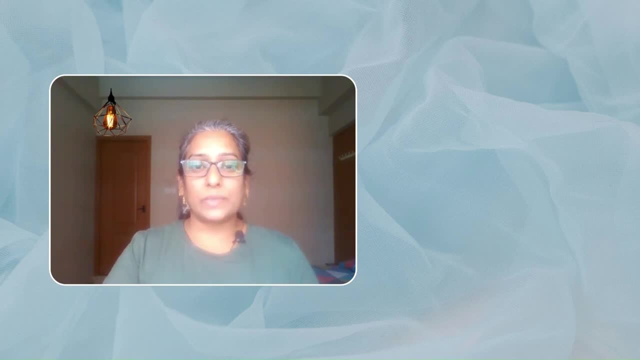 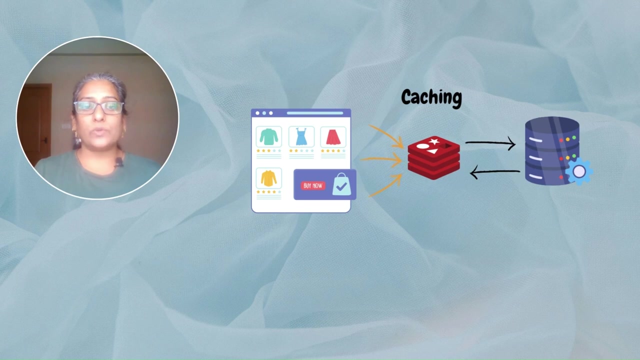 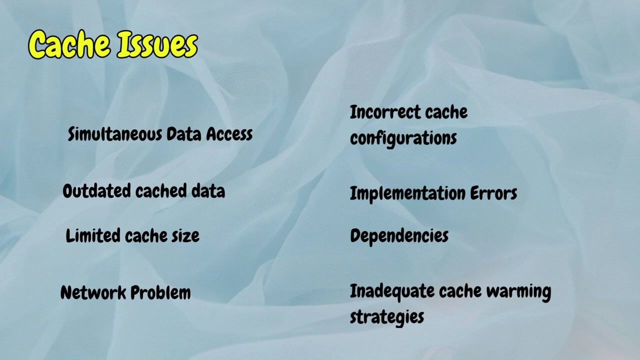 and disadvantages, and the choice depends on factors such as applications, access patterns, memory constraints and performance requirements. The e-commerce platform in our example has now implemented a caching solution leading to noticeable improvement in website performance. However, several cache-related issues have recently emerged. 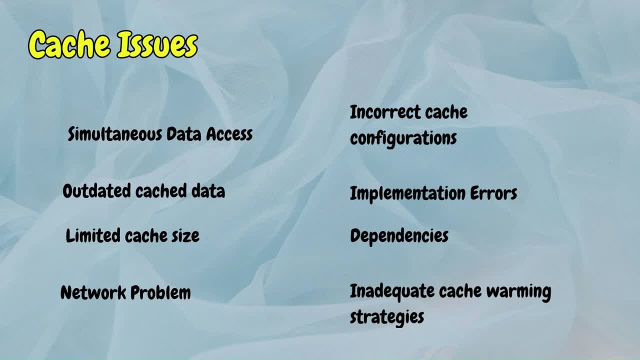 Cache-related problems occur due to issues such as multiple users or processes accessing data simultaneously, outdated cached data, limited cache size, network problems, incorrect cache configurations, implementation errors, dependencies on external systems and inadequate cache-forming strategies. Let's discuss solutions to a few common cache-related problems. 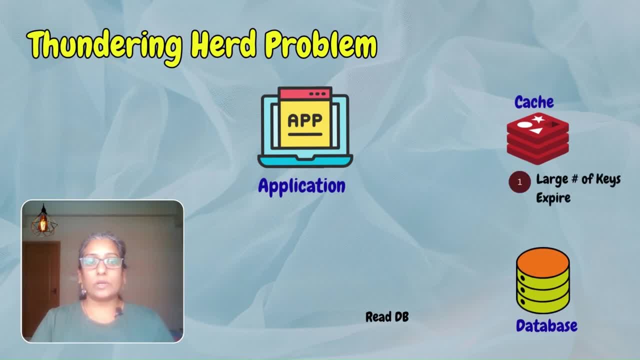 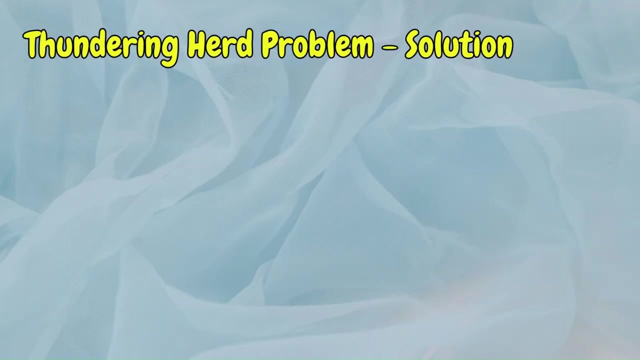 Thunder-herd problem occurs when multiple requests trigger simultaneously cache misses. This could happen when a large number of cached content expires at the same time As the requests now directly hit the database. it overloads the database. There are two ways to mitigate this issue. 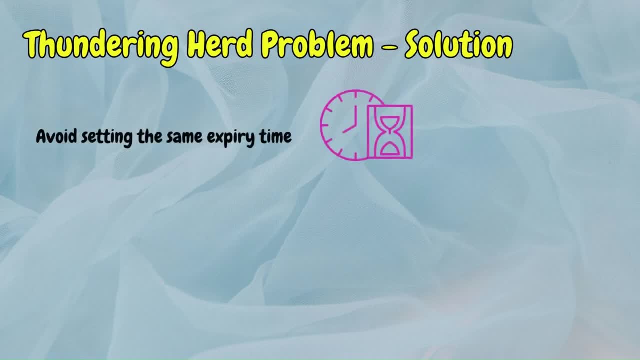 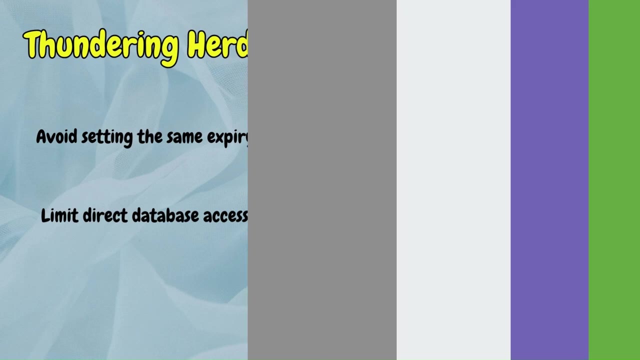 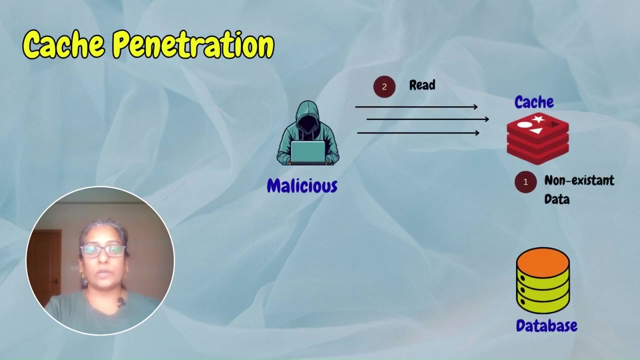 One is to avoid setting the same expiry time for the keys. Another approach is to limit database access to essential business data only, preventing non-essential data from accessing the database until the cache is operational again. Cache penetration happens when malicious users bombard the system with requests for non-existent 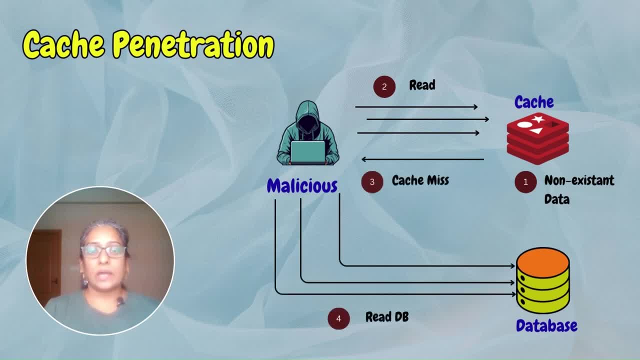 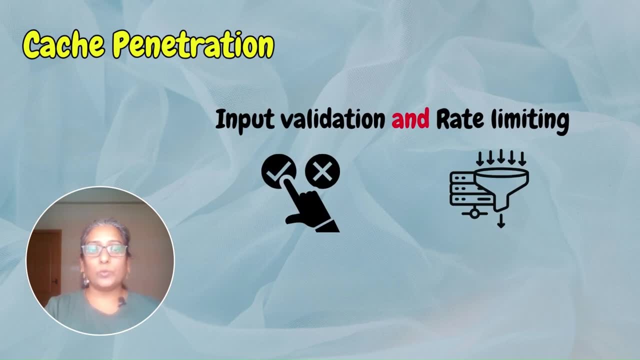 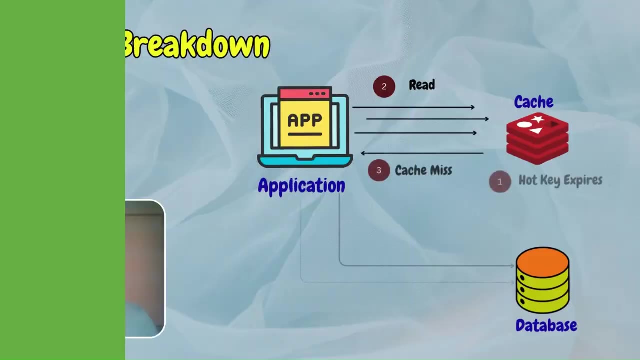 data. This causes cache bypass and causes unnecessary load on the back-end. One solution could be to implement input validation and rate limiting to mitigate the impact of cache penetration attacks on the system. The cache breakdown problem is similar to the thunder-herd problem.